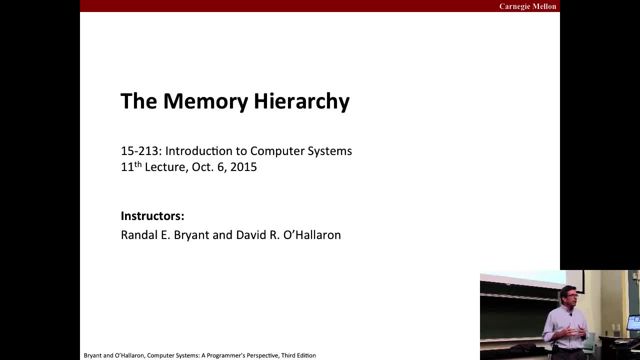 But in actuality, the memory system is a very complex system. It's a very complex hierarchy of devices that provides this abstraction of this large linear array. And so today we're going to look at how memory hierarchies are built and why they're built the way they are. 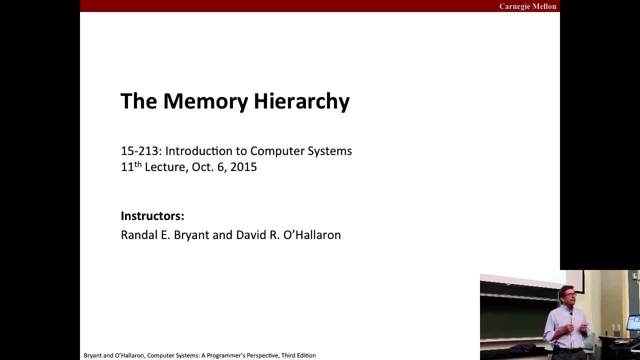 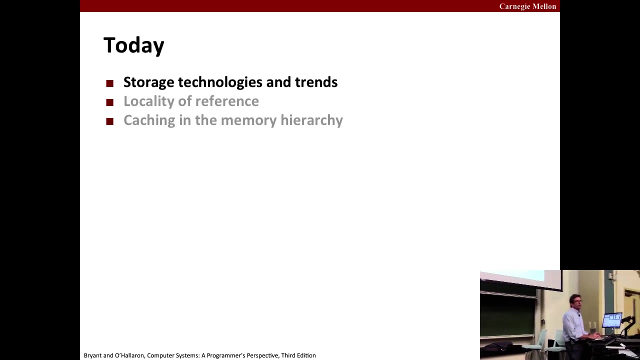 And what we'll see is that this sort of beautiful confluence of the properties of storage devices and the properties of programs come together to create this hierarchy. So we're going to quickly kind of do a high-level tour of storage technologies and trends. We're not going to go into a whole lot of detail. 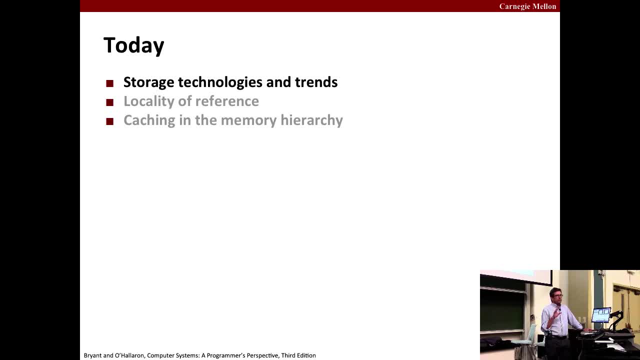 The point in looking at the properties of these technologies is that there are some fundamental properties that determine their performance and their speed, determine limits on their performance and speed, And so I want you to have just some high-level idea of what those, what those properties are, and then we'll. 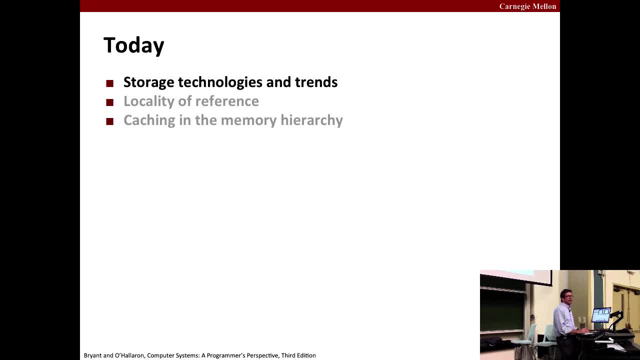 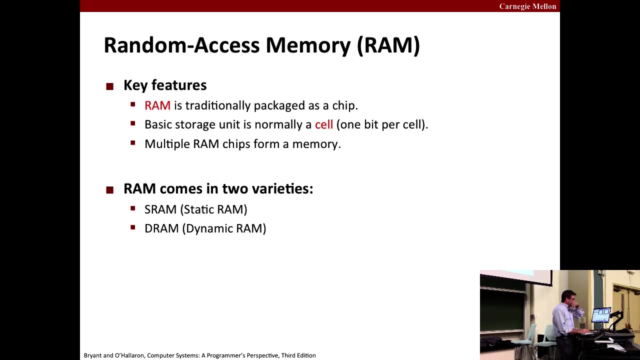 look at a property of programs called locality of reference and we'll see how that locality and the properties of storage devices come together to suggest this design of memory systems as a as a hierarchy. okay, so we'll look at memories first. now the, the workhorse memory, is called a random access memory or RAM. 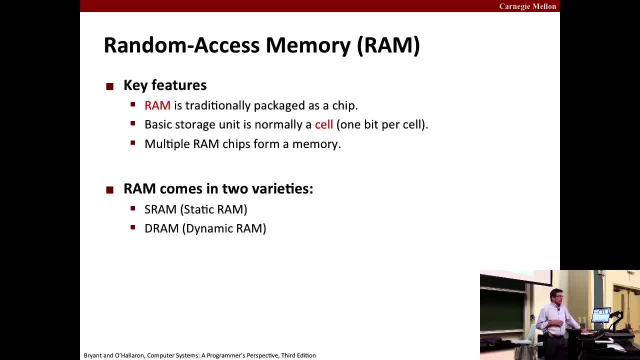 it's, it's traditionally packaged up as a chip, and then you put multiple chips together to form, to form your main memory, and there's a basic storage unit called a cell, which, where each cell stores one bit. okay, now there's there's a RAM, comes in two varieties: there's a SRAM and DRAM, and they're distinguished. 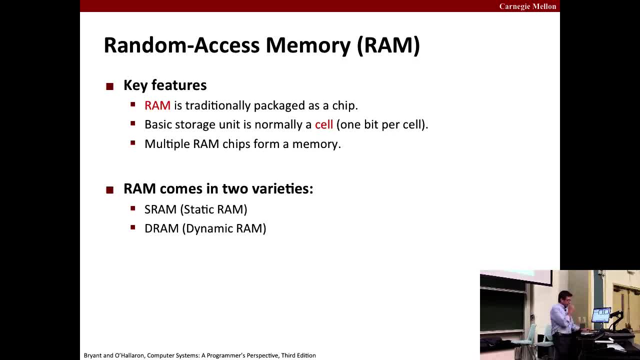 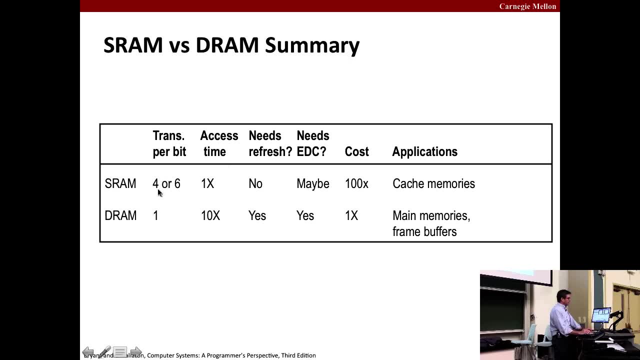 by the the way that those cells are implemented. so in an SRAM requires it's. it's more complex than a, than DRAM. it requires like four to six transistors per bit, whereas DRAM only requires one transistor. okay, so you'll see that SRAMs are going to be more expensive, lots more expensive, because 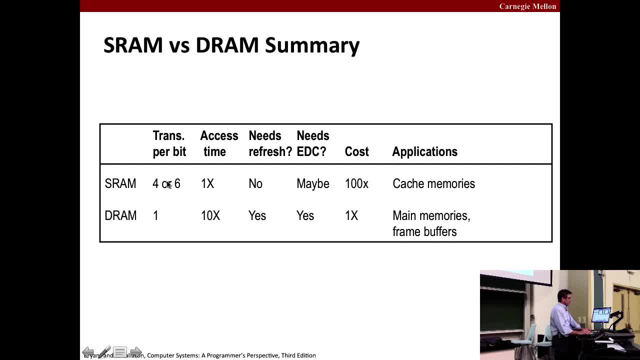 they. they're more complex- each cell is more complex- but they're also much faster, like ten order of magnitude faster than DRAMs and they have a. they're so much relatively less expensive than each ACE cell. you have right, that's quite common AR. I count 55 vagabond. I have a Canon of Yay Public. 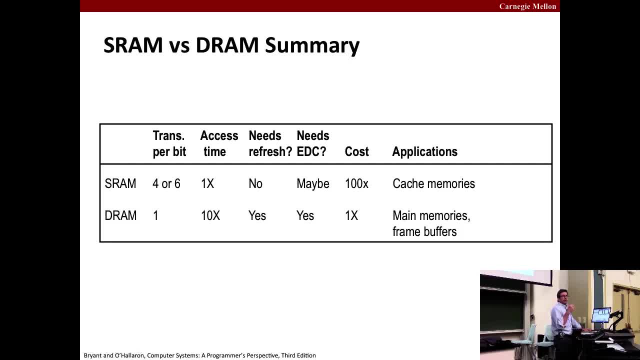 Data center. so there's typically 600 oruck and of them it's essentially just multiple 선 here. all right, so it's a award. I mean again, there's not that much of a difference between the PRAM degrees. I don't think they adjust. there's some benefits that the, the 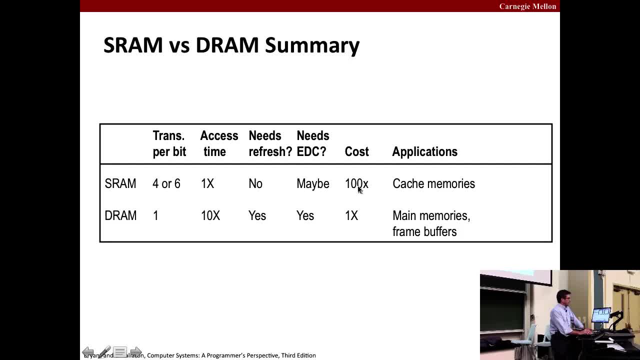 right, this is only 50%. so if you raw promote what we're not, they capture a lot of data, right so. but the PC Fach efforts are not color for use, and so on and so on. The SRAMs are costlier, smaller and faster than DRAMs. 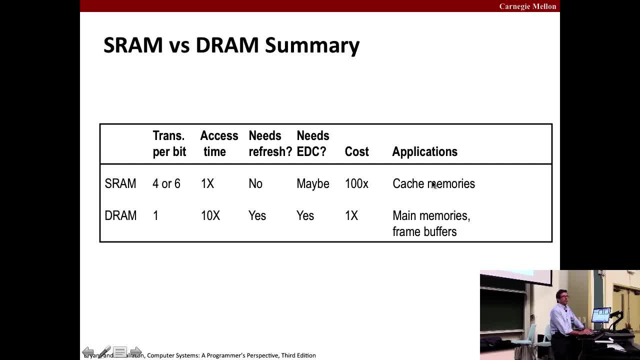 We find SRAMs being used in these small fast memories on chip called cache memories, And we're going to learn all about those on Thursday. And then DRAM is the workhorse used in main memories and the frame buffers associated with graphics cards. 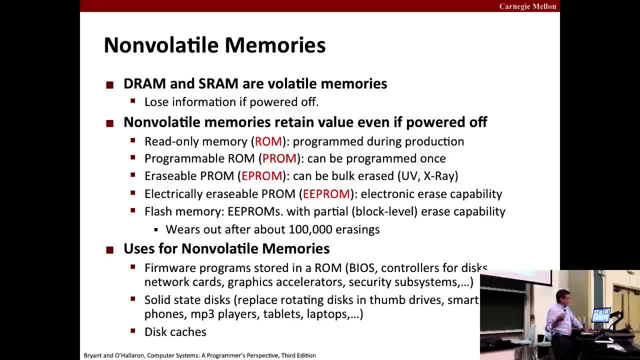 Now, DRAM and SRAM are volatile in the sense that if they're powered off they lose all the information. So this is why when you turn your computer off, you lose everything in your memory, And when you turn it back on you have to sort of reload everything from your disk. 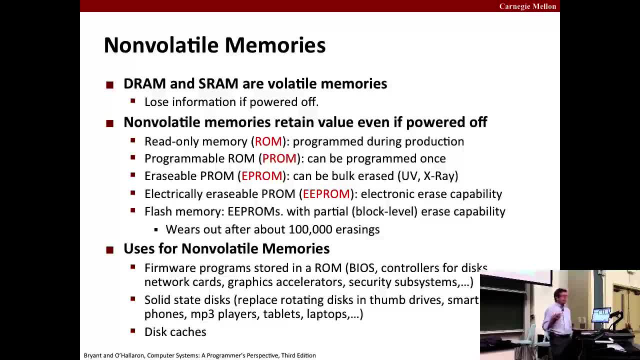 There's another kind of memory called a non-volatile memory, which retains It's information when it's powered off, And there's a whole bunch of these things, so-called read-only memories. So the generic name for these non-volatile memories is read-only memories or ROMs. 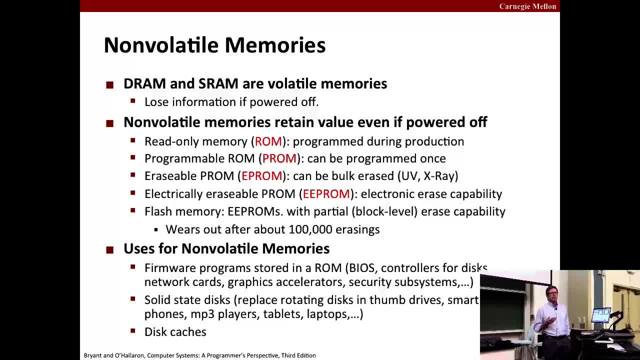 And there's a whole bunch of different kinds, Sort of going back in time. the original read-only memories were ROMs and they can only be programmed once, when the chip was produced, And then over time, gradually, over a period of like 20 or 30 years. 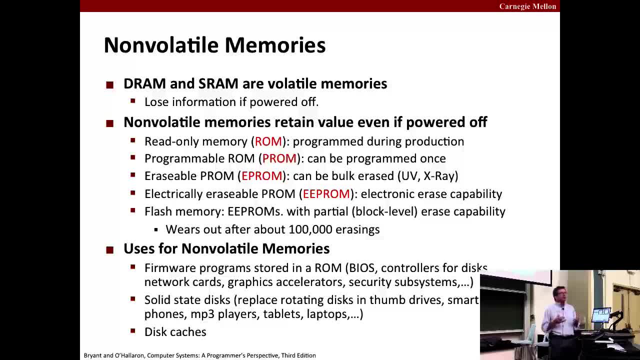 there were improvements in the way that ROMs could be programmed and in how they were erased so they could be reprogrammed. What we have today, the modern form of read-only memories, is called flash memory, which provides the capability of erasing. 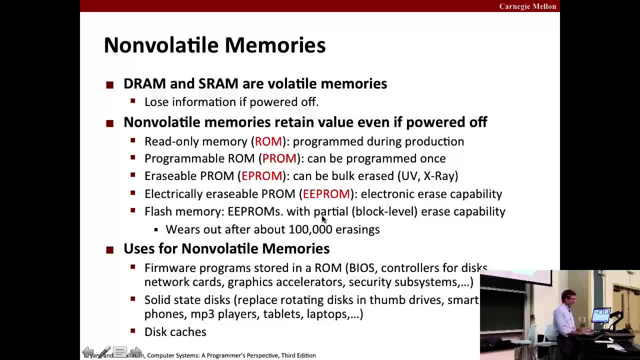 You can erase just chunks of the flash memory, called blocks, And then the downside is that these things wear out after about 100,000 years, So it's a very, very long process. You can erase and reprogram 100,000 erasers, okay. 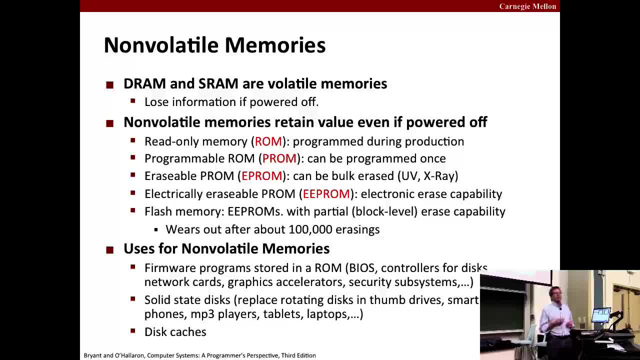 So you can erase and reprogram 100,000 times and then you're bricked. Now these non-volatile memories show up in so-called firmware, which is software that's programmed into a ROM, And you see those in the BIOS of computers. 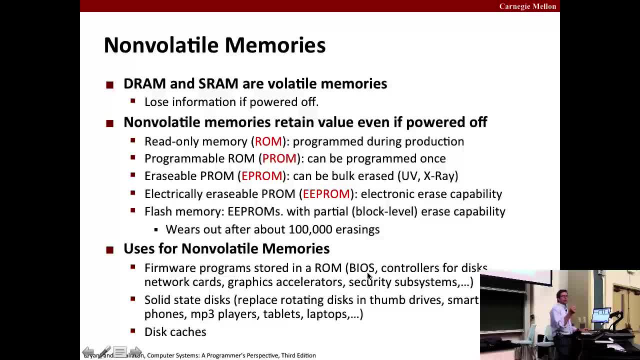 So when you power on your computer, the very first instructions that execute are stored in the BIOS. So when you power on your computer, the very first instructions that execute are stored in the BIOS. So when you power on your computer, the very first instructions that execute are stored in the BIOS. 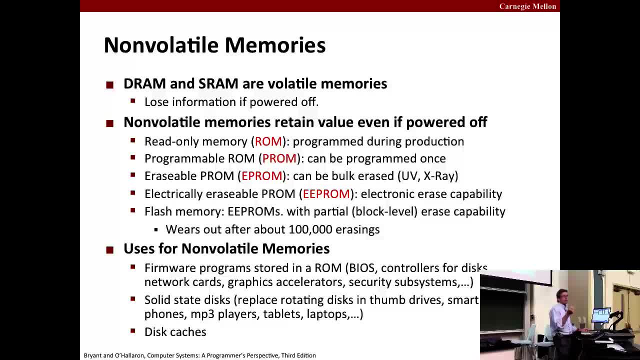 So when you power on your computer, the very first instructions that execute are stored in a ROM, right? If you're wondering, like, where do those things come from? So they're stored in a ROM and then there's a boot process. 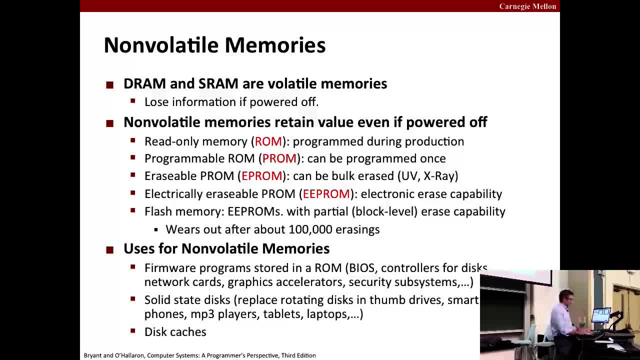 where gradually, more and more information is and instructions are loaded into memory. You know, IO devices have little computers in them, called controllers. These controllers consist of instructions and data that are stored in ROMs And you see them all over the place in these sites. 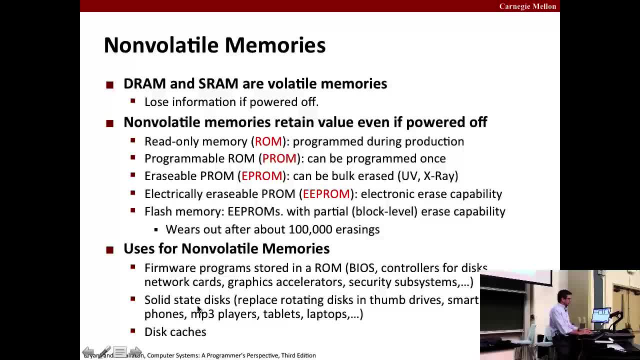 So they're stored in a ROM And you see them all over the place in these sites: Solid-state disks that to the system look like a rotating disk, but they're built of flash memories. And these are. you see these in thumb drives, smartphones, tablets and laptops. 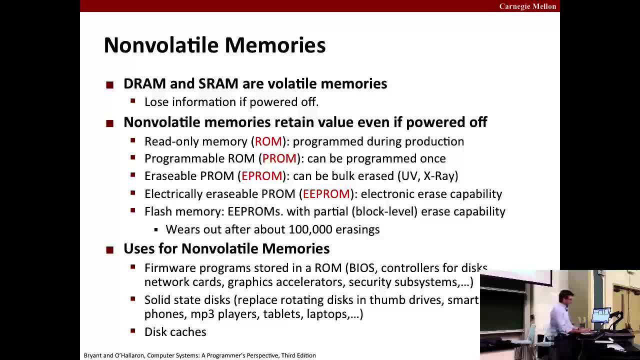 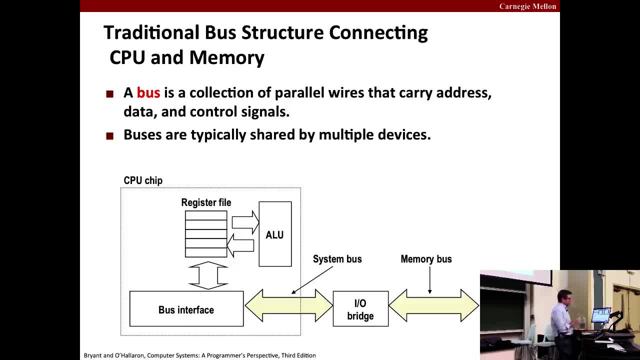 and they're even starting to show up in servers now. So the memories are connected to the CPU. So the memories are connected to the CPU. So the memories are connected to the CPU Using wires that are collectively called buses. okay, So data flows across the wires back and forth from the. we have the CPU chip. 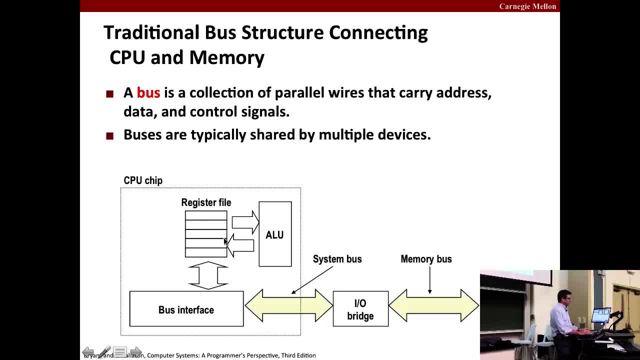 and it consists of a register file- These are the general purpose registers, RAX, RDI and so on- And there's an arithmetic logic unit that reads and writes data from the register files and then manipulates that data in some way by doing this. 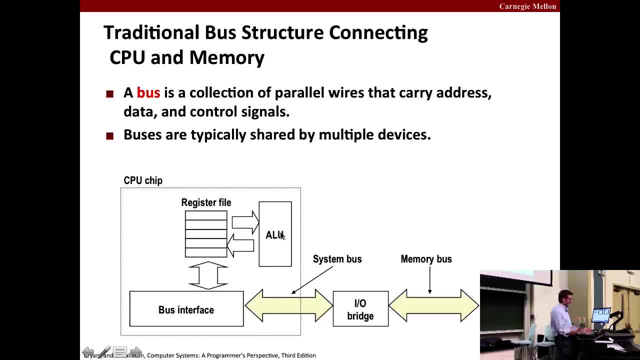 And then manipulates that data in some way. by doing this And then manipulates that data in some way. by doing this, You're doing some kind of arithmetic operation or some logical operation And if instructions need to access memory, so if you're doing a move instruction that reads or writes to memory. 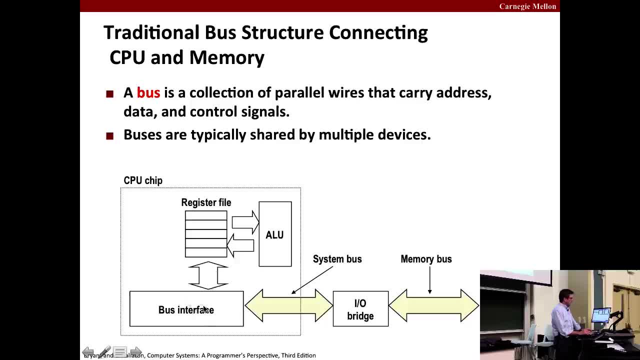 then that's handled by a bus interface which is connected to what we'll call a system bus, And then that's connected to an IO bridge, And this, This is another collection of chips. Intel calls this what I'm calling the IO bridge, they call the chipset. 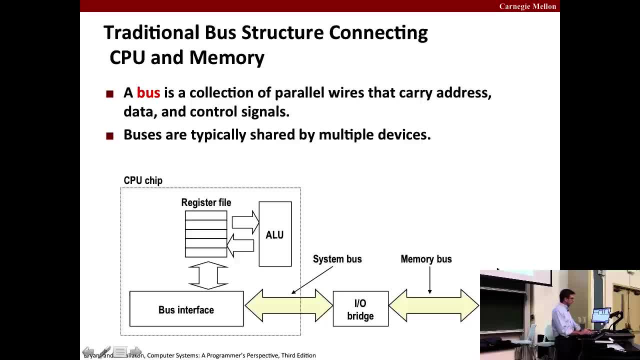 Okay, but it's a collection of chips separate from the CPU chip, And then the IO bridge is connected to another bus called the memory bus, which connects the main memory. Okay, now, this is kind of an abstraction. I don't want you to take this too literally, but it gives you the idea. 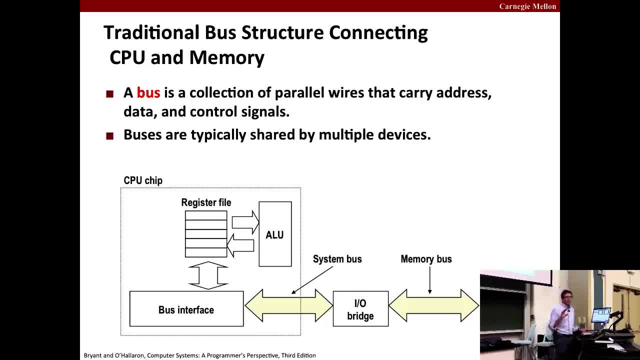 of how information flows in the system. Okay, modern, Modern systems use proprietary bus designs and they're very, very arcane and increasingly complex. So we're just going to use a fairly simple abstraction for these bus architectures. Now suppose you do a load operation. 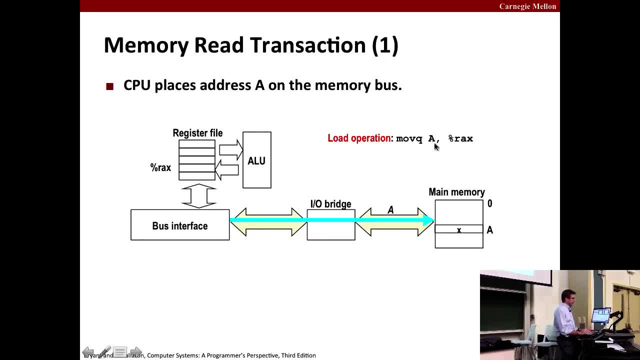 like move queue the eight bytes at address A into RAX. Okay, so we call that a load because we're loading from the point of view of the CPU. we're loading data into the CPU, Or we're loading data from memory into the CPU. 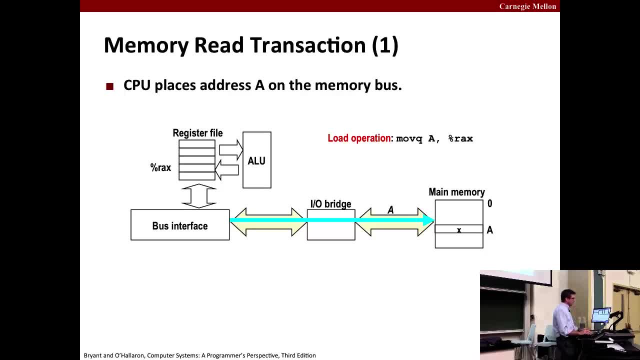 So when the CPU executes a move instruction like this, it first places the address of A on the memory bus and then the main memory senses that address and it reads the contents, the eight bytes at address A, So it retrieves the word. 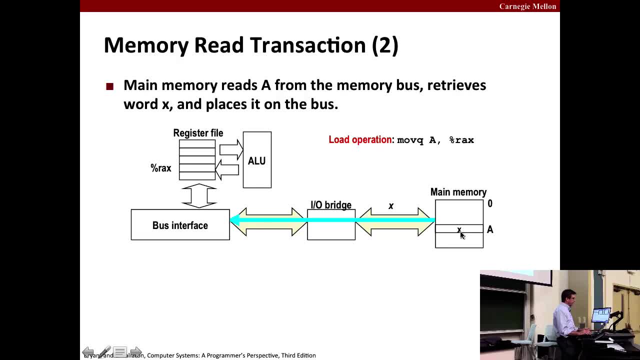 The eight byte word from address A and places it back on the bus. Those bits travel through the IO bridge to the bus interface and then the CPU reads the word X from the data, word X from the bus and then copies it into register RAX. okay, 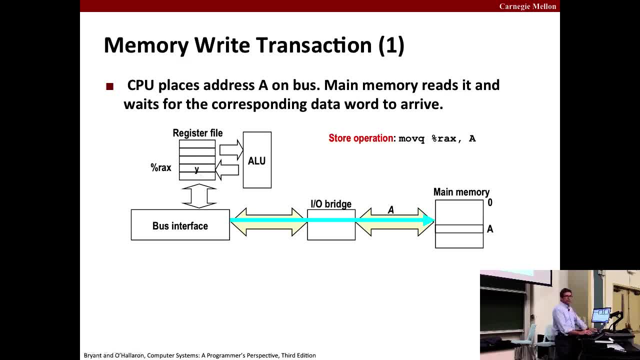 So it's now. writing is similar Again. so here we're doing a move instruction. Move queue from RAX. Move queue from RAX into address A in main memory. Okay, so the CPU starts as before by placing the address A on the bus. 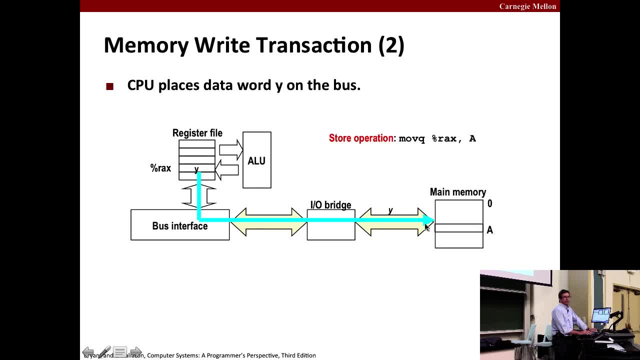 Main memory reads that address and then it waits for the data to arrive on the bus. So the CPU then places the contents of RAX on the bus and those contents travel across to main memory, which then reads the, reads that word from the bus and stores it at address A. 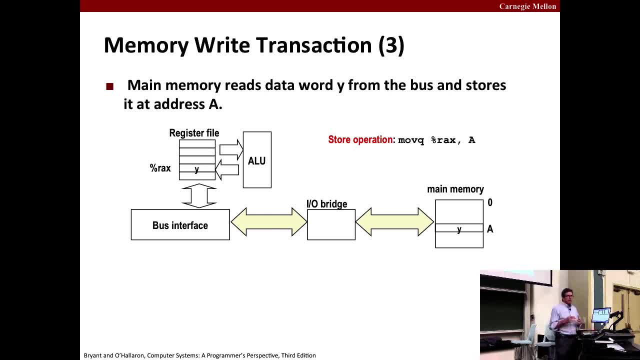 Okay, So the And the. the point about this is that operations that occur- you know, reads and writes of registers, because the register file is very close to the ALU- these happen in in on the order of a few cycles, okay. 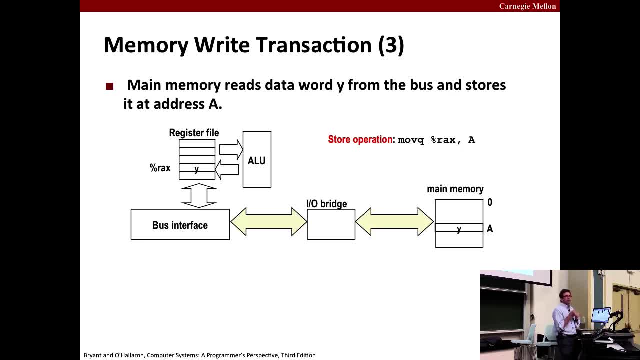 Register. the register is very close to the, to the ALU, So those operations or very happen very quickly, Whereas memory is actually OK, Fogs, Uthl, away, relatively speaking, from the CPU, and there's a lot going on. and when you 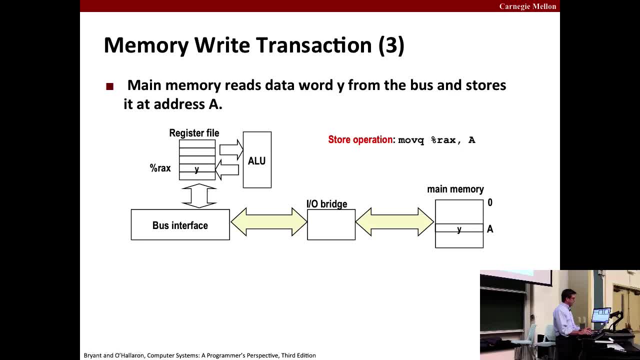 if you have to read or write memory there's, you have to do multiple operations on the bus. data has to travel, propagate across that bus. all this stuff takes time. so memory operations- reads and writes- are typically, you know, maybe 50 nanoseconds, 100 nanoseconds, whereas operations that occur between registers. 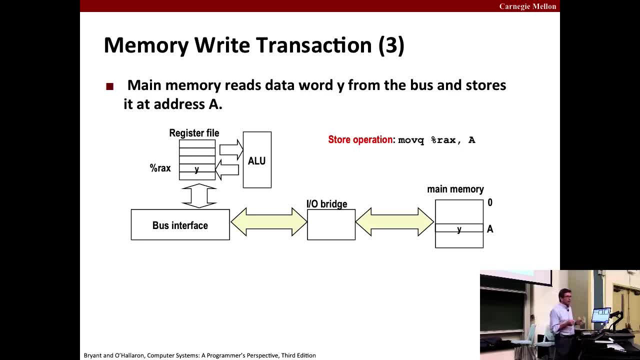 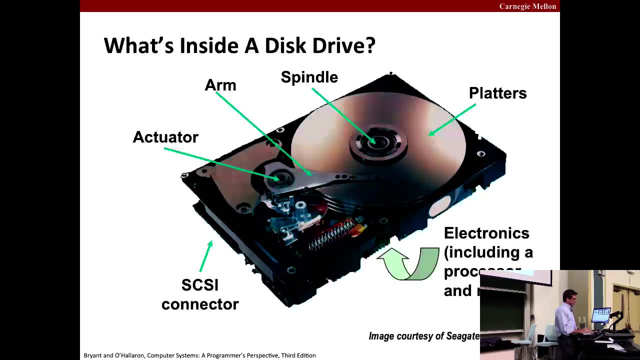 or sub nanosecond. okay, on the order. so you're talking about one to two orders of magnitude difference. if you have to go off chip to retrieve something from memory, okay. so that's the first sort of big takeaway item about memory systems. now another popular storage technology is rotating disks, and I don't know if 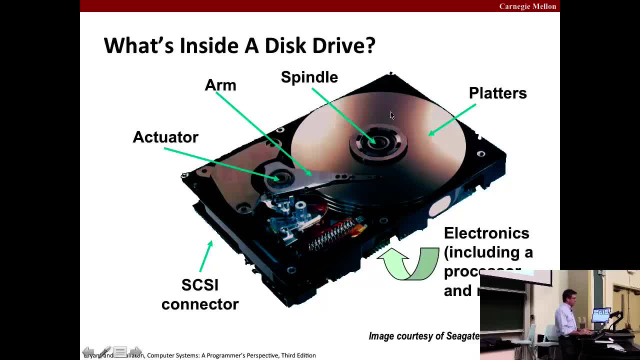 you've ever torn one apart. they're kind of interesting that there's a series of platters, platters, platters. each platter is coated with a magnetic material and then, and then bits, ones and zeros are encoded in that, in that magnetic material, and then there's this: 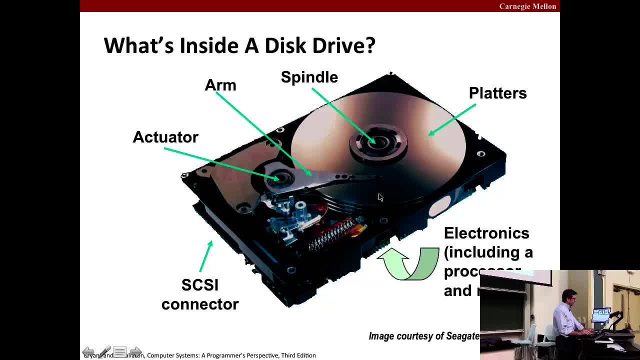 arm. that can it's. it's hinged right here and then it can. it can it floats over the platter. so it floats on a thin layer of air over the platter and there's a read right-hat at the very end that can sense the changes in the magnetic field. 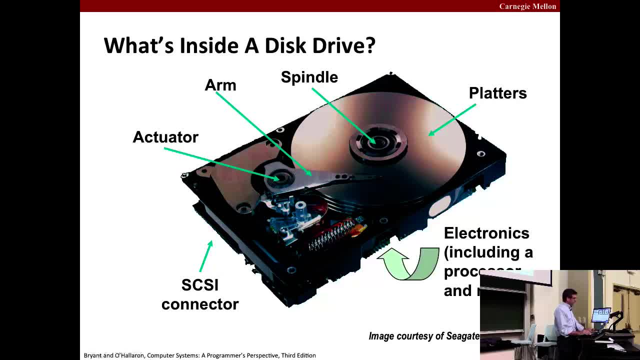 that encode the magnetic field and then it floats over the platter. so it floats over the bits. okay, so these platters are spinning around like, like counterclockwise, like this, and this, this arm can go back and forth. so there's a lot of mechanical gear, so this is all mechanical. so the mechanical nature of a 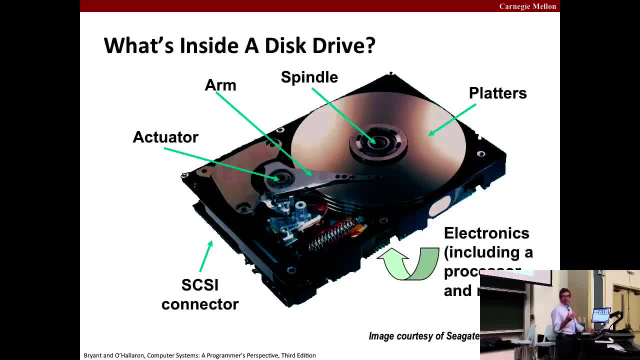 rotating disk means it's going to be slower, right then. then D Rams and NS Rams, and there's also electronics, like it's like a little computer in firmware that that actually controls the, the operation of this drive, like controls how this, this arm, goes back and forth. 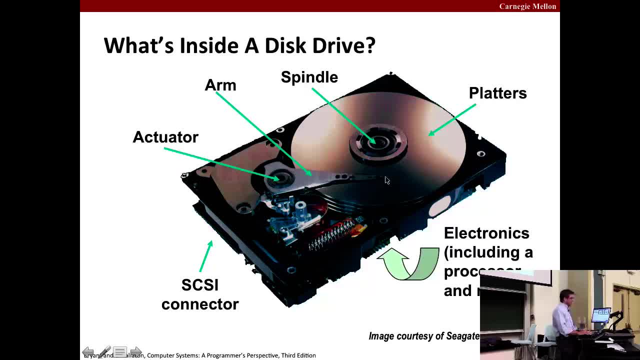 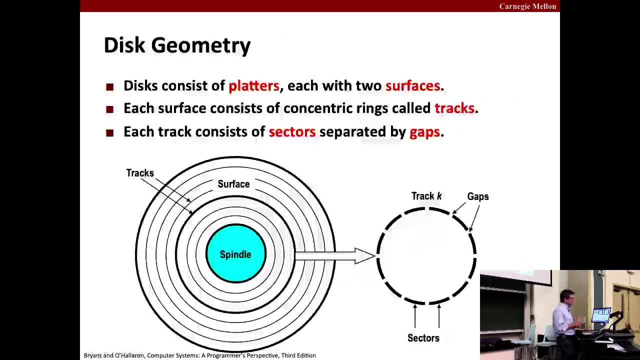 and and and controls how the data is read off of the, the read write head. so just in a little more detail we can think of these. discs consists of platters. each platter has two surfaces, the top and a bottom, and then the. each surface consists of these trans, these concentric rings called tracks, and then 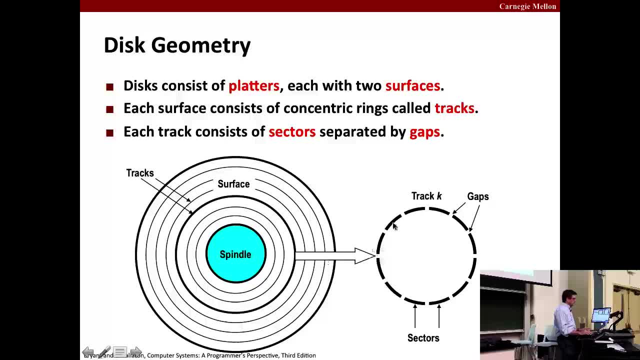 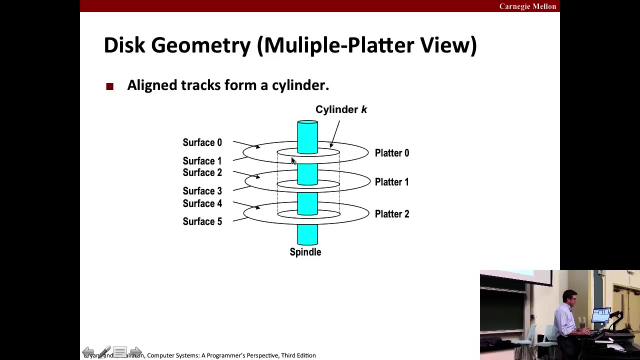 each track sound track consists of sectors which contain the data, so typically 512 bits or, I'm sorry, bytes, and then these tracks are separated by gaps. these gaps, like right here, that don't contain data. Now, platters are aligned on top of each other on this spindle, and so 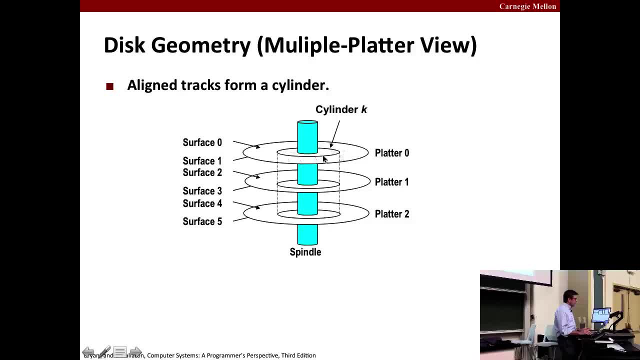 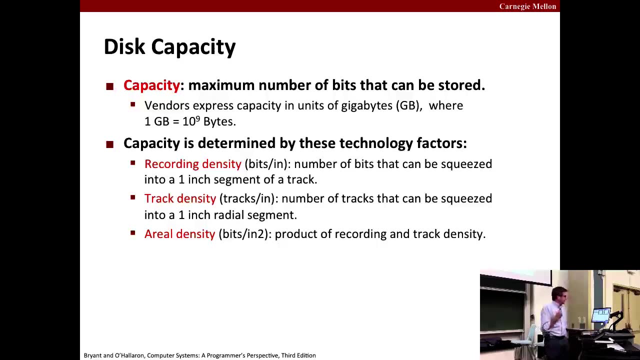 tracks that are aligned on the different surfaces, such as this track here. the collection of those tracks form what we call a cylinder because it has this cylindrical shape. Now, the capacity of disks is the number of bits that can be stored And vendors kind of all disk vendors use. they quote the capacity in gigabytes, but 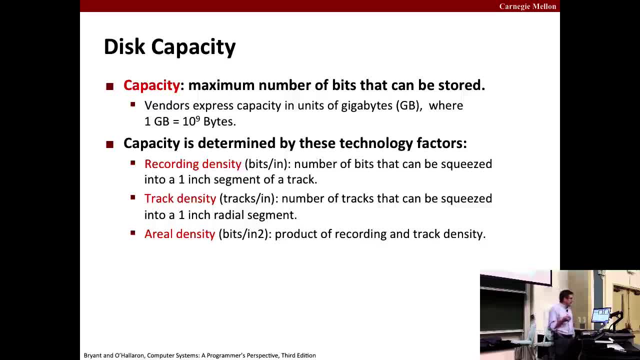 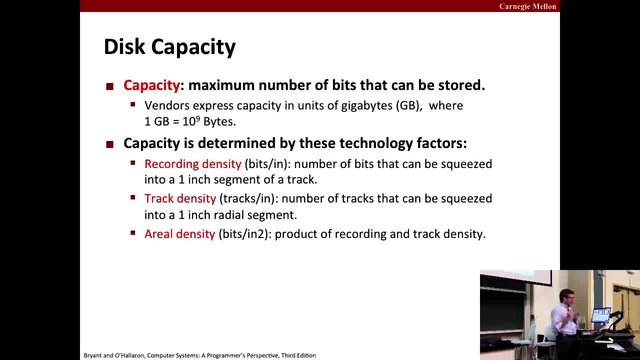 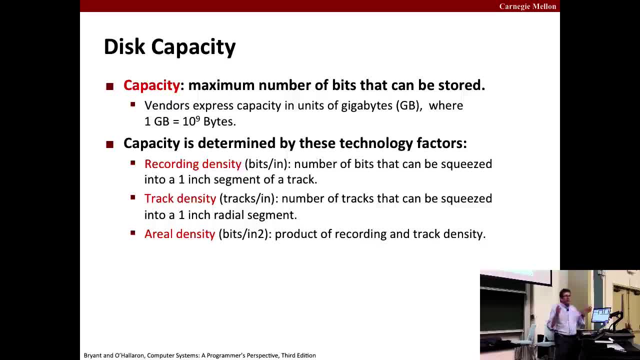 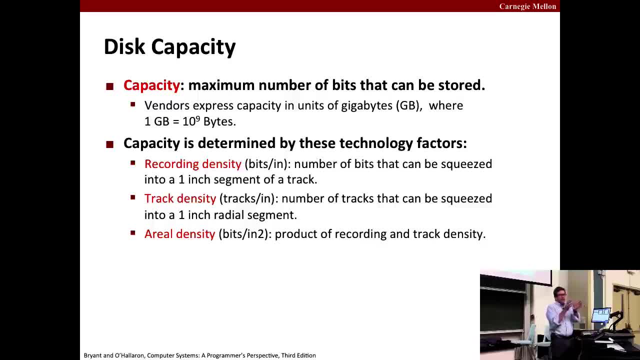 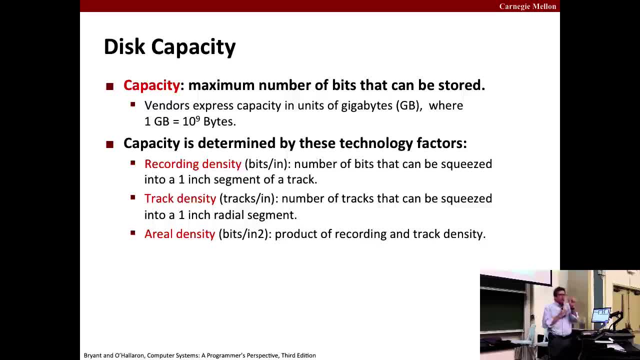 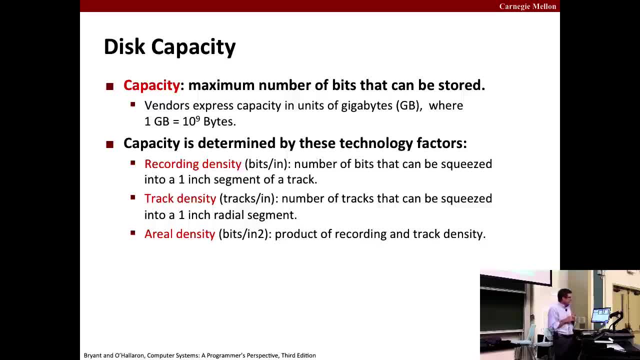 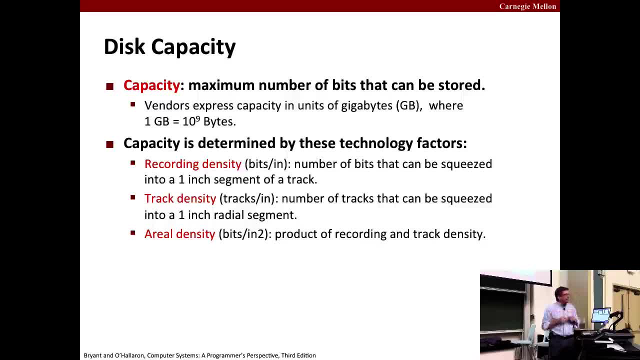 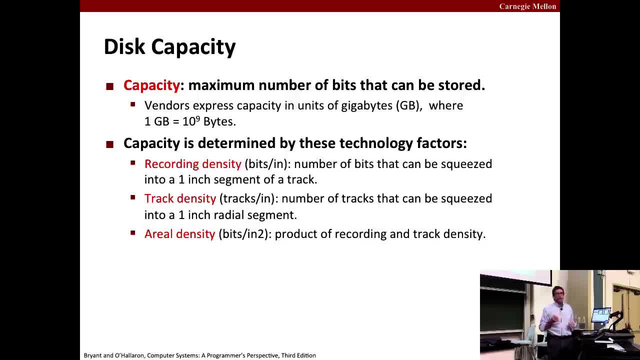 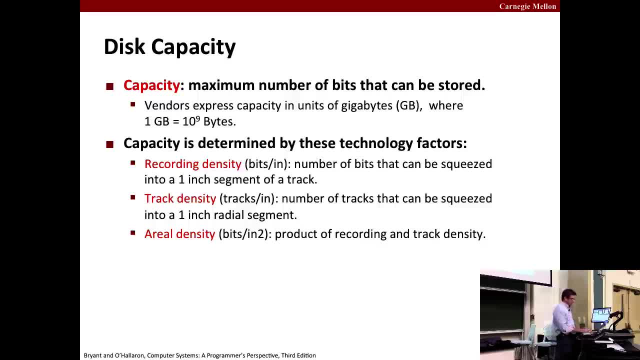 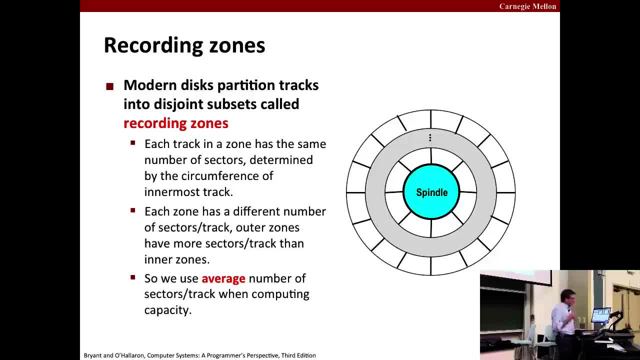 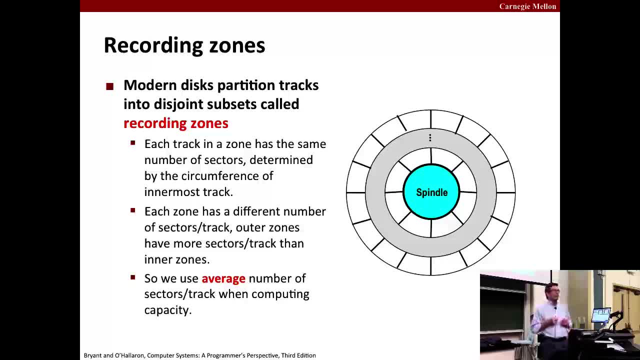 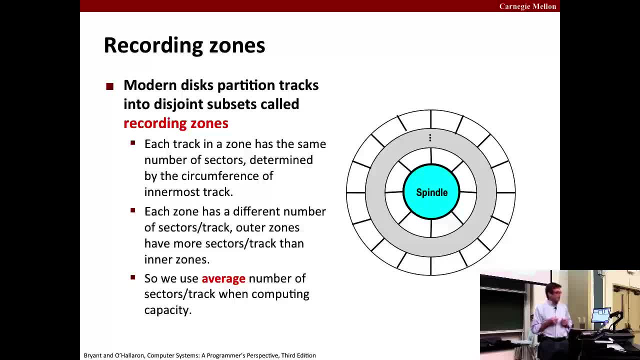 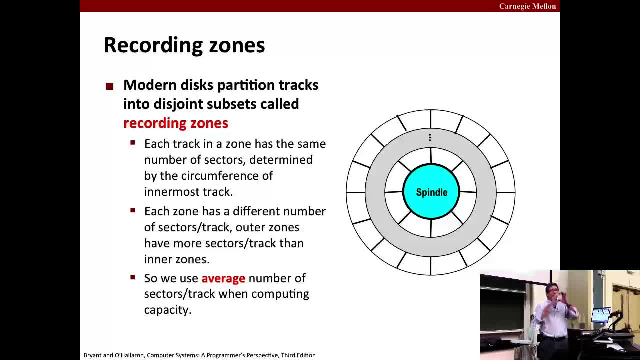 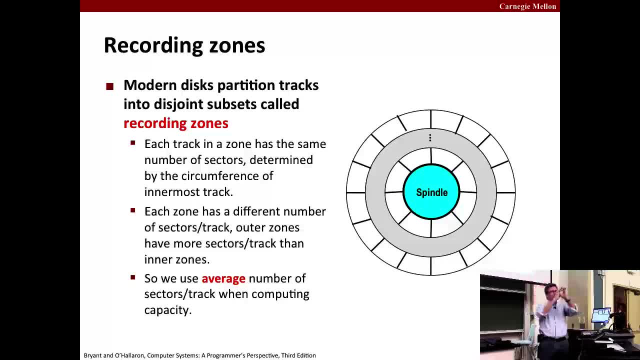 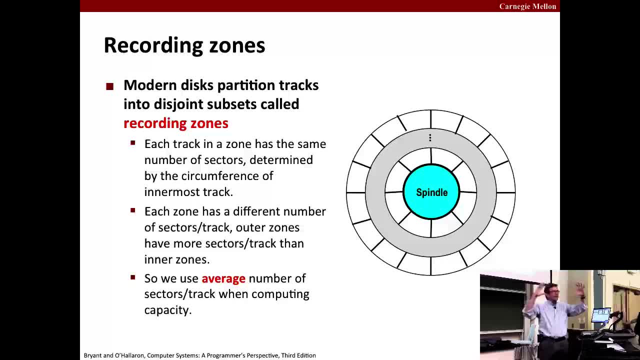 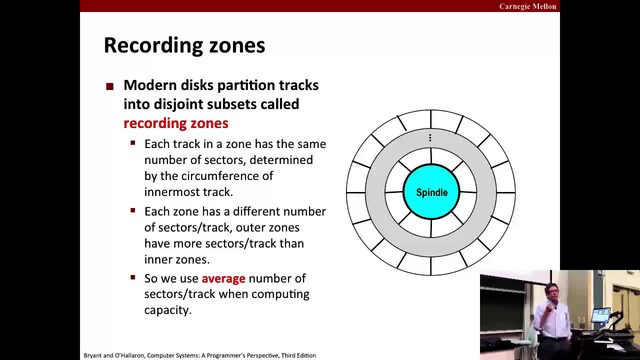 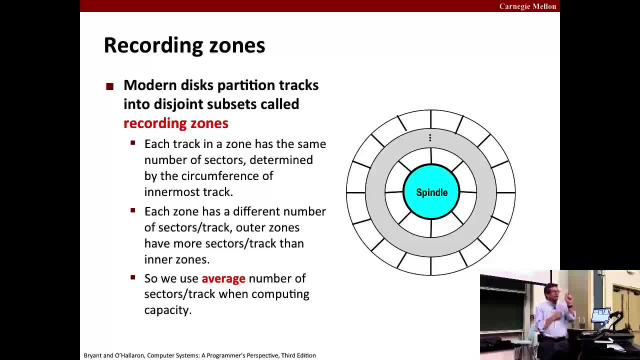 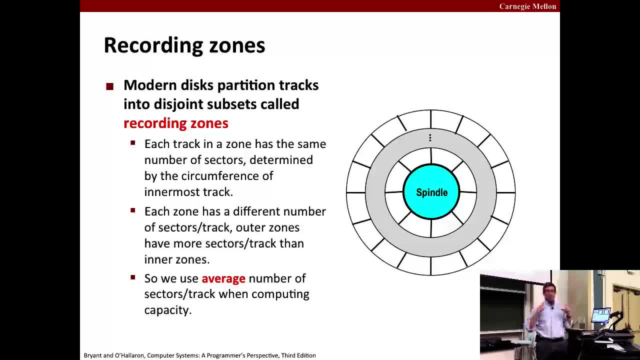 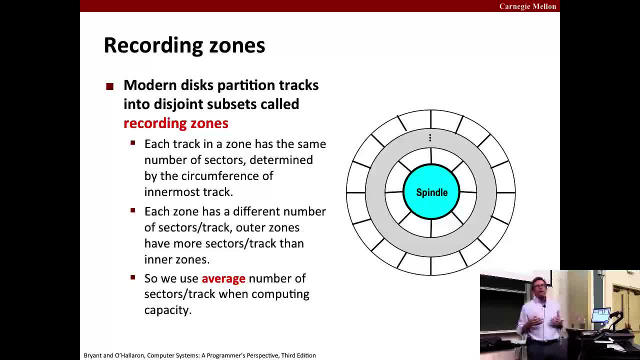 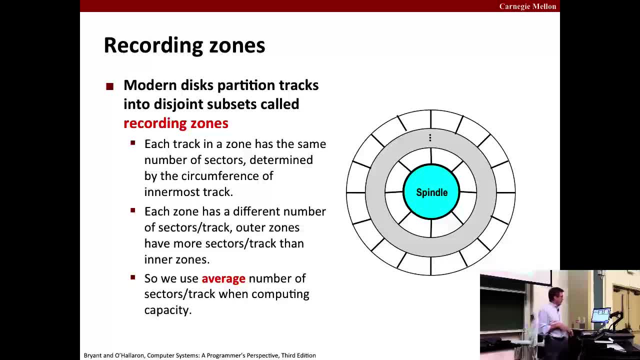 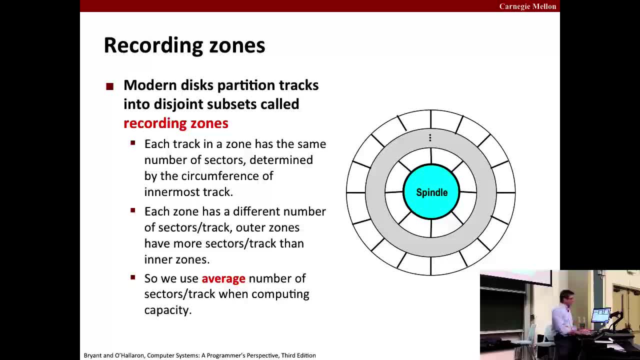 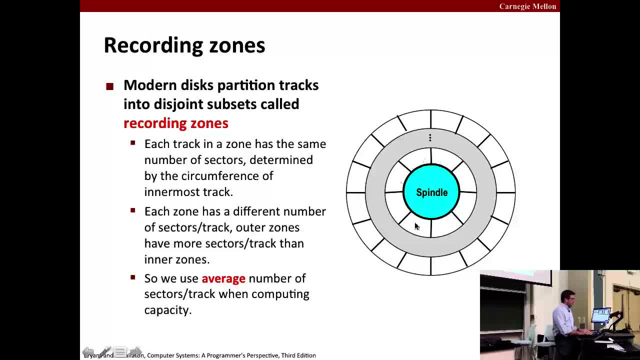 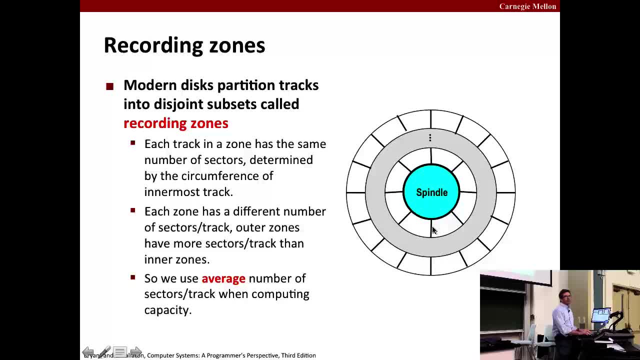 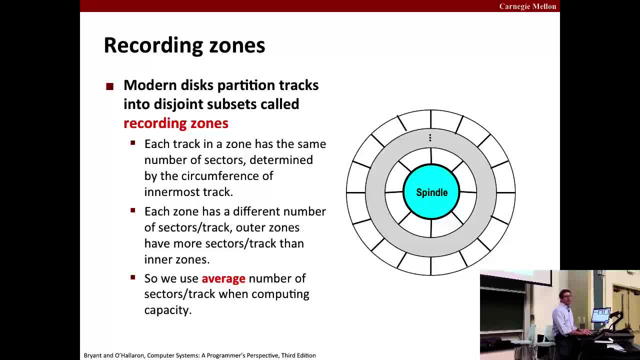 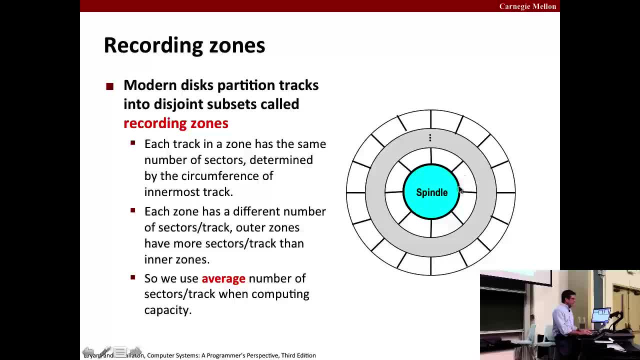 their capacity in gigabytes, but it allows by quoting their capacity in gigabytes, but it allows by quoting their capacity in gigabytes, but it allows by quoting their capacity in milligrams. and newини getting too large and so, because we don't really have the, the number of 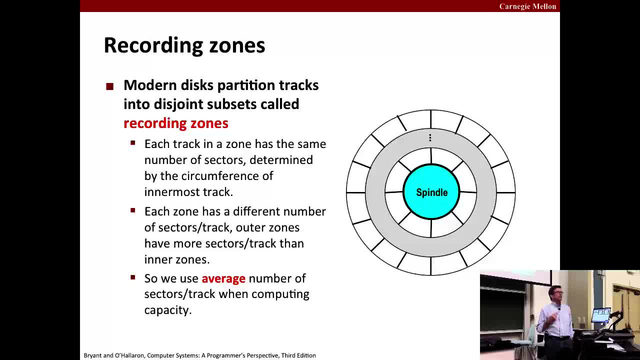 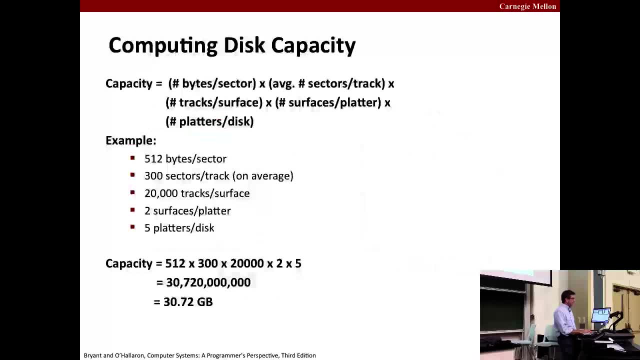 sectors per track isn't constant. we'll use an average: the average sectors per track across all recording zones, when we do serve our capacity estimates. okay, so, as you can imagine, the the formula for computing the disk capacity is fairly straightforward: it's the number of bytes per sector times the average number of 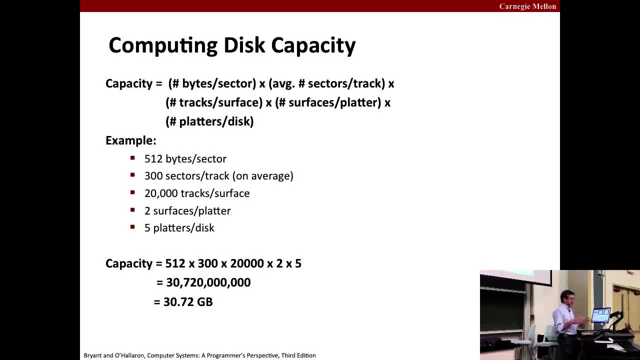 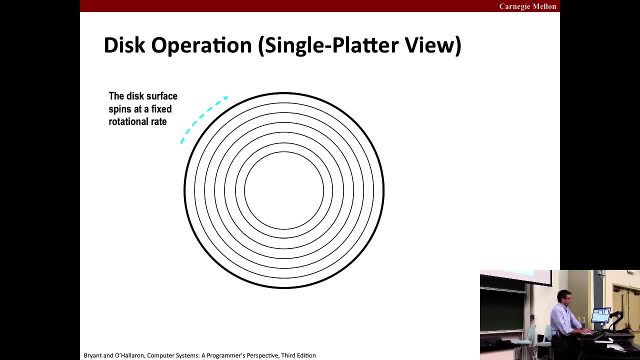 sectors per track. times the average number of tracks per surface. times the number of surfaces per platter. times the number of platters per disk. okay, now let's look at how disks work. so these, these surfaces are spinning at a fixed rotational rate. now a typical rate maybe. 7200 rpms is a fairly common rotational. 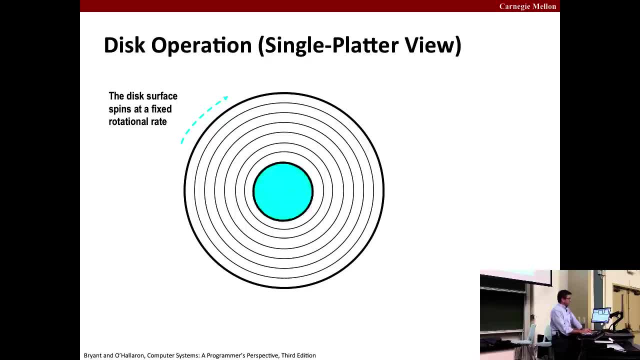 rate. so the disk is spinning around. you can see this pretty proud of that. so it's spinning around the counterclockwise and then the the. the arm moves radially. here we go. the arm moves radially and it can go over any of the tracks. okay, all right. 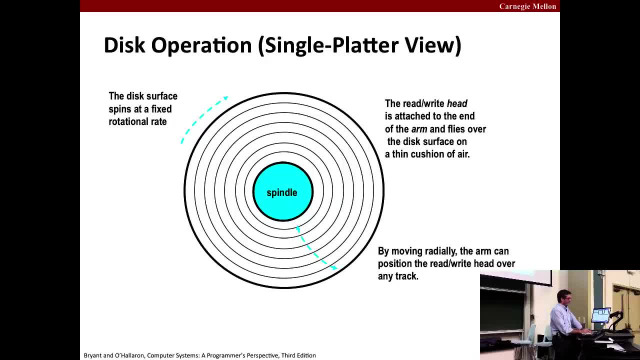 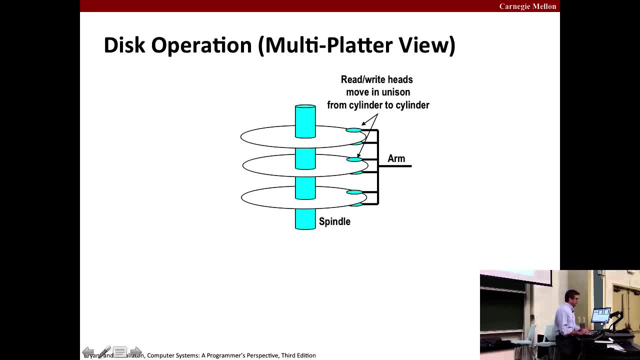 that's enough. okay now, when you have multiple plans. So the platters, each one of these, each one of these, there's actually multiple arms and there's a reed right head on each surface. so if the platters has two, if each side of the platter is coated with this magnetic material, then you have a reed right head on each side and then these are all connected and they kind of move together. 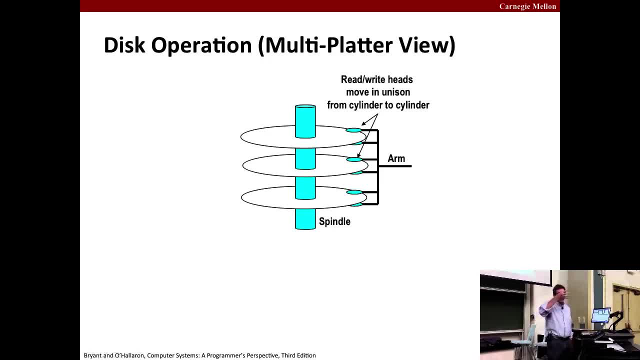 Now, originally these reed right heads would be. they were rigid right because the densities track densities weren't that high, so they could just sort of like, and even though the tracks didn't align perfectly, they could just sort of they could still cover. the reed right heads could still cover the tracks with these fixed arms. 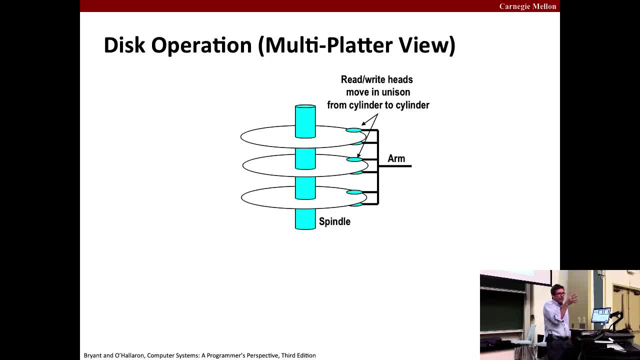 But nowadays the densities are so high that they actually the controller can actually move the reed right heads a little bit so that it matches up with the all of the tracks on all of the surfaces, right? Okay, so let's look at how this works, how we read data. 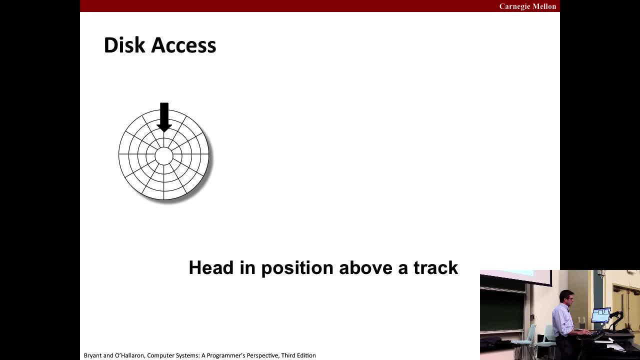 So we have our, this is our, this is our arm, and the tip of the arrow is the reed right head, and it's positioned. and the platter is rotating counterclockwise And it's positioned, just ready to read the blue sector. 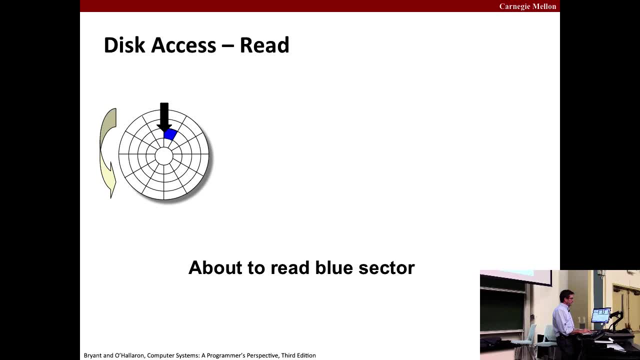 So it, as the blue sector spins underneath the reed right head, it senses those bits and sends them up to the controller, which passes them back up to the, the CPU. And now the CPU has requested that the the disc, it's requested the red data from the red sector. 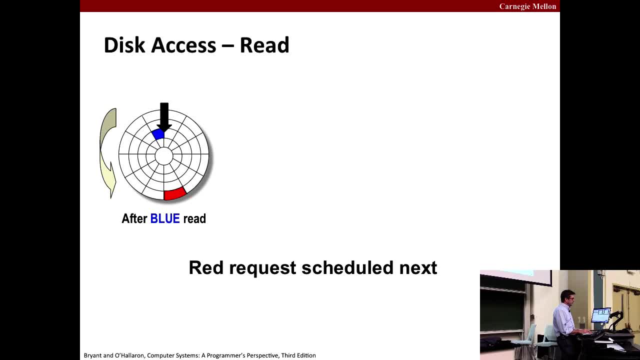 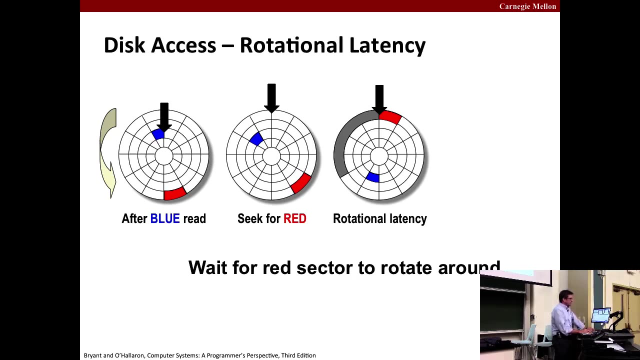 So we have to take the. the controller takes that reed right head, moves it back to red's trap- Okay- and then waits for it to spin around and to the to the read right head, and then it reads that. that read that red sector: okay, so when we first. so there's really 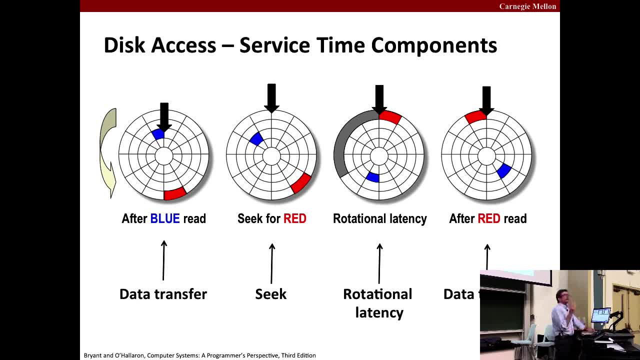 three components going on here that determine how long it takes to read one of these sectors, the. when we move the head, that's called a seek. when we waited for the red track to to sort of rotate around, that's called the rotational latency. so however long it takes, on average it'll be half of the half of the. 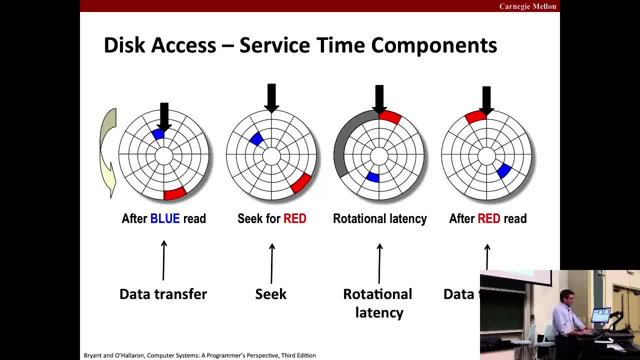 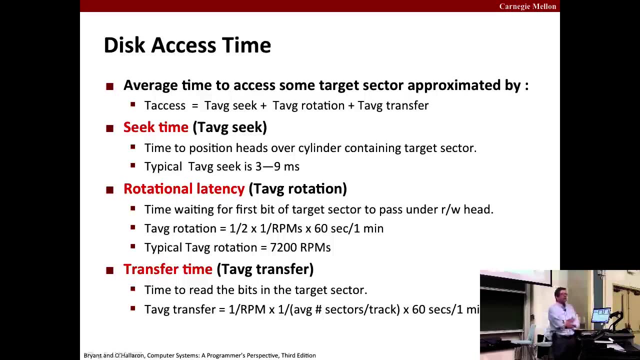 time it takes for the entire to circle all the way around. and then there's the data transfer, which is sort of how long it takes for that, for that track to pass under the read right head. now the reason, the reason it's important to know this- is that 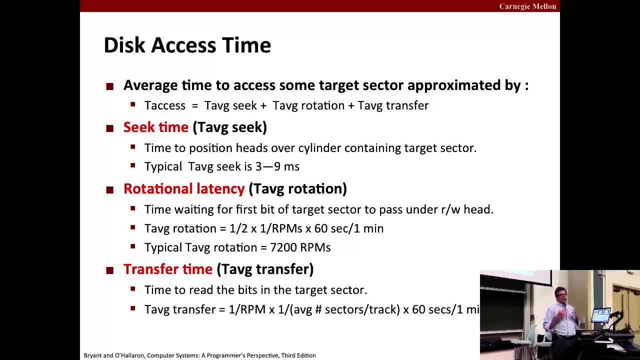 these three components. you add them together and that's the. that's what your average acts time it takes to access data. that time is dominated by the seek time, so seek times are measured in milliseconds, right, so we're moving this head. there's this, there's a servo that has to fire up and and there's actual 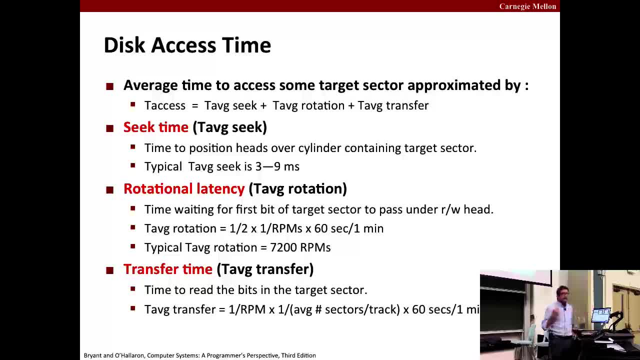 mechanical motion, and that that takes time, and it's on the order of three to nine milliseconds, and this is been true for decades, right? so this, this value, is not changing, right? there's just sort of fundamental mechanical limits that make it very difficult to to decrease this, this value now, the rotational latency, the time that it. 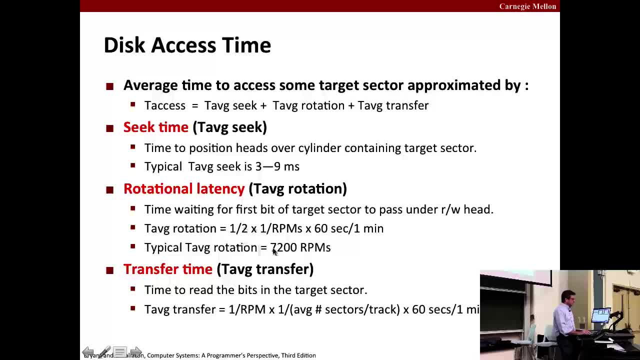 takes to spin around. well, we'll call that the T average rotation, and then the time it takes to read the, the bits will call T average transfer. okay, so we have T average seek, which is this seek time, rotational latency and transfer time. and now, if we just take 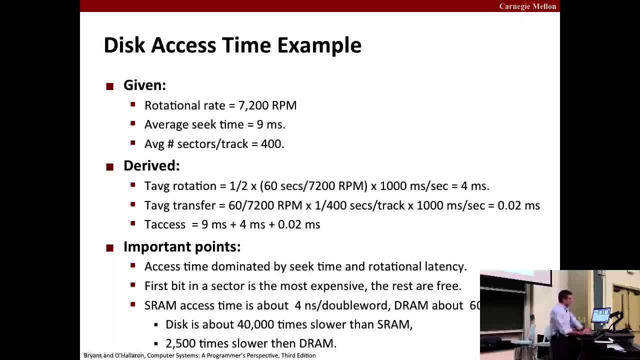 some typical numbers and plug those in. you see that our seek time is on the order of milliseconds. the rotational rate is also on the order of milliseconds, right? so there's there's also mechanical limits, and how fast you can. you can spin these around the access time and the transfer. the transfer time is very small, so it's. 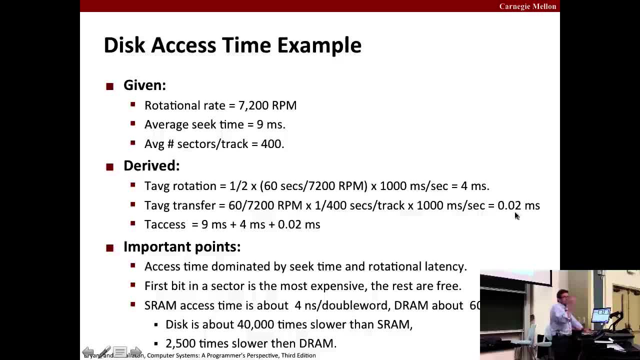 orders of magnitude smaller because you just, you just have to read a few that the bits that are in one sector. okay, so if you, if you look, you can, you can see that the total access time is is dominated by seek and rotational latency. so you know a good rule of thumb, just for sort of estimating how long it. 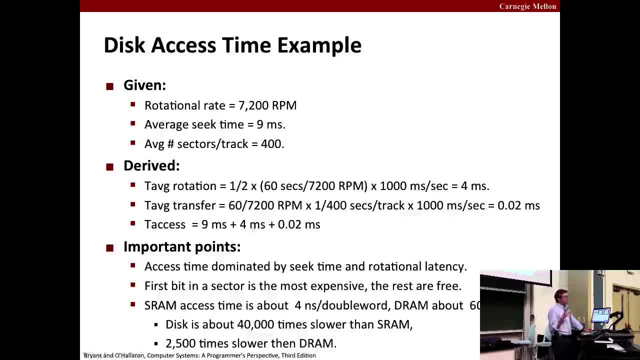 takes to read from a disk is: just take twice the seek, the seek time and you'll be. you'll be pretty close and basically the transfer time is: you get that for free. now. here's the. here's the important thing to know about disks. we SRAM access. 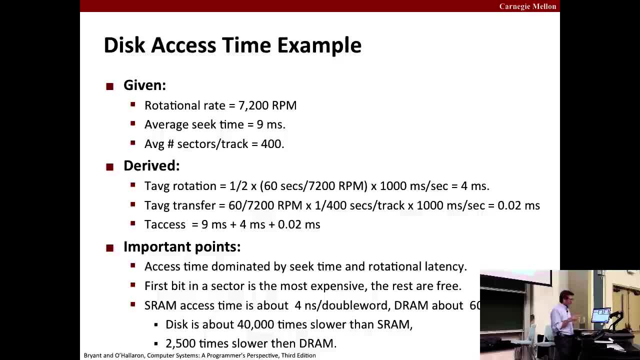 times about four nanoseconds to get a double word. DRAM is about 60 nanoseconds, and so DRAM is about an order of magnitude slower than SRAM. but disk is 40,000 times slower than SRAM, so that's 4,000 orders of magnitude difference. 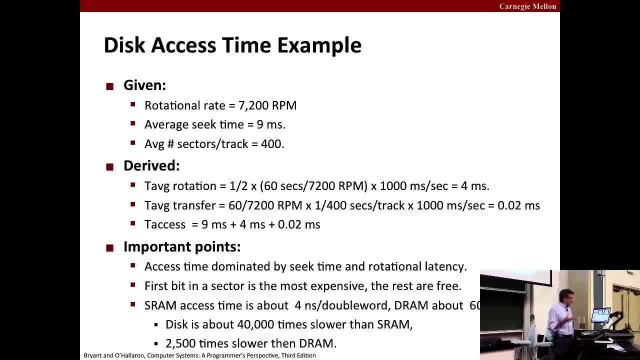 that's huge and it's- it's 250 times orders of magnitude slower than DRAM's. so the the there's a big gap between DRAM and SRAM and there's an even bigger gap between disk and and other other memory types, now modern disks. 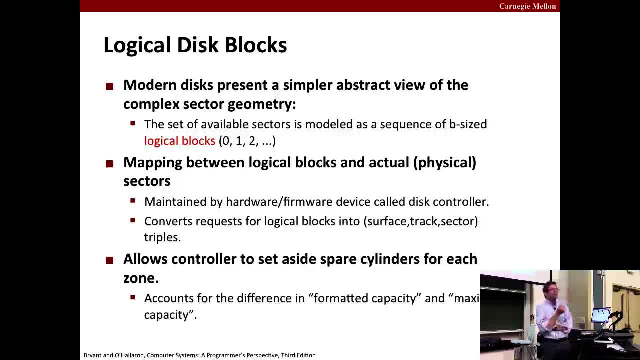 present a much simpler view then. so we then this: this track, cylinder, sector geometry, so modern, modern disk controllers actually present to the CPU. they present the disk as a sequence of logical blocks, where each block is is a multiple of a sector size. so this, in the simplest case, a block is. just think of a. 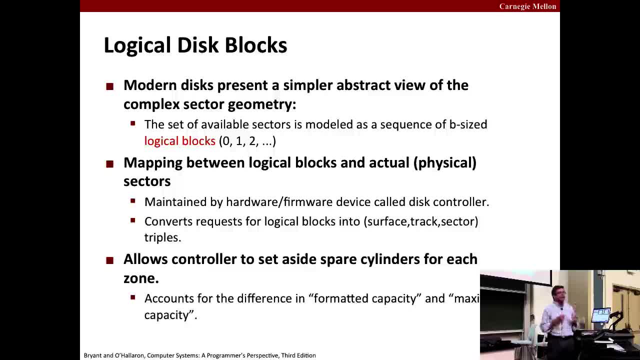 logical block is one sector, and then blocks are numbered, starting at zero, and they just go all the way up to some, to some large number, and then the, the disk controller keeps the mapping, maintains the mapping between logical blocks and the actual physical sectors, so as, as in the old saying, is you know most most. 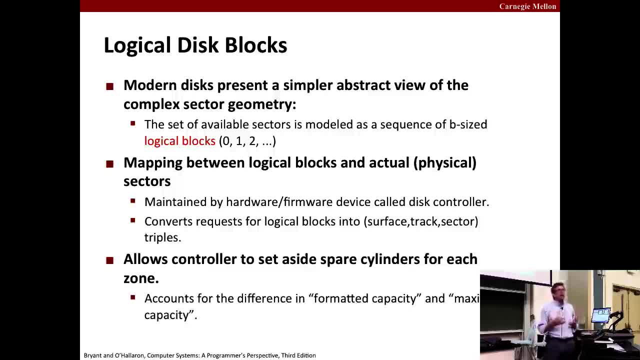 interesting ideas in computer science are involved, some form of indirection. so this is a level of indirection that provides, you know this mapping between logical blocks and physical blocks, so it allows controllers to take some cylinders and reserve them as spare cylinders that aren't mapped in illogical blocks and then, if, if there's, if, one of the sectors, 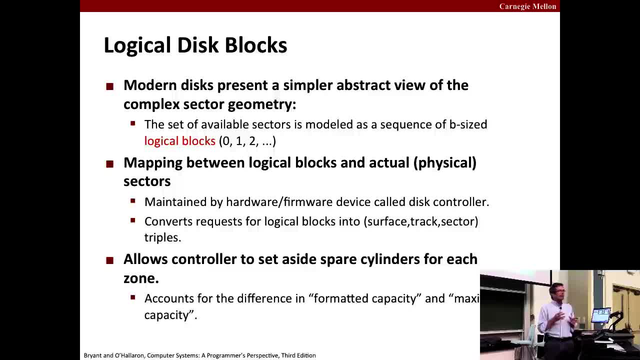 goes bad in a cylinder that the disk controller can can just copy, copy the data over to to a spare cylinder and then just keep going right. so this and so this is why your formatted capacity is is less than sort of the. if you know, if you counted the number of of actual cylinders on the disk you form at a 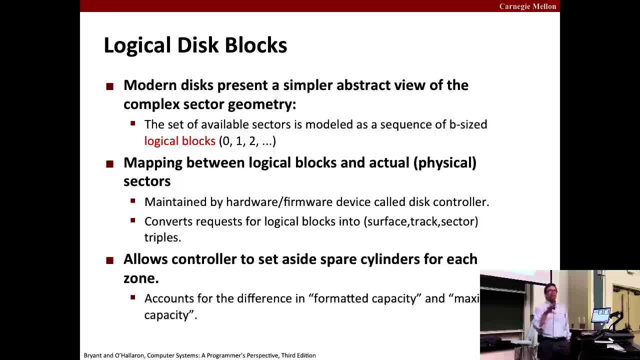 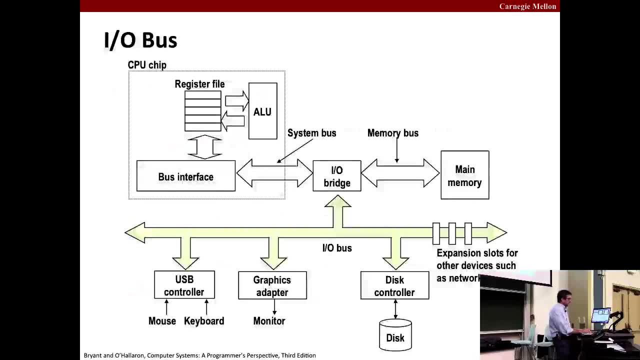 capacity is less than the maximum capacity because some of those cylinders are being reserved for failures. Now, devices like disks are connected to the CPU and the memory via the I-O bridge, over another kind of bus called an I-O bus. This, what I'm showing you now, is actually 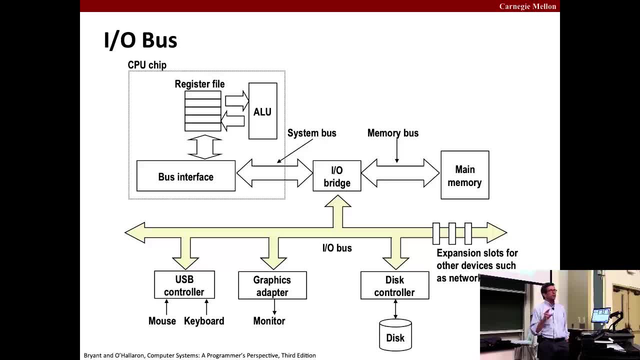 not representative of modern systems. It's representative of what was called the PCI bus about five years ago. Modern buses now are: the PCI bus is a broadcast bus, meaning it's just a single set of wires. So if any device changes the values on those wires, 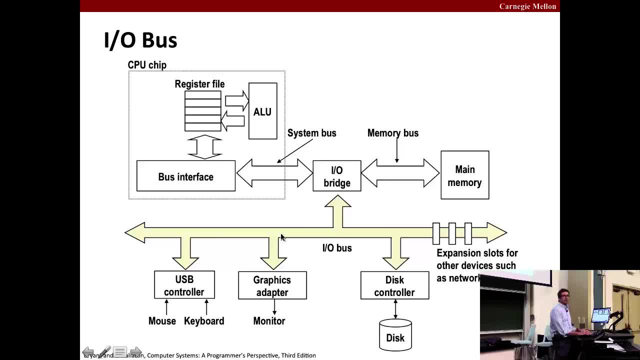 every device on that bus can see those values. That's called a broadcast bus And it's the simplest kind of way to hook things together. Modern systems use a bus structure called PCI Express, which, although it has the word PCI in it, 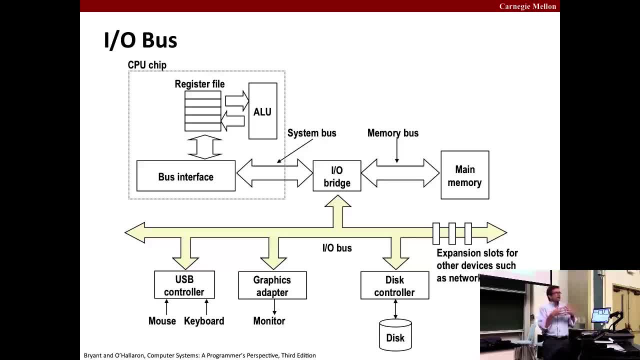 it's completely different. It's point to point. So devices are connected by a set of point to point connections, arbitrated by some kind of a switch, And we won't go into it. It's the same idea. It's a much more efficient design. 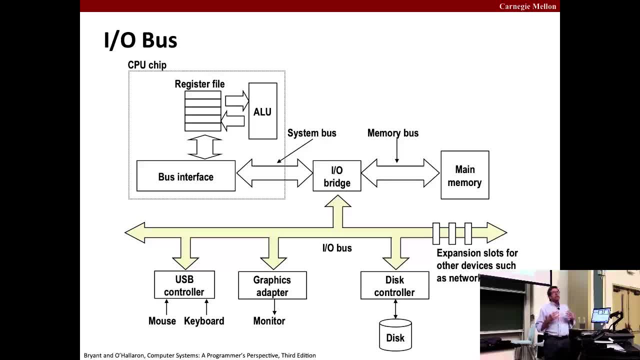 It's much faster, but it provides the same capability. Mainly, it just attaches that, but it allows you to attach all of your devices to your CPU. So just think of this bus as this sort of a single set of wires, where each wire carries a bit. 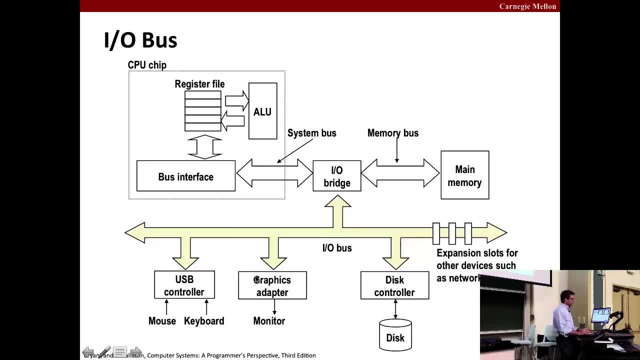 and every device attached to it can see all the values of all the wires. And so there's some devices that are just built directly into the motherboard and they attach to the bus. Like you know, disks are just plugged directly into sockets on the motherboard. 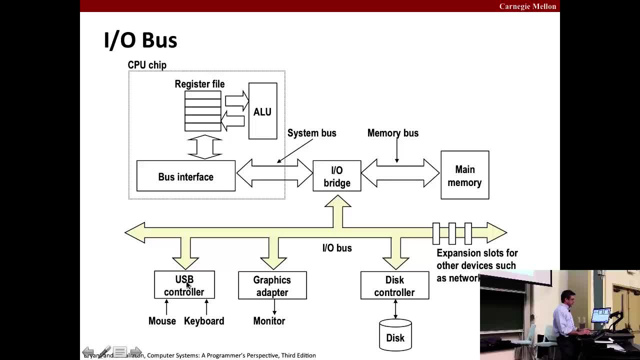 You know your graphics adapter and the USB controller And then the system presents an interface so you can plug mouse things like mouse, mice and keyboards into the USB controller. And then there's expansion slots that allow you that connect to the wires in the bus. 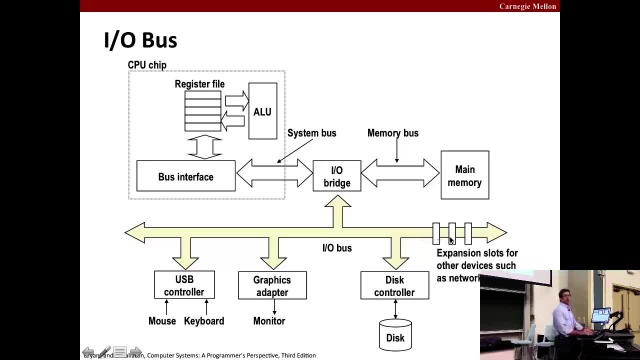 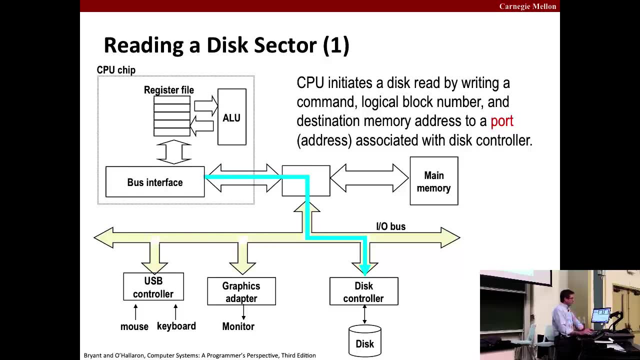 that allow you to add other devices, Like maybe network, you know if you want to put a network adapter in there. Now what happens when we want to read a disk sector? Well, the CPU initiates this read by writing a triple. 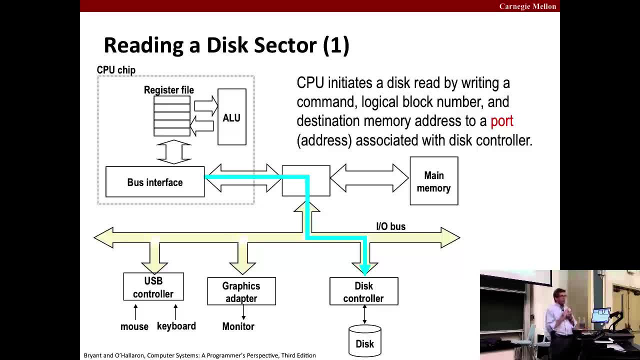 So it writes three different values. It writes a command like say read. It writes a logical block number. So I want to read a logical block number And I want to place the contents of that logical block at a certain address in memory. 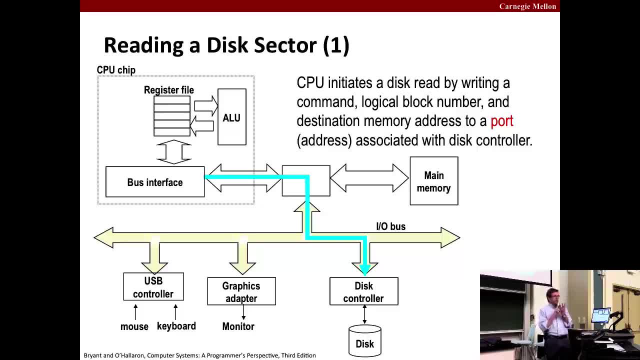 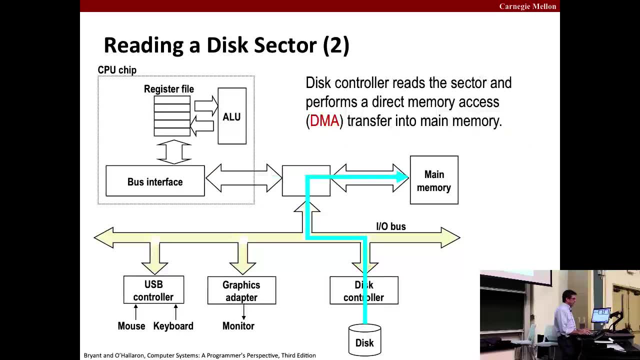 Okay, so it's a command, logical block number and a memory address. The disk controller reads whatever sector corresponds to that logical block. So we'll assume that logical blocks consist of one sector. And then it does this interesting thing: It copies, it takes control of the bus. 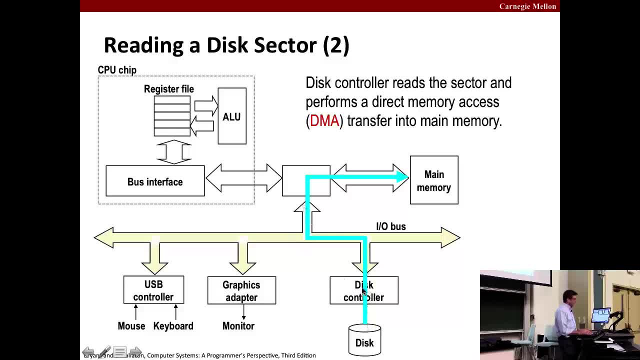 and it copies the data. This is the disk controller now Copies the data across the IO bus, through the IO bridge and directly to main memory without ever notifying the CPU. So the CPU is completely oblivious to the fact that this transfer is going on. 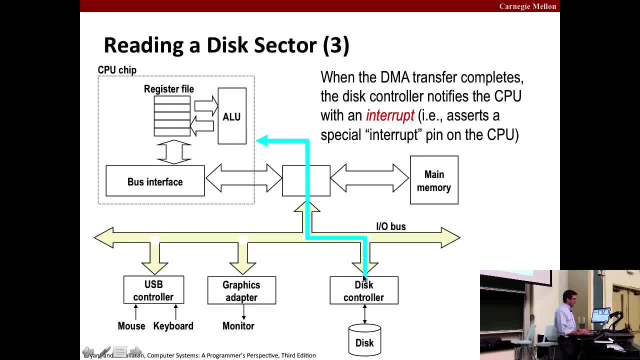 And then, once it's transferred the data to main memory, then it notifies the CPU using this mechanism called an interrupt. So it actually asserts a pin on the actual CPU chip itself. So it changes the value of that pin from zero to one And that triggers an interrupt. 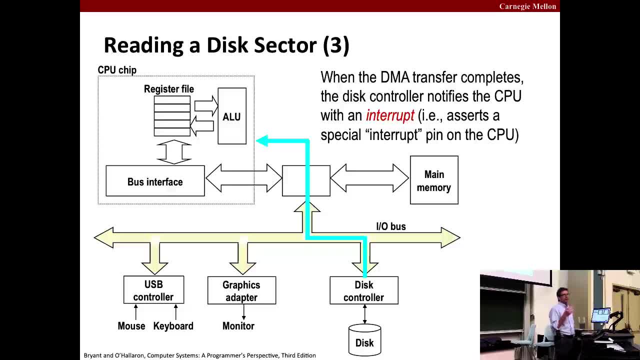 which notifies the CPU that that sector's been copied. Okay, so then the CPU: there's some program somewhere waiting for that data to be read into memory. so now the CPU can execute that program and deal with that memory. So what this? 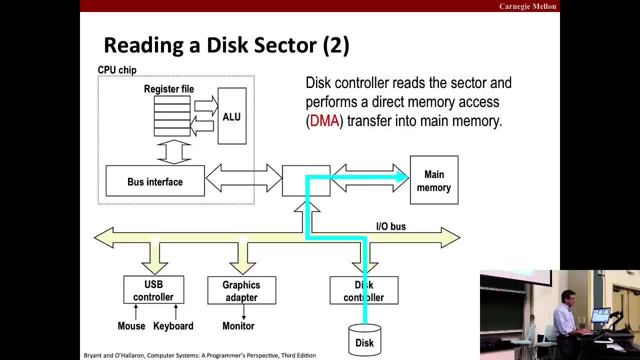 what this mechanism allows, and the reason they do this is because disks are just so godawful slow. Within 10 milliseconds, within 10 milliseconds, a system could be executing millions and millions of instructions. The CPU could be executing millions and millions of instructions. 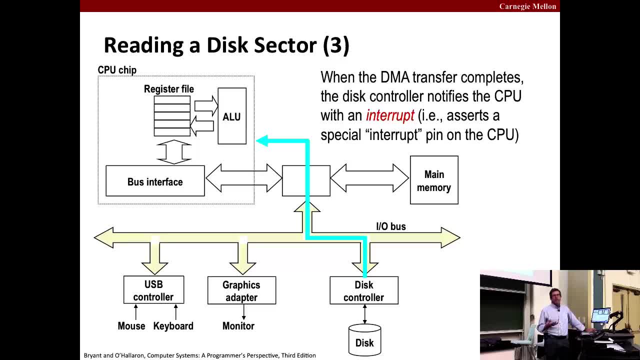 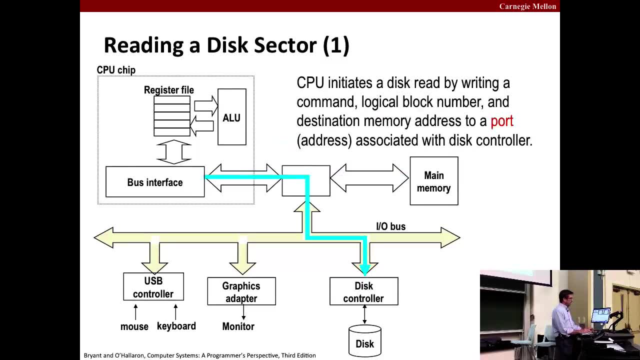 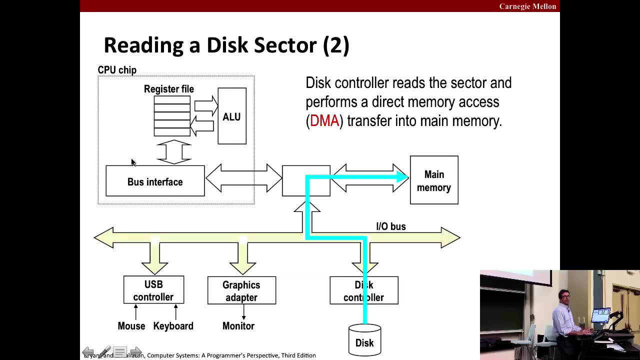 It would be a terrible waste if the CPU waited for that data to come off the disk. So what it does is it issues this request to the disk controller and then, while that really slow, laborious process is going on, the CPU can be executing other instructions and doing other useful work. 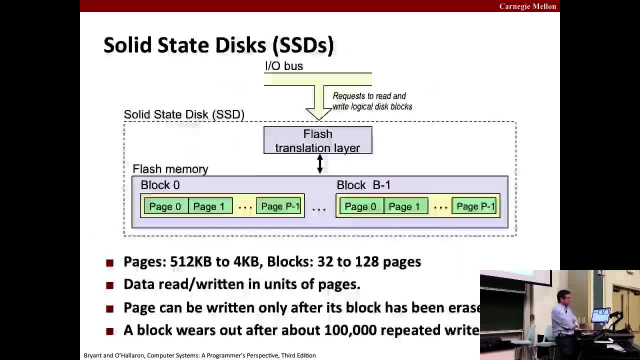 So this is really essential To sort of getting reasonable performance and from keeping this really slow disk system, from slowing the system down. Now there's another interesting high kind of disk called a solid state disk, which is kind of halfway between rotating disks and DRAM memories. 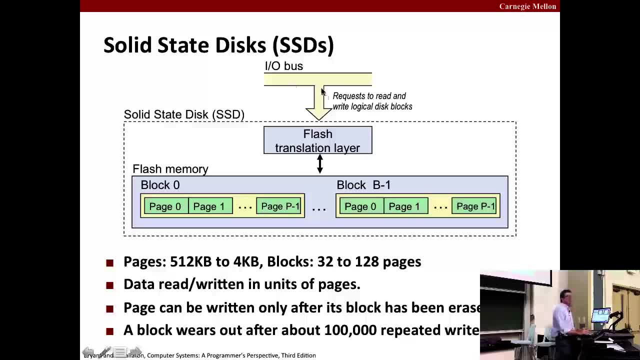 And a solid state disk to the CPU. it looks exactly like a rotating disk. it has the same socket plug. it has the same physical interface. it has the same packaging. it looks like a rotating disk But instead of having all these mechanical parts. 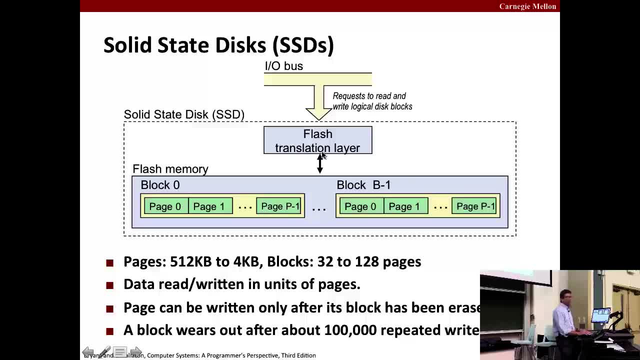 it's actually built entirely out of flash memory and firmware that access the controller. So inside of a solid state disk there's a firmware, a set of firmware called the flash translation layer, which serves the CPU. And that's the purpose, the same purpose as a disk controller does in a rotating disk. 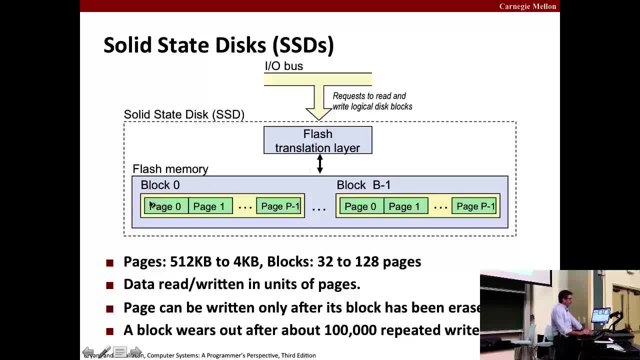 And then the memory itself. the read data can be read and written from the flash memory in units of pages which, depending on the technology, can be 512 K bytes to 4 K bytes, And then a sequence of pages forms a block. Now, these blocks are different from the logical blocks that the CPU does. 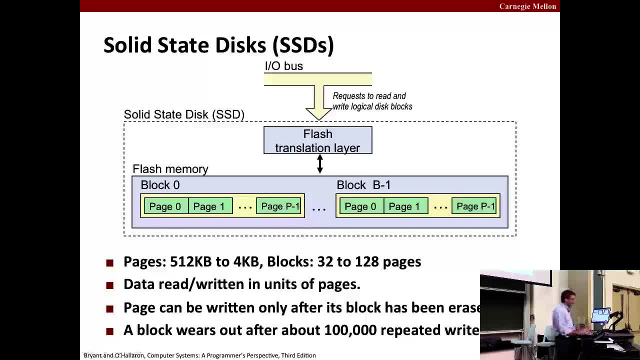 So it's kind of an unfortunate overlap of terms, But the trick is, or the, I guess the limitation is that data is written in units of pages, but a page can only be written after the entire block has been erased. Okay, So that's. that seems kind of weird. 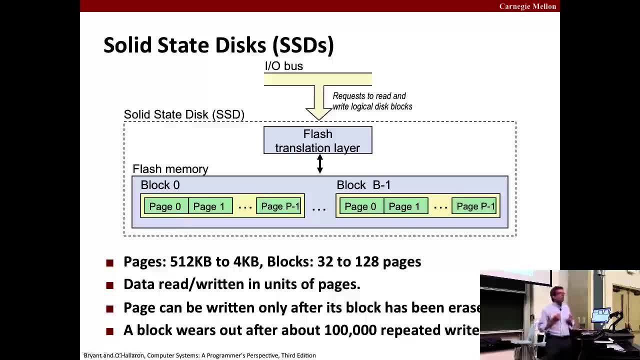 I don't know if you're familiar with that. It seems kind of weird, but that's that's the way it works. So what that means is if you want to write, if you want to write to a page, you have to find a block somewhere that's been erased. 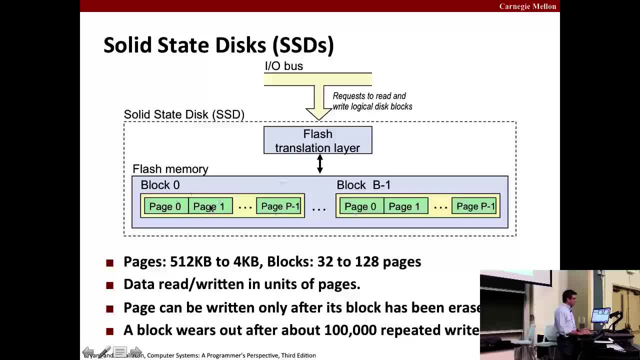 You have to copy all of the other pages in your, in your target block over to that new block and then you can do the write. Okay, So you can see that writes now become fairly complex. operation Reads: you can read anything. 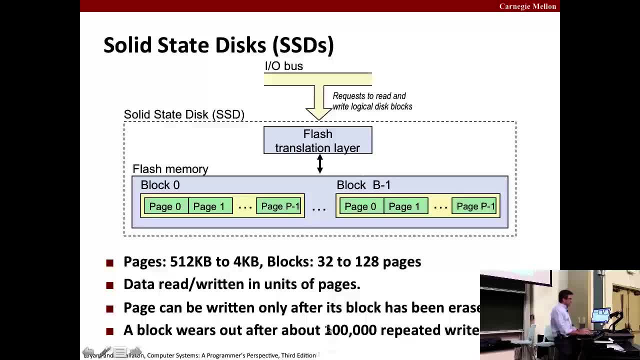 And then, like all Flash, so it's kind of inefficient, right, because you're you're writing one page, But to do that you have to sort of copy all the other pages in that block and you have to erase the whole and then, when you're finished, 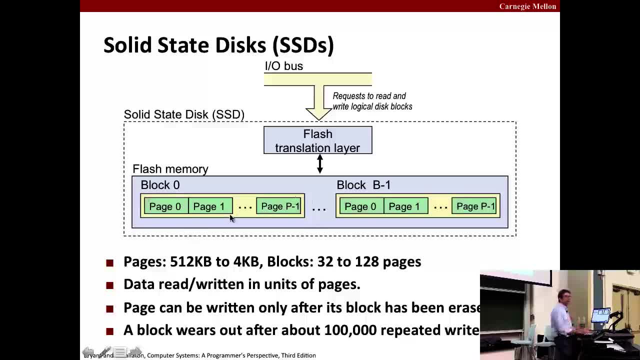 then you erase this block so it can be used for for other writes. So eventually, after 100,000 repeated writes, these, these wear out. Now the Flash translation layers in modern systems do all kinds of fancy proprietary algorithms to sort of extend the life. 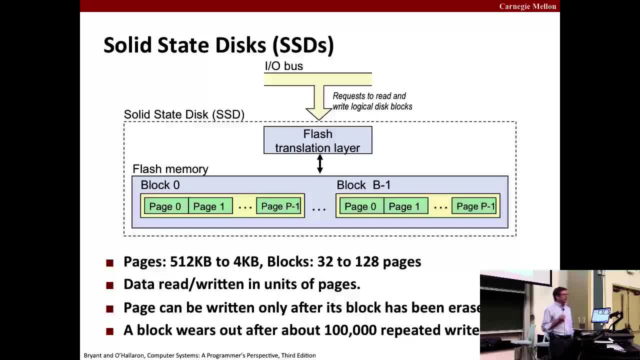 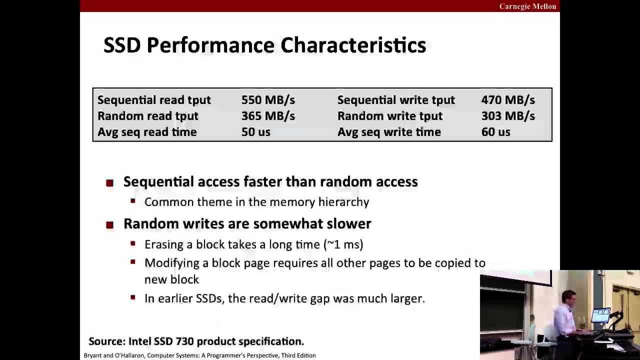 They use caching and and various tricks to extend the life of these SSDs. So in in practice it's not really a problem, which I'll show you in a second. So the performance characteristics of SSDs. now you can think of a typical hard drive. 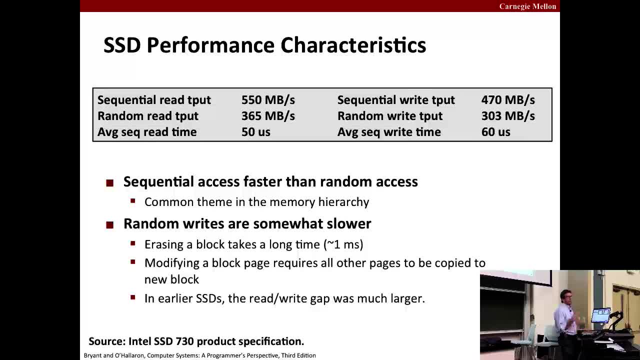 you might be able to get you know. I mean, when I measure them, when I measure my drives, I'm maybe 40, 50 megabytes per second. Okay, And that would be a typical rate. Okay, These SSDs are 10 times faster than that. 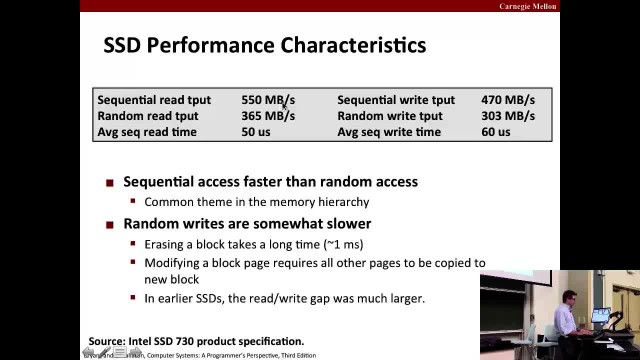 So for sequential reads you can get about 550 megabytes. Sequential writes are a little bit slower. Random access- whether you're reading or writing is- is a little bit slower than sequential access And- and as we'll see this is this- is fairly common. 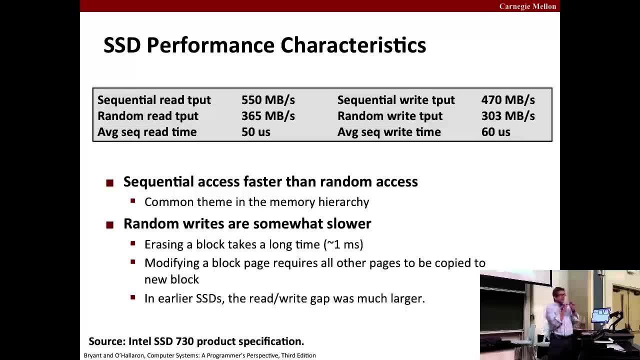 It's. it's in memory systems. it's almost always better to do things sequentially than to jump around. So location is a little bit harder for the recircul. comfy And erasing random writes are slower because erasing erasing takes about a millisecond right. 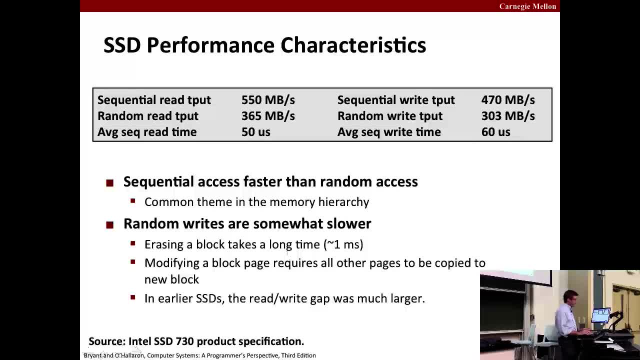 So now we're back up to that, that that millisecond range which is which is slow, And, as I mentioned you, if you modify one, one, one page, all the other pages in that block have to be copied. 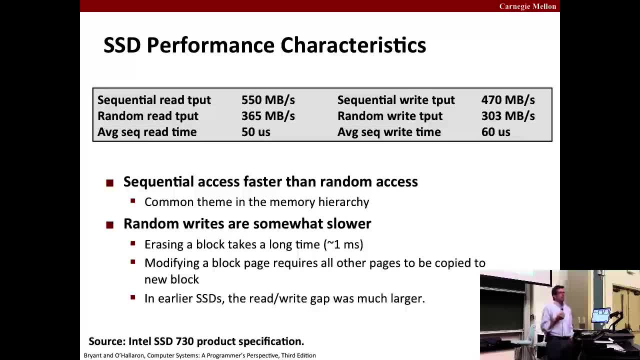 Now, earlier SSDs had a huge gap between random rights and and and sequential reads, but because of sort of improvements in the flash translation layer, these aren't really that difference. right Reading and writing. writing is slower, but they're doing all kinds of interesting amazing. 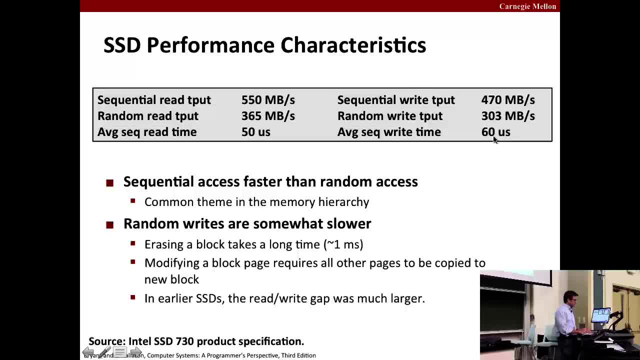 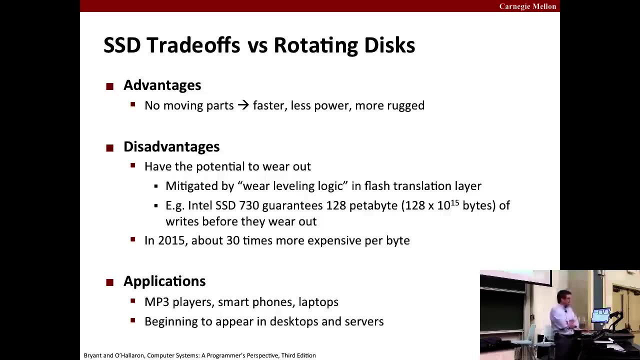 things to get these numbers fairly close. Okay so, when we have a model of SSDs, we really don't need to distinguish any more between reads and writes. Okay so SSDs, because they have no moving parts, they're faster, they take less power. 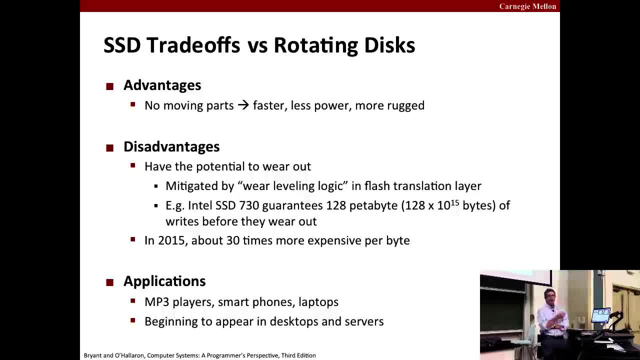 they're more rugged, which is why they're good for thumb drives and iPods and things like that, But they have this potential to wear out, which could be a problem, but in practice it's not. For example, Intel guarantees that you can do 128 petabytes of writes before you're. 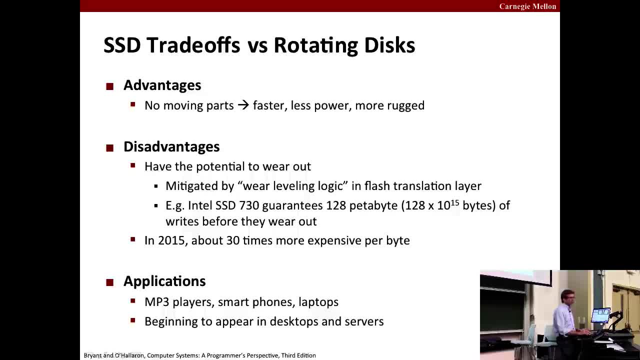 there, SSD is no longer good, So that's a lot of data to write. I mean, think about how many years it would take to write that much data, And as of 2015,, as of now, they're a lot more expensive per byte than rotating disks. 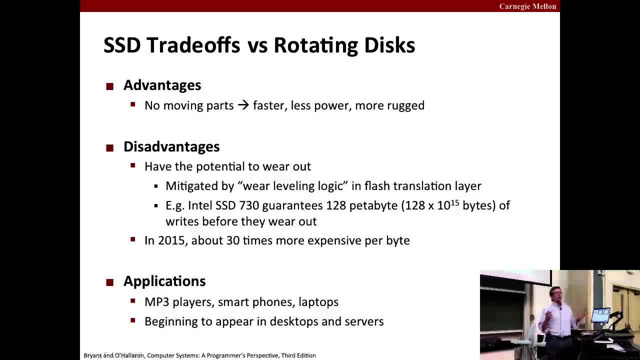 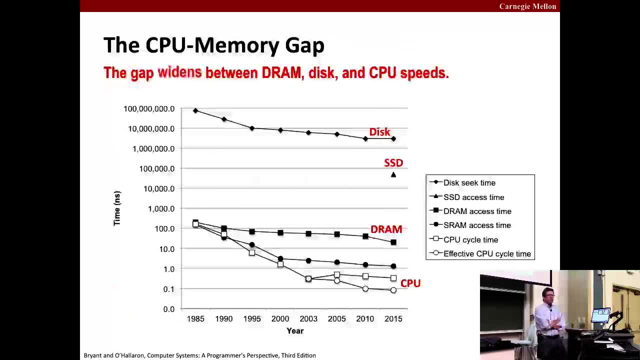 So rotating disks are much bigger, but they're slower. SSDs are smaller and they're faster. Now, If you take, If you look at the performance characteristics of these different storage devices relative to CPU, over time you get this really interesting graph. 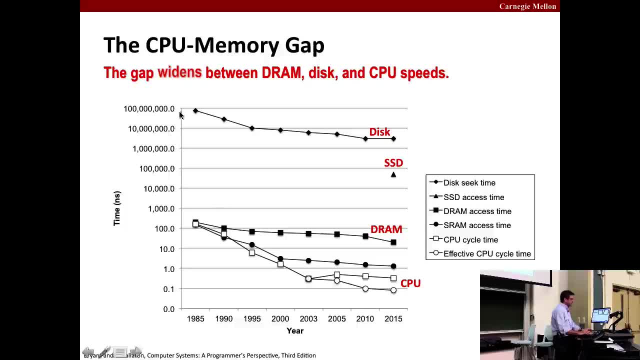 Now this graph shows, on the y-axis, access time in nanoseconds in a log scale. So each one of these, each change in units from 1,000 to 10,000, represents an order of magnitude difference in access time. On the x-axis, I've plotted time going from 1985 to 2015.. 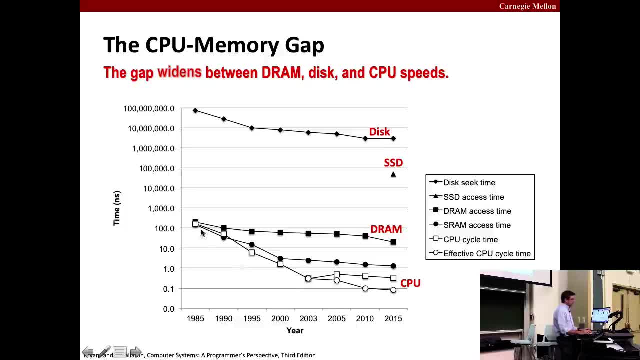 And then I've plotted the access time or the cycle time of these devices: disk, SSD, DRAM and SRAM and the cycle time of processors. So let's look at On the bottom we have the The cycle time of processors over time. 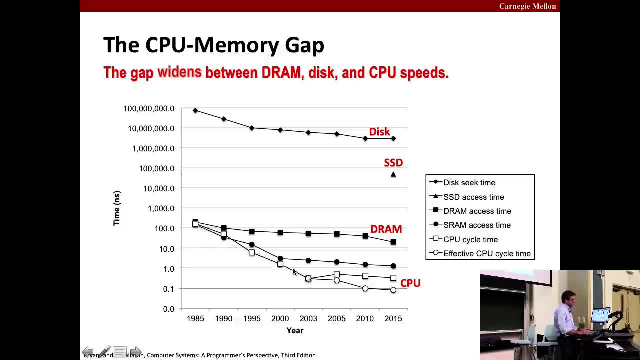 And what you see is it's going down at this sort of exponential rate from 1985 to 2003.. There's a doubling, basically every 18 months or two years in clock frequency and a resulting halving of the cycle time over this 18-month to two-year period. 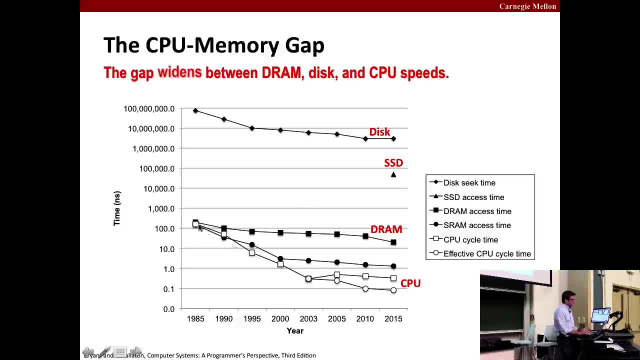 So this, So what? What manufacturers did until 2003 to make their processors faster was they would just double the clock frequency, They decreased the feature size of the chips that they were making, and that would allow them to put things closer together and then have the 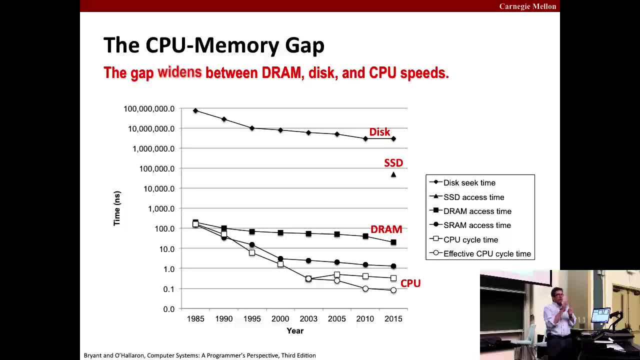 And then increase the clock frequency by a proportional amount. Now this all ended. 2003 was an interesting year. We have year in computer history because of this. there's this sort of unfortunate property that the power that you consume is proportional to your frequency. 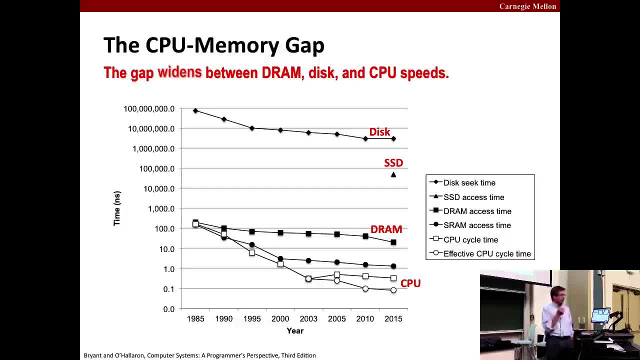 So the more power- I mean the higher the frequency, the more power you consume. By 2003,, the processor that Intel was getting ready to ship was going to burn about 800 watts of power. Think about 800 watt light bulbs inside your laptop. 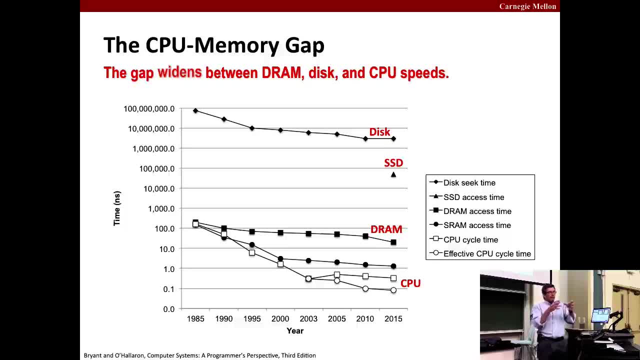 And I actually saw an early prototype of one of these devices and the heat sink to absorb the power from the chip was about this big. it was about four square inches. it was a giant thing just sitting on the motherboard. So that's what we. what we say is that processor design hit the power wall. 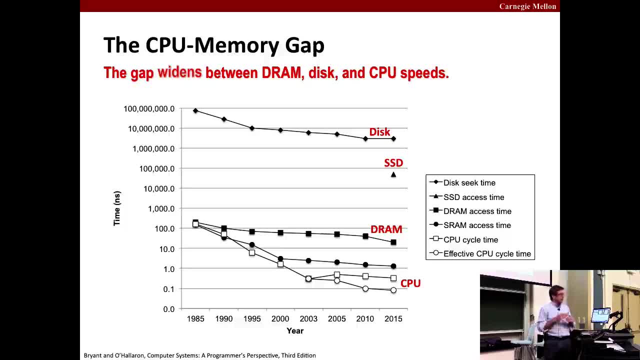 In 2003,. they could no longer just continue to increase clock frequencies to get faster, to make faster computers And what so. what they had to do after 2003,: instead of increasing the clock frequency and try, instead of doubling the clock frequency, they put more processor cores onto the chips. 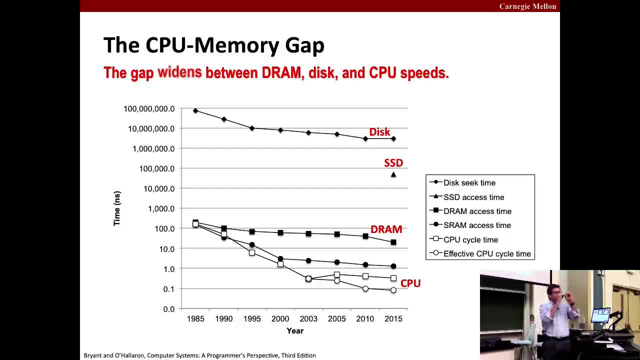 So now they subdivided a CPU chip into individual processor cores And each one could execute its own instructions. And then so, and by running in parallel, you could do more effective work. So the effective cycle time could continue to go down. So what I've plotted here on the bottom is the effective cycle time. 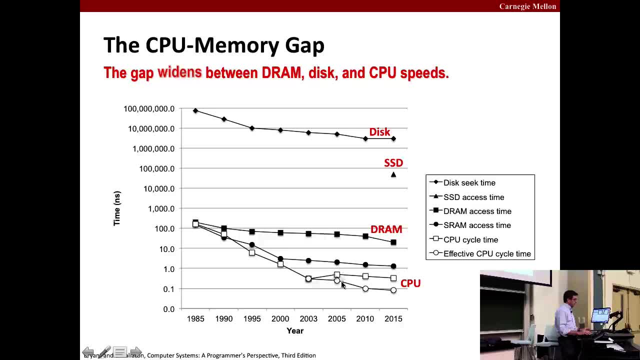 So basically the cycle time divided by the number of cores. So here in 2005,, the first systems used two cores. So now you can run two independent threads or two independent programs, And currently it's about four cores. server class systems you can get eight cores and 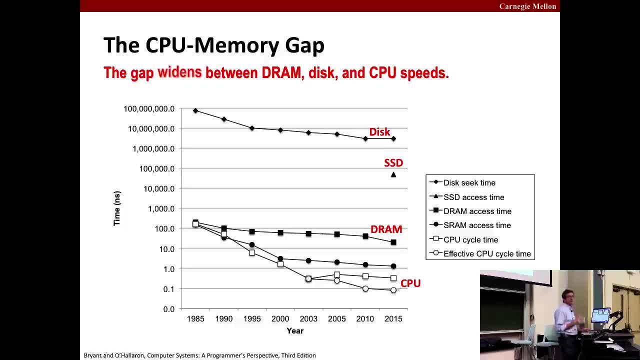 there's even some 12-core chips. So in the future, what's going to happen is that the clock frequencies are going to stay fairly constant. So you can see the, you can see the cycle times. are they actually increased a little bit here? 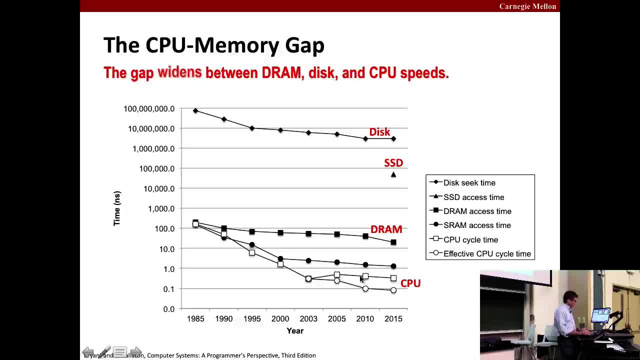 And then they're slowly going down, but it's generally flat, And so the only way to really get more performance Going forward is to increase the number of independent cores, And that's just. that's just the way it's got to be. 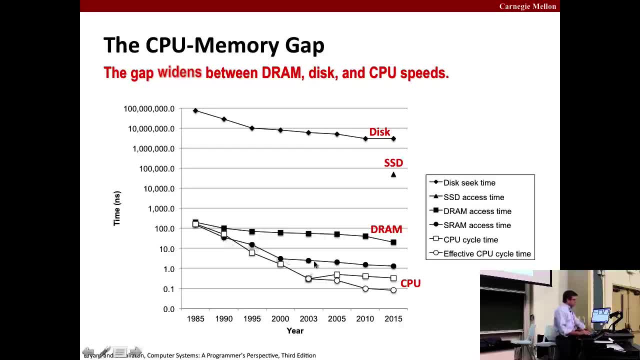 Now here in the black circle, the second line, I plotted the access time for SRAM over time And you can see that SRAM is tracking CPU pretty good And it and there's. it's an order of magnitude slower but it's tracking the CPU performance. 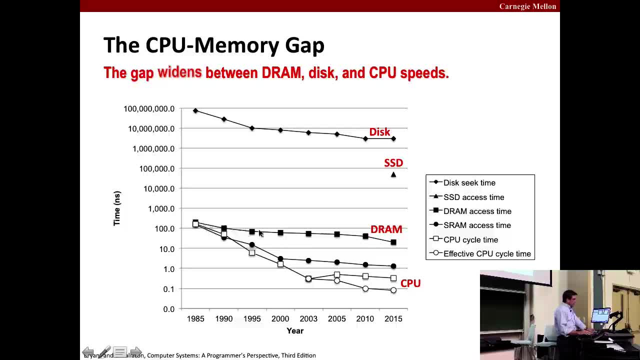 pretty well. And then in the black circle you can see that SRAM. you can see there's a huge gap between the CPU and the DRAM, several orders of magnitude, And in the last few years DRAMs have gotten a little better, but they've, they've proven. 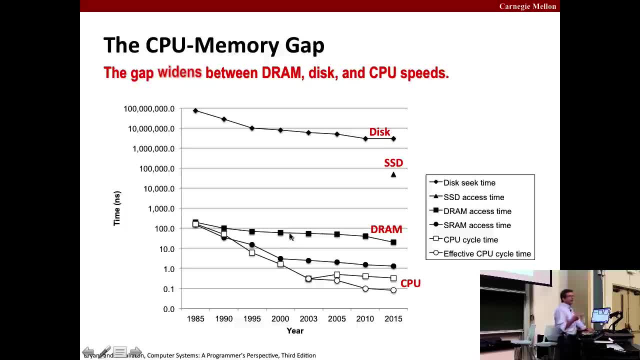 surprisingly difficult to to make faster. SSDs are kind of in between disks and DRAMs And then disks up here you can see at a million nanoseconds. that's the, that's a millisecond, So you can see disks are sort of in this. 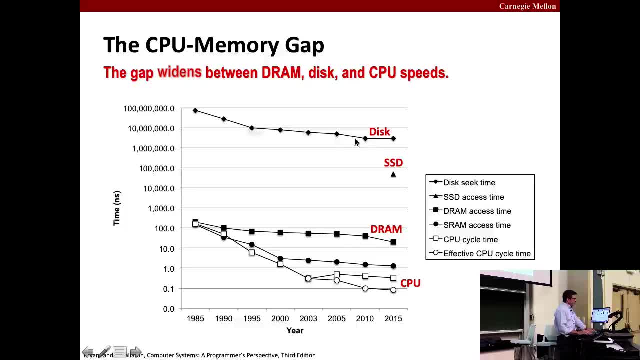 In this sort of millisecond range with access times And those. those have. they've gone down a little bit, but not really too much. So the the point I want to make is that there's this huge gap between DRAM SSD disk and 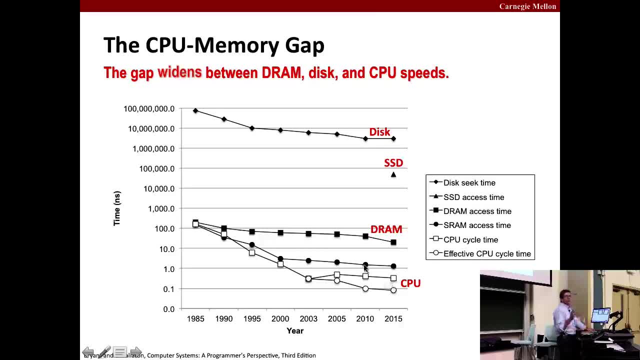 and CPUs, And in some cases it's even getting worse as time goes by. So that's a problem, right? How? How We don't need data. Our data is stored in memory and disk. So if, if, our, if our computers are getting faster and our storage devices are are staying. 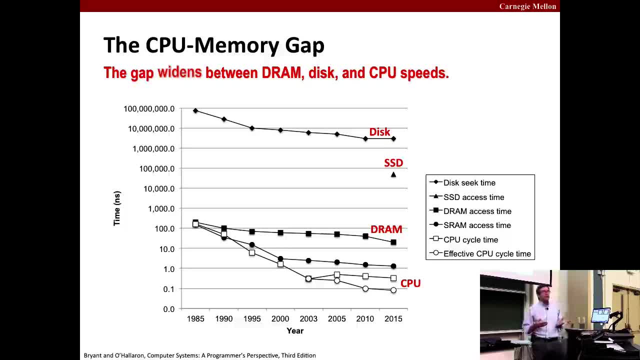 relatively the same or relatively slower, then we've got a problem right. Increases in in our in computer performance, won't? it'll be hard hard to make our programs run faster because we'll be limited by the time it takes to to access the data. 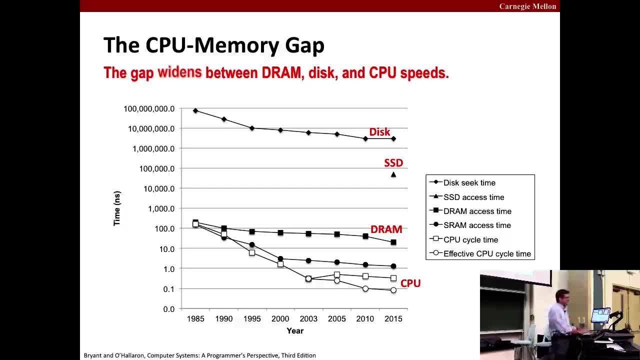 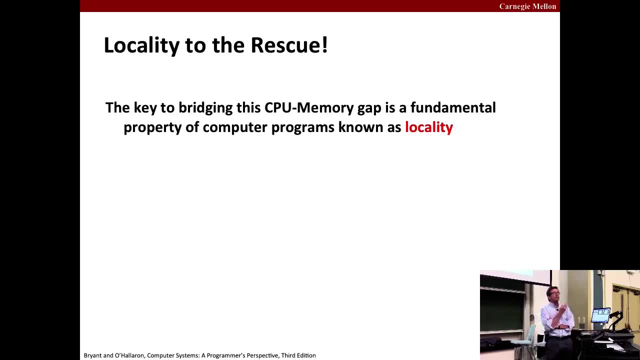 Okay, So that's the. that's sort of the fundamental problem that we have, We have to deal with, And it turns out that the key to bridging this, this gap between the CPU and and memory, is this, is this very basic, fundamental property of programs called locality. 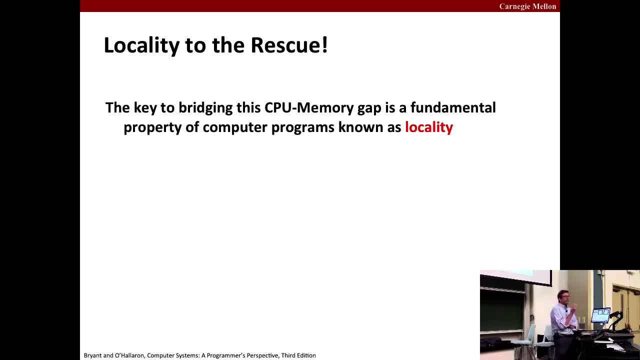 Okay, And so this is an essential sort of fundamental, enduring property of programs. So we say that. So So programs have this property called locality, And what this means is that- I'm sorry, I'll just I have to read it because it's it's. 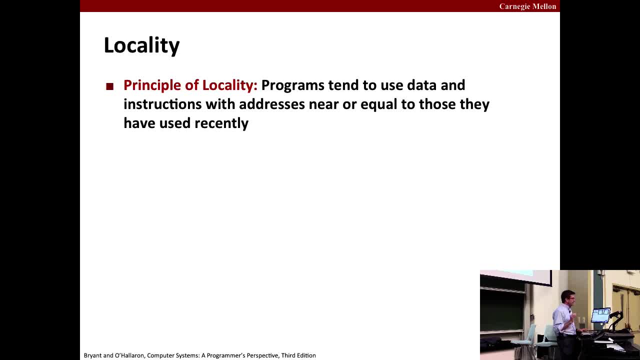 it's really accurate definition. So programs tend to use data and instructions whose addresses are near or equal to those that they have used recently. Okay, So if a, if a, if a program accesses a data item, the chances are very high that it's. 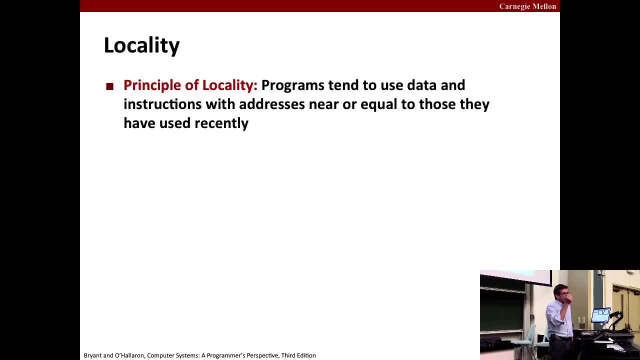 going to access that data item or an address, Okay- Or a nearby data item sometime in the near future- Okay, That likelihood that the program is going to access that data item or a nearby data item in the near future is the. is this property called locality? 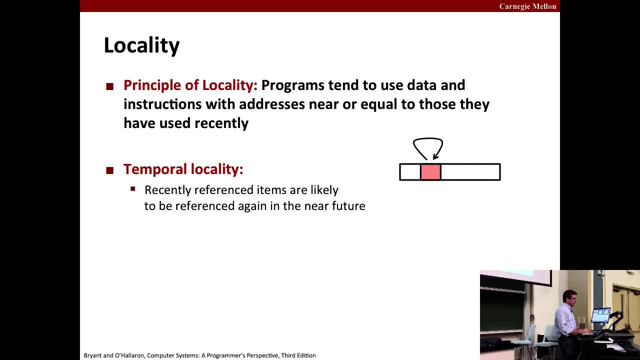 So we'll just. we just typically distinguish two, two different kinds of locality. Temporal locality is the property that recently referenced items are likely to be referenced again in the near future. Okay, So, if, if so, if you read a variable, chances are you're going to read that variable again. 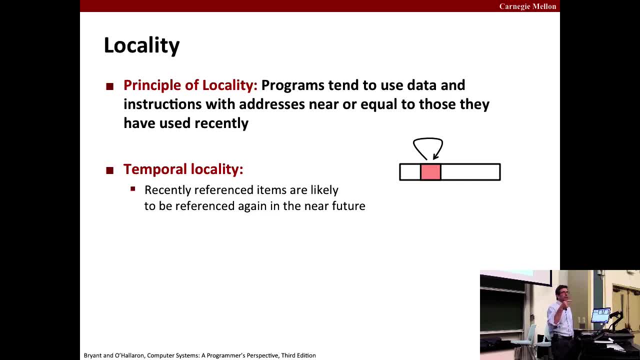 For example, suppose you're summing into a variable inside of a loop Each loop iteration, you're going to access that that variable. Okay, Spatial locality is that the tendency for items with nearby addresses that items if we access, if we access one item, chances are high we're going to access a nearby item. 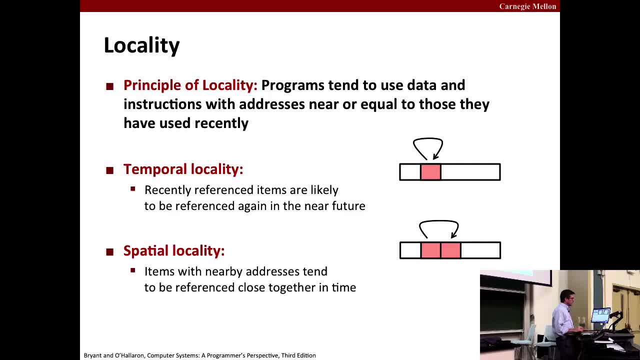 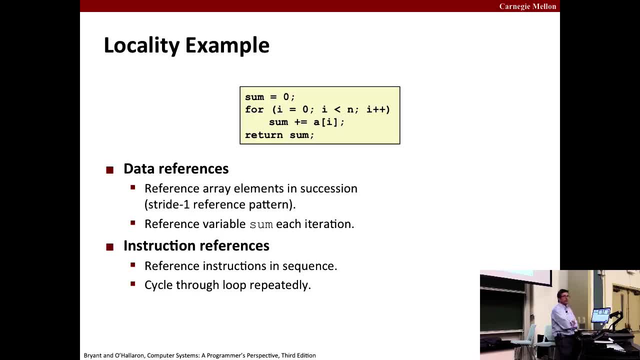 Okay. So let's look at this little snippet of code and see if we can identify all the different kinds of locality in this code. So we have two different kinds of of references. There's data references and then there's instructions, right? 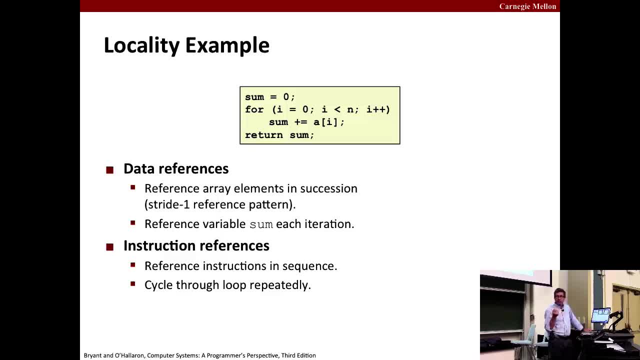 So we're we're reading instructions out of memory, and those instructions are referencing data. Okay, So, first of all, notice that we're we're referencing the elements of an array in succession. Okay, So we're increasing i by one each time, and then we're, so we're incrementing i each. 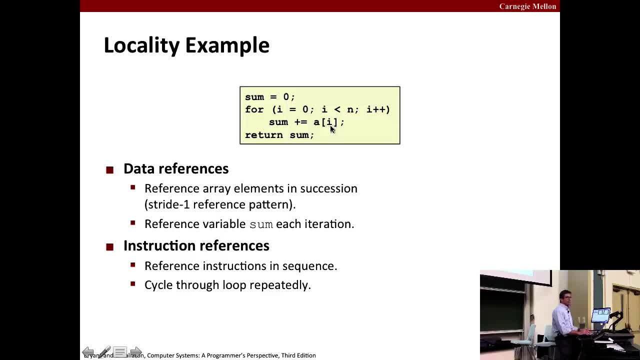 each iteration through the loop and we're reading ai: Okay, So this is called a stride one reference pattern, The. the stride is how much we're incrementing this, this index. So we're, since we're incrementing it by one, we call that a stride one pattern. 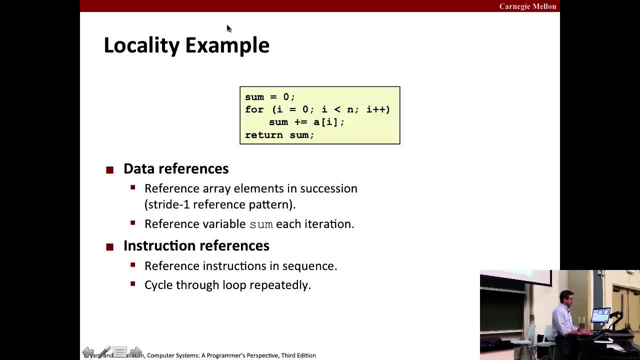 So what kind of? what kind of locality is the? these repeated references to ai? Okay, So what kind of locality is that? Spatial or temporal? Spatial- Spatial, right Cause we're accessing nearby items. Okay, What about the referencing this, this variable sum inside the loop? that's temporal. 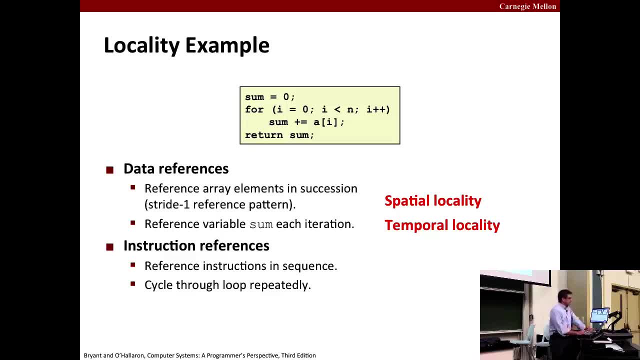 Now, what about instructions? So we're we're referencing, we're each loop iteration, we're reference, We're executing a sequence of instructions. So what kind of locality is that Temporal, within each loop iteration? No, that's spatial, right. 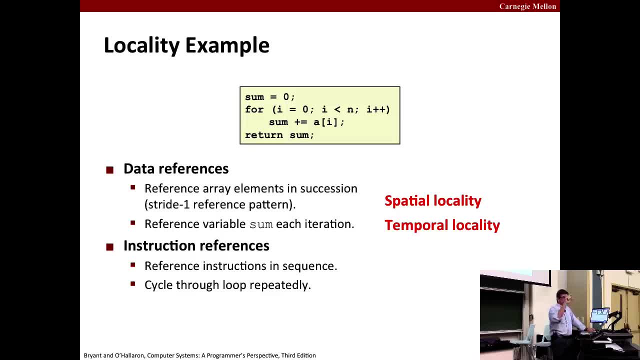 Because we're just executing a sequence of instructions within each loop iteration, But then we cycle through the loop repeatedly. So each loop iteration we're going to access each of those instructions that we accessed the previous loop iteration. So we go up and we're just going to keep executing. 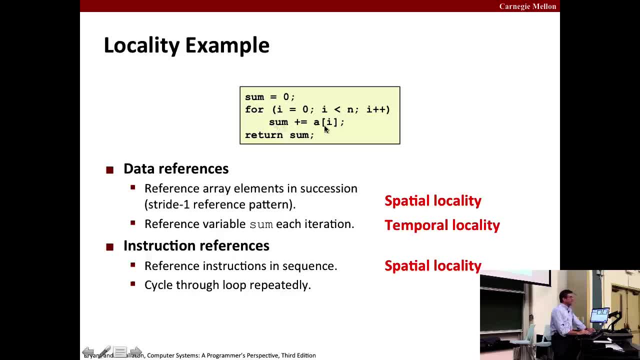 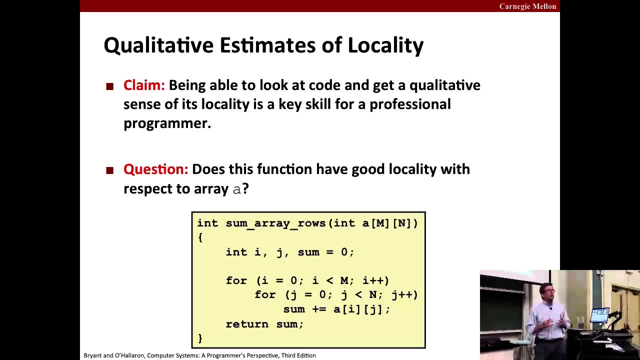 the same assembly language instructions that implement this loop body. Now, in this simple example, it's probably this one instruction, But in general your loop can have multiple instructions. Now what I claim to you and one of the main sort of points of this whole course: 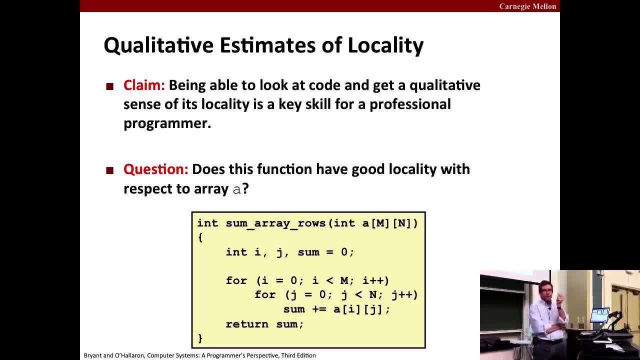 is that, as a professional programmer, it's an essential skill that you be able to look at code and get a qualitative sense of its localization Because, as we'll see, good locality turns into good performance, the way that systems are built these days. So, as a programmer, it's very important for you. 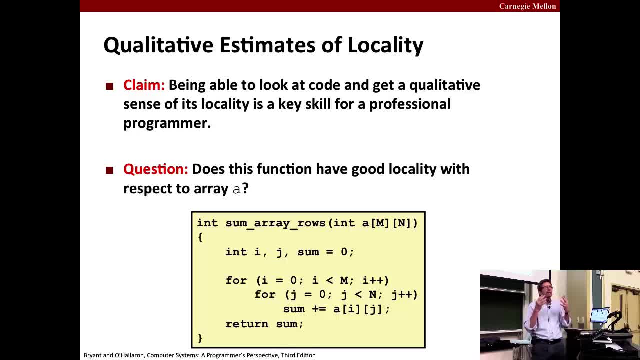 to be able to kind of look at code and get some qualitative sense, Like, eh, that's pretty good locality, That's terrible locality, right. And what you want to do is avoid the terrible locality in your code. So let's look at a simple example here. 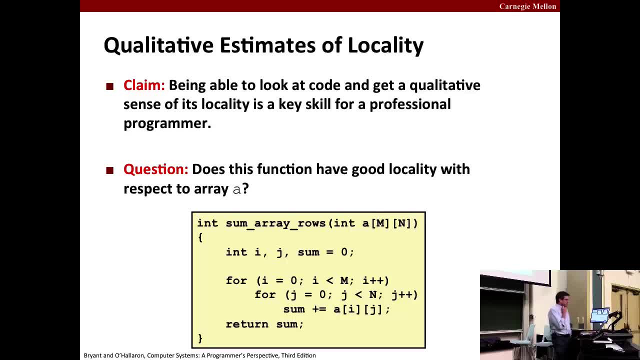 to see what I mean by this. So what I'm doing is I'm taking an array, a two-dimensional array A with M rows and N columns and, within a doubly-nested loop iterating on I and J, I'm summing the elements of that array. 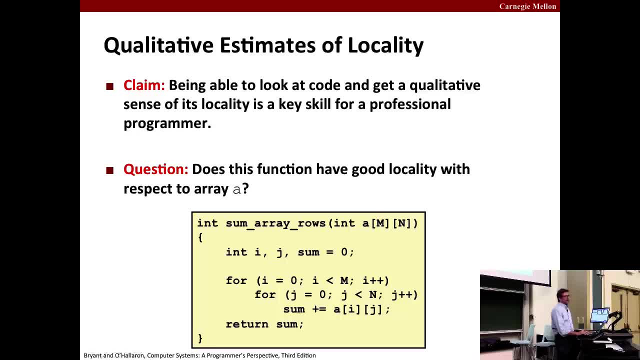 Okay, it seems this is a very simple operation. What could go wrong? right, So it turns out, if you write this code, you have got to be able to do this. You have got to be able to do this. If you write bad locality, it'll run. 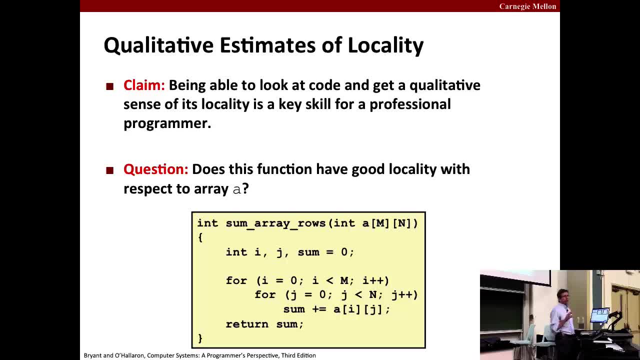 order of magnitude slower. So just look at this. If you look at this, do you think this has good locality or bad locality? I mean, let's look at the with respect to the accesses of A Good or bad Good. 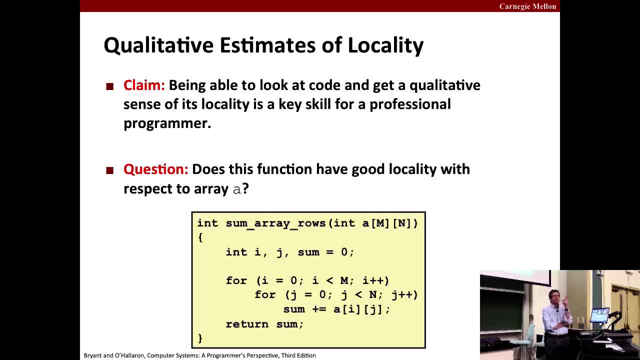 Well, so how is A laid out in memory right? It's row-wise, right? So C lays out arrays row-wise, So all the elements of the first row, followed by all the elements of the second row, followed by all the elements of the third row. 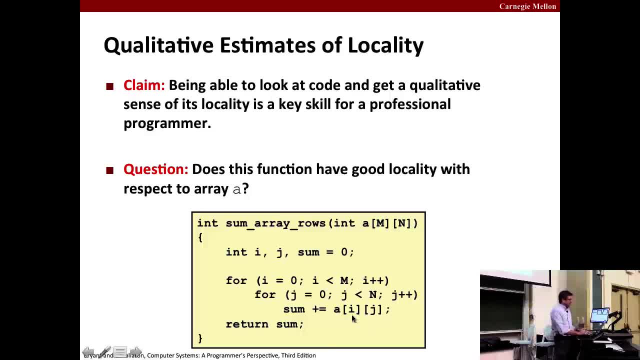 Okay, so how are we accessing this array? Look at, we're accessing A, I, J and we're varying J the fastest. So we hold I constant and then we vary J and then we access all. so we hold I constant to access row I. 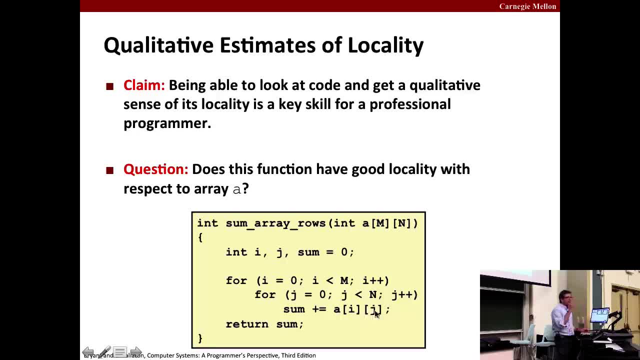 and then we vary J to access all the columns in that row. Okay, so each each and then we increase, and then we go back and increase I. So now we're accessing the next, the next row. Okay, so if we were to look at the addresses of A, I, J, 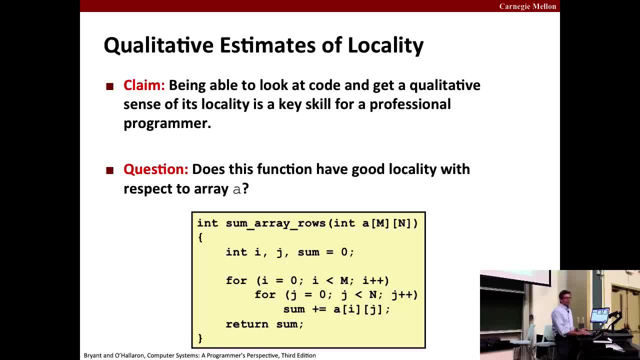 the sequence of addresses that are being read. those would correspond to a stride one access, and so we'd be accessing all the elements of of A sequentially in order. Okay, so that's really good. spatial locality- right, That's the best you can do. 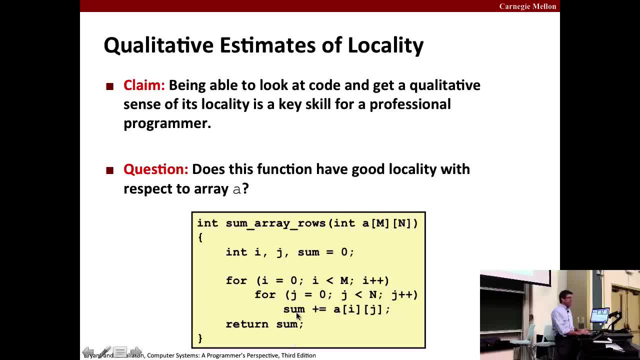 Now what about? what about? and then we have temporal locality, and then we have interlocality on some. so that's good, right. So everything about this is pretty good. So this is the good case. Now, what about this? 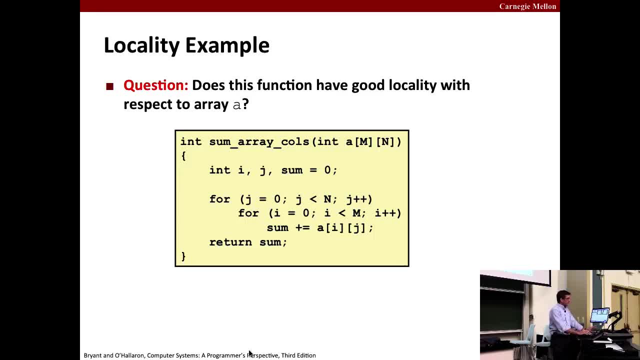 What I've done. I've taken the same program and I've just inverted the loops. So I loop on J first and then on I, and then I just have the same inner loop body. Now, what does that do to this? 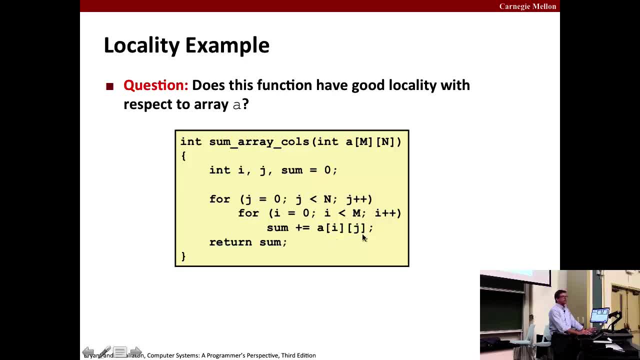 what does that do to the spatial locality of our accesses of A, Yes, Terrible spatial locality? Terrible because it's going. you should be offended when you see this. This is awful, But it's, it's terrible, right. 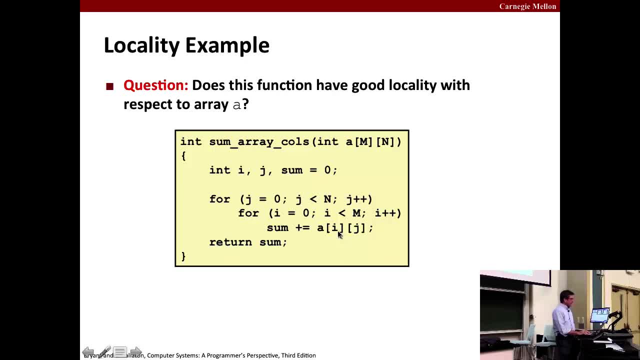 Because look at, so we're now, we're holding J, we're holding J constant, and then we're iterating through the Jth element of each row, so that's skipping. We have N. we have N elements in each row. 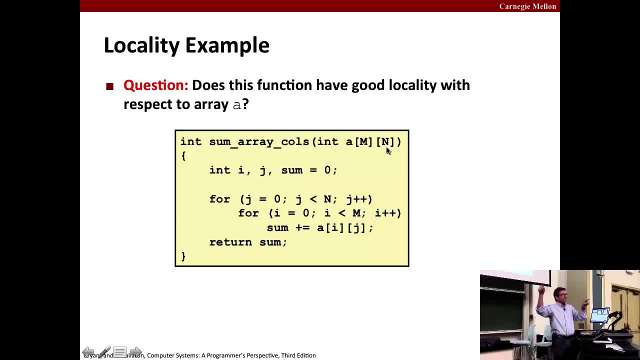 so we're doing a stride N access through memory. So we're going like this and then we're incrementing, then we're looking, then we're incrementing the column by one and then we're doing this again. So it's terrible spatial locality. 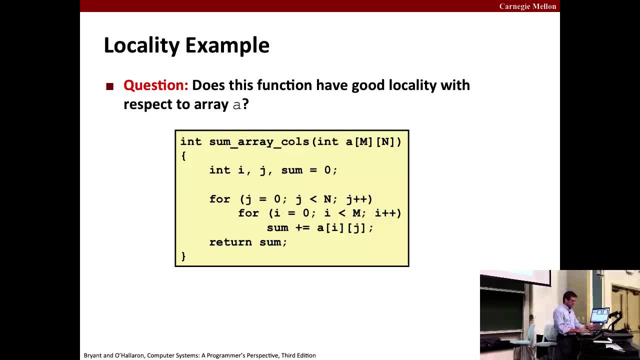 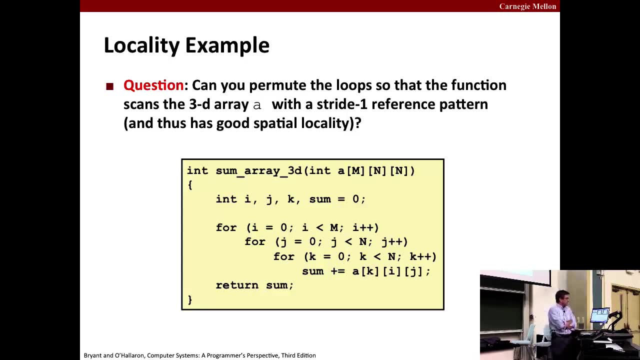 This is the worst spatial locality we could get. Now let's look at a three-dimensional array And let me ask you the let me pose the following question: Can you, based on this sort of qualitative idea, this idea that you want to try to get, 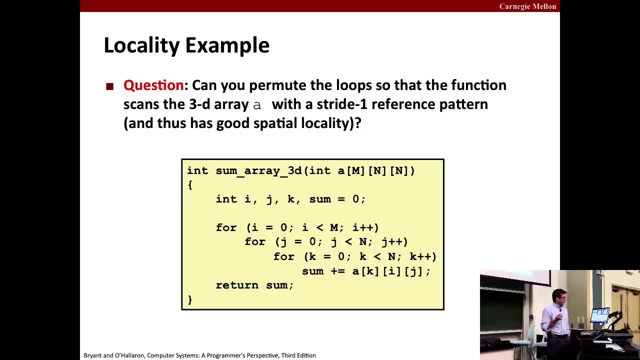 a stride one reference pattern. okay, so how would you permute these, given this inner body, A, K, I, J. how would you permute these loop indices to give a stride one reference pattern? K, that's right, K I J is right. 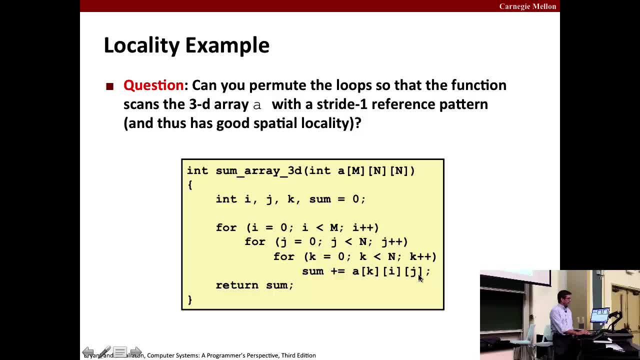 So what, in general, what we want to do is we want to go going from right to left. we want those indices to be changing the fastest. So we want J, we want K and I to be held constant, and then we want to change J. 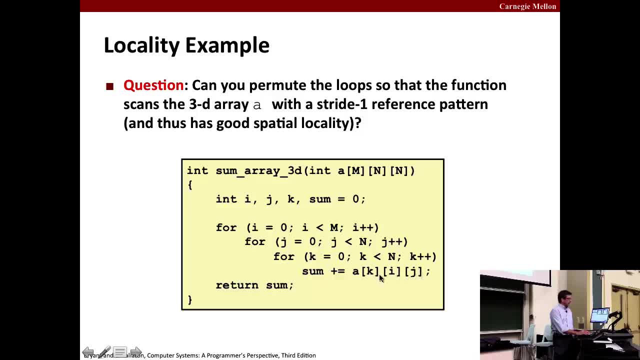 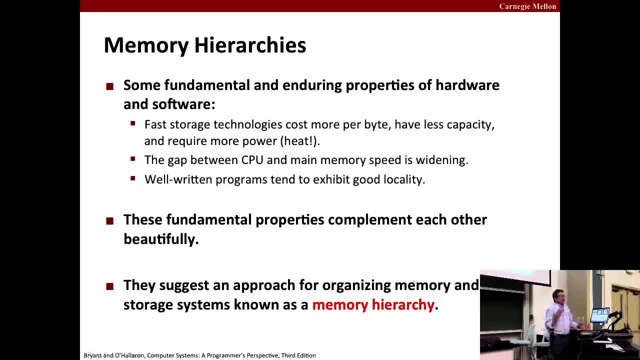 Then we want to increment I and then for that value, those values of K and I, we want to sequence through all the values of J again, Okay, Okay. so we've looked at properties of technology, of storage technologies and what we 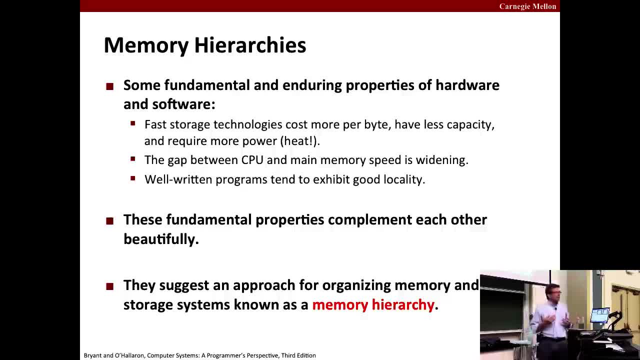 and there's this sort of basic, sort of fundamental principle that cheaper storage, bigger storage, higher capacity storage is cheaper, More expensive storage is smaller. right, because we just don't have enough, we can't spend enough money. There's this gap. there's this gap between our storage devices. 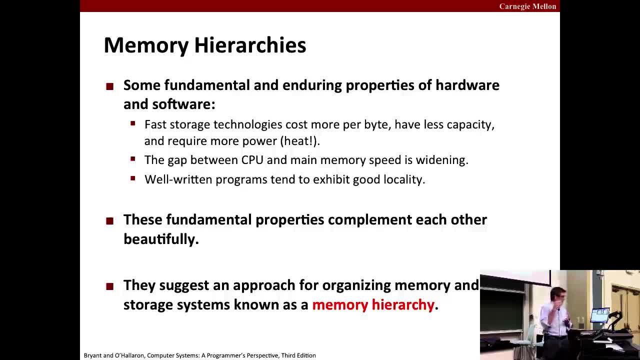 and the CPU that, at least in the case of disks, are getting bigger and we have programs that exhibit locality. Okay, so these three things, these properties of storage technologies and properties of our programs, complement each other in this beautiful way to suggest and inform the design of our storage systems. 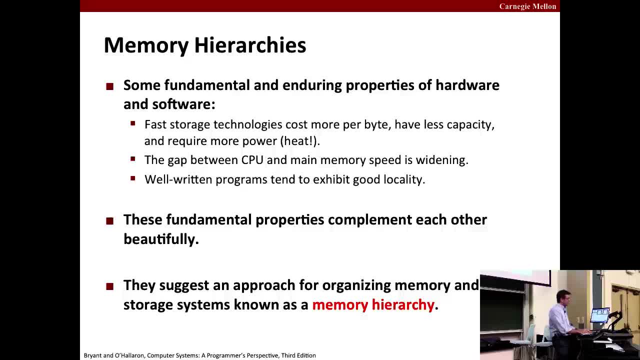 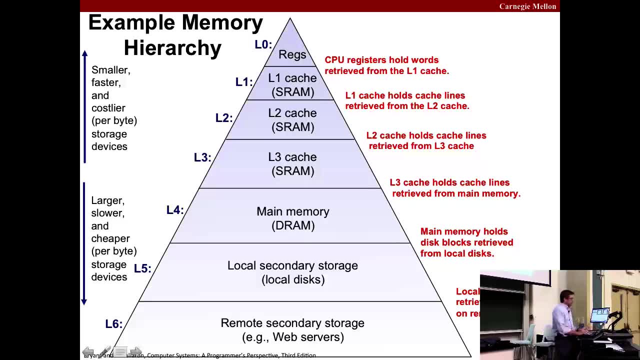 And this design is something called the memory hierarchy. Okay, here's the idea of a memory hierarchy. You layer instead of a flat memory system. you now you create your memory system as a hierarchy of devices and at the top of this hierarchy, 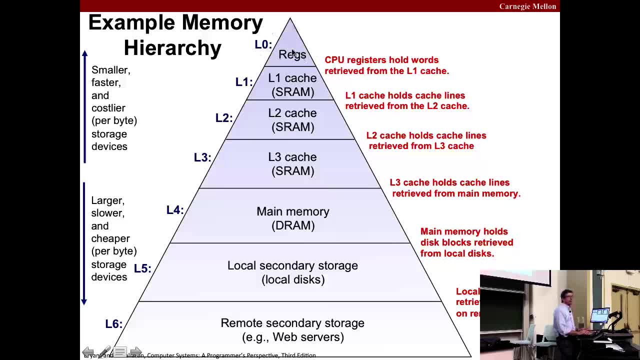 you have your smaller, faster and more expensive storage devices. So at the very top, you have registers which are which can be accessed within one cycle right One instruction, while that instruction's executing can access, read and write into a register. 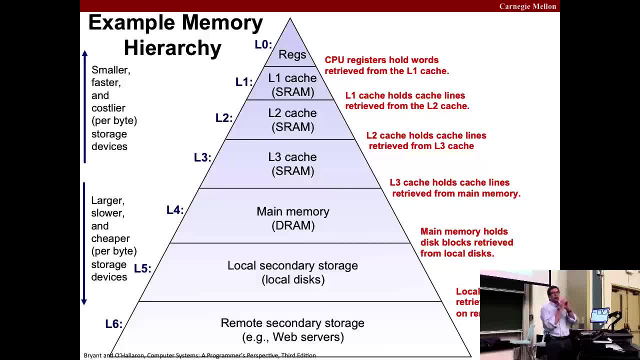 Okay, so registers are at the top of the hierarchy, But because those are in custom silicon, they're very expensive, right? The fabrication plants to make processors cost billions of billions dollars. okay, so this is the most expensive, and because of that it's also. 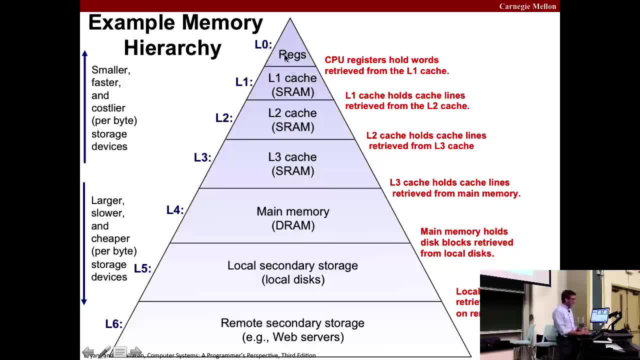 the smallest. we've only got 16 registers at the top of the hierarchy now below that we put one or more SRAM memories. remember, SRAM is faster, it's the fastest kind of memory. so we put one or more so-called caches- cache memories built out of SRAM- in the processor chip itself. 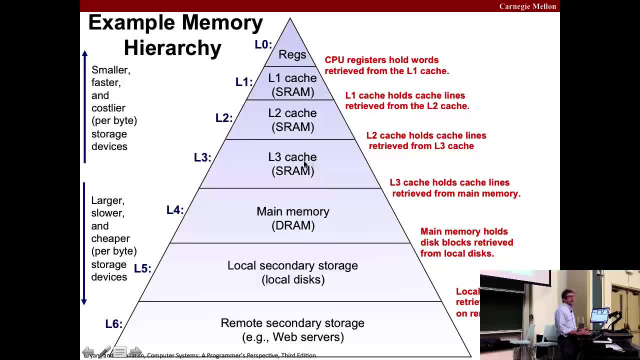 and then and these caches, because they're made out of SRAM, they're on the order of megabytes in size. okay, they're much bigger than registers, but they're. they're megabytes okay which, if we look, and then beneath that is our main memory, which is built out of DRAMs, and those can be gigabytes. 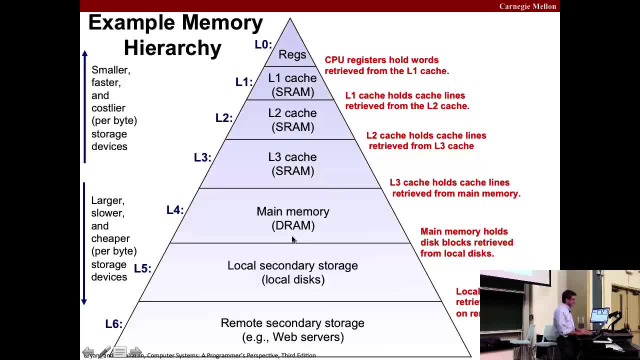 tens of thousands of megabytes and then we put one or more of those in the disk and we have thousands of gigabytes on modern systems and then below that is our local disks and we can even have lower layers like web servers that are storing. you know, if we're storing stuff on Google, that you can think of that as. 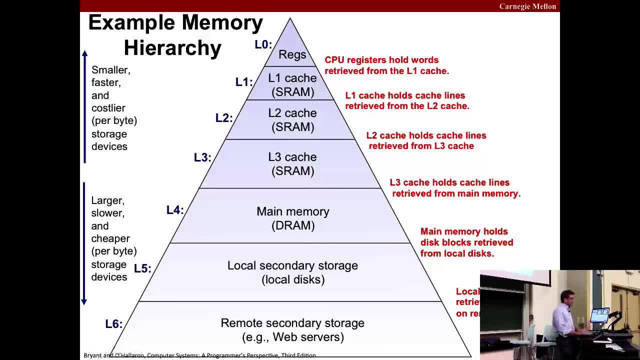 just part of our hierarchy. now here's the. here's the key idea in a higher, you know in a memory hierarchy, each level in this hierarchy holds data that's retrieved from the next lower level. Okay, so registers hold data that's stored in the L1 cache. 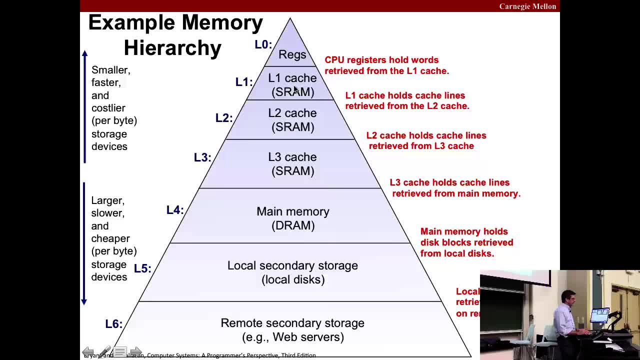 The L1 cache holds data that's retrieved from the L2 cache. The L3 cache holds data that's retrieved from main memory. Main memory holds data that's retrieved from secondary disk, and so on. Now, as we'll see the reason, memory systems are designed like this. 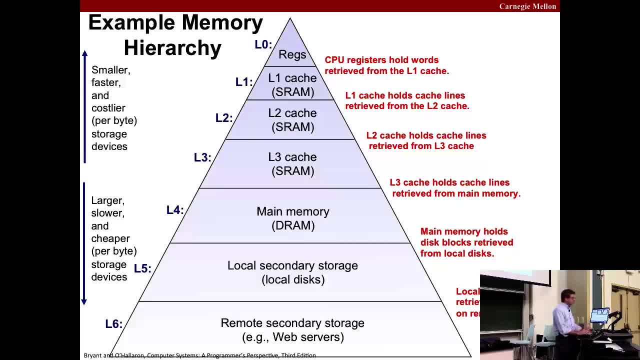 is that they, when you have this kind of system, this you can access. in general, you can access your data at the speed of the fastest item at the top of the hierarchy. So that's the fastest, But with the cost of the storage at the lower part of the hierarchy. 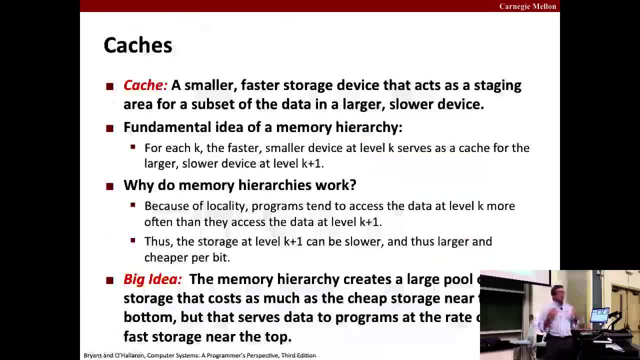 Okay, so this works all because of an idea called the L1 cache. It's called caching, So a cache. to a computer scientist it's a smaller, faster storage device that acts as a staging area for the data in a larger, slower device. 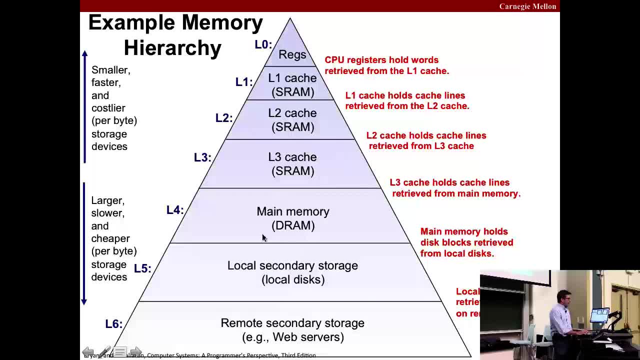 So, just like here, you can think of your main memory as a cache for data that's stored on disk. You read memory from disk and then you store it in main memory. Okay, you can think of the main memory as a staging area. 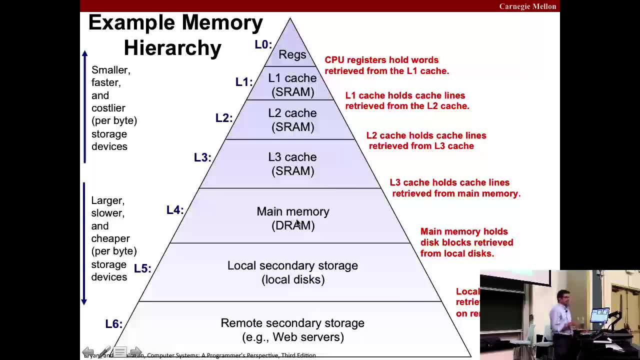 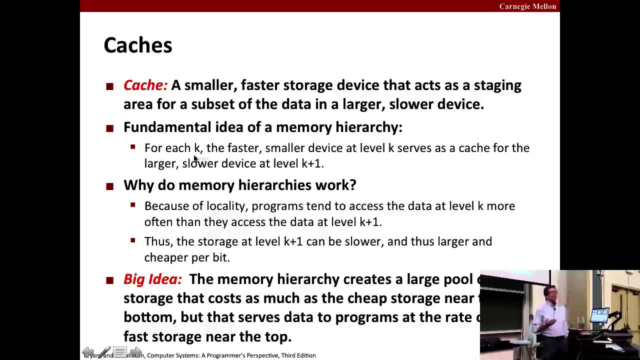 So once you get the data from the disk, you don't access it again on the disk, you access it in memory, which is much faster. Okay, so this idea propagates all the way up the hierarchy. Okay, so we you can think of a cache. 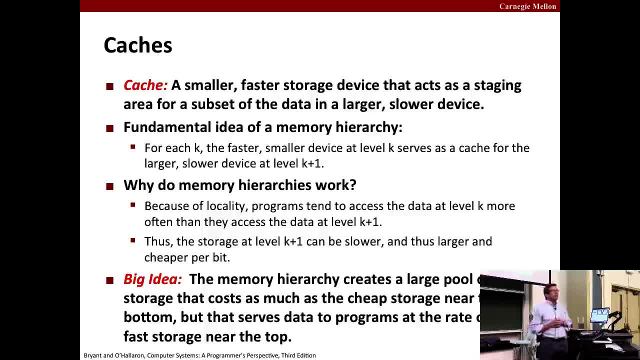 one way to think of a cache is: imagine your backpack when you're getting ready to come to school in the morning. So you're in your apartment, which is kind of far, far away from school. So before you come into school you take items from your house. 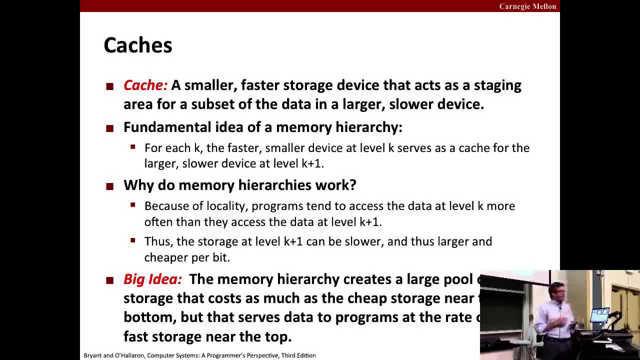 and you put them in your backpack- right, Because? and then you walk to, then you come to school and if you need those items they're in your backpack. You know, if you didn't do that every time you needed something. 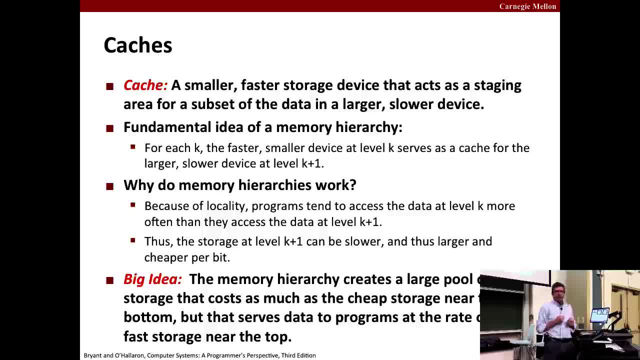 you'd have to walk back home and get it and then walk back to school. All right, so it's so. the idea of caching is very- you know, it's a very familiar kind of simple notion, but it turns out to be quite powerful. 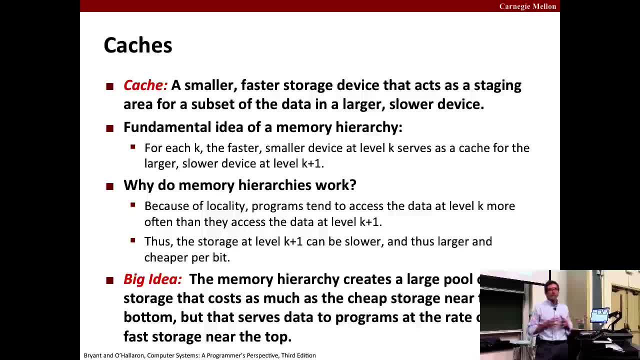 And it it shows up in all parts of of computer systems. Okay, so, so what we say is that for each level K in the hierarchy, the the faster smaller device at level K serves as a cache for the larger. 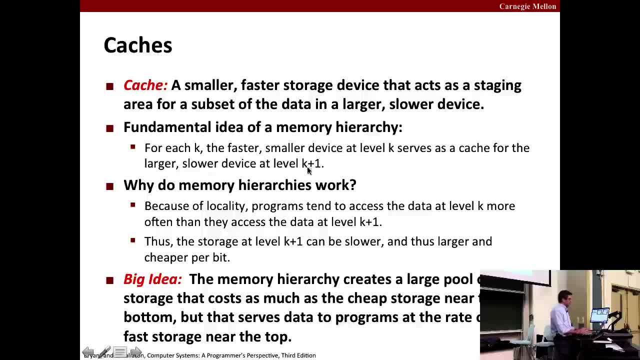 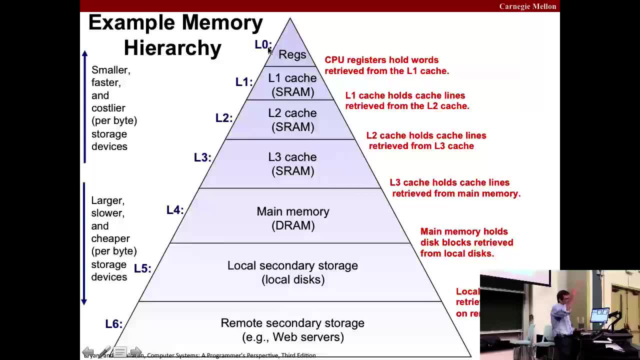 slower device at level K plus one. And remember our, our levels go from: so L zero is the highest. So the the smallest, lowest level is actually the highest, the furthest up in the in the hierarchy. Okay. 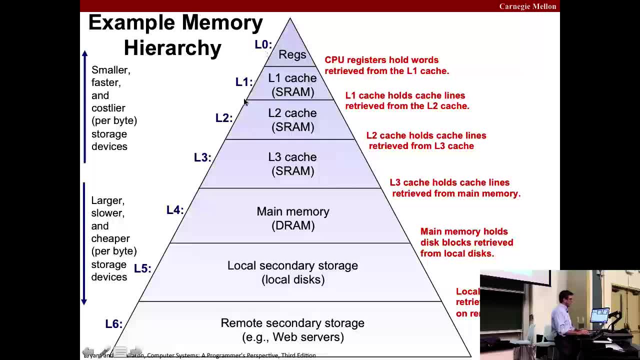 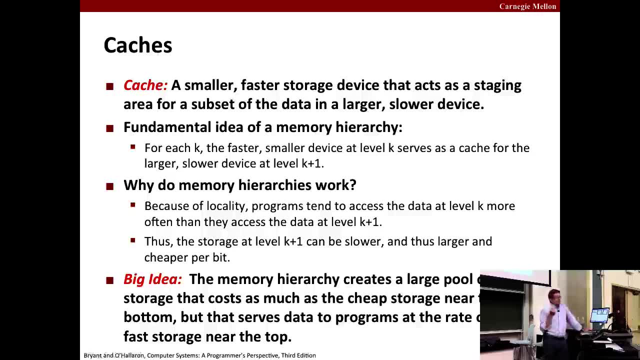 And as we increase the levels, we're going down the hierarchy. Now, why do they work? So this is this is a really fundamental idea: They work because of locality, So be because of locality. programs tend to access data that's stored at level K more often. 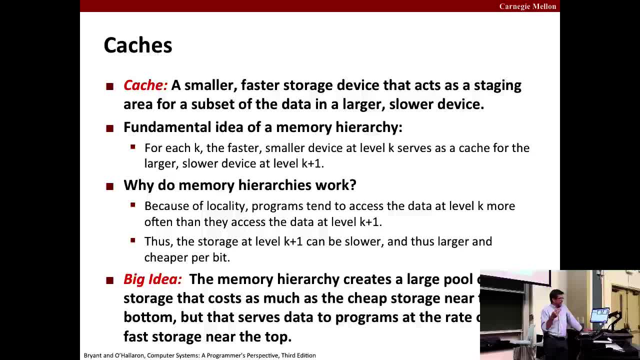 than they access data at level K plus one. Okay, so if we access an item at level K plus one, we can move it up to level K. chances are, because of locality, we're going to access it again. Okay, so now we're accessing the data at level K multiple times. 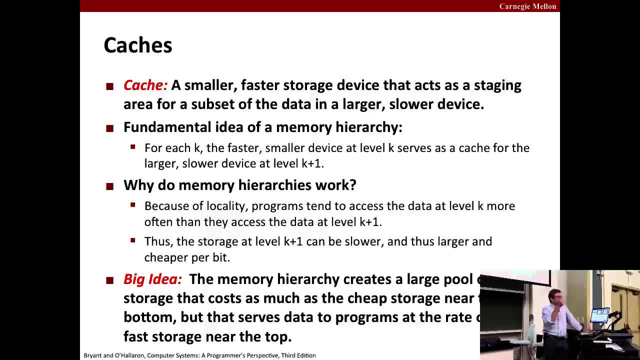 at the, at, at the rate, at the speed of level K, not at the speed of level K plus one. Okay, so that's, that's the fun, the, the fundamental idea. And because? because we're not accessing data at level K plus one, as often? 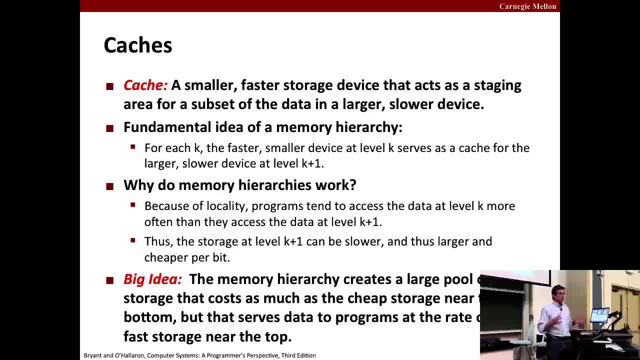 we can. we can afford to use slower storage devices, which are cheaper, Okay, And thus and thus we can make them bigger and cheaper per bit. So what this does is the hierarchy creates a, a large pool of storage. that's roughly about the size. 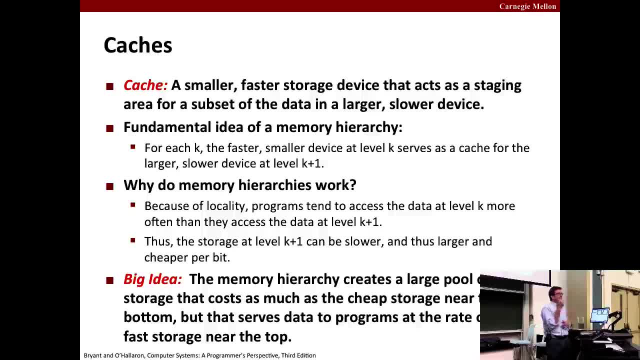 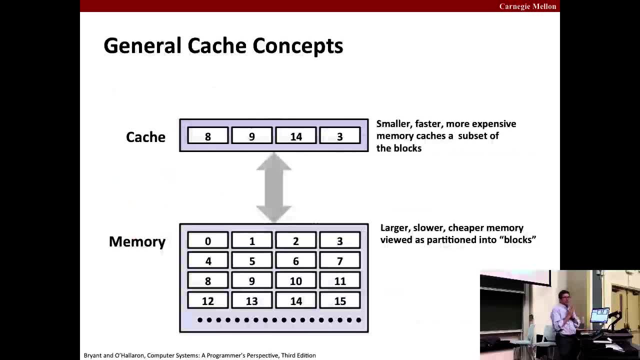 of the lowest level that can be accessed at the speed at at the highest level. Okay, All right, Let's do this again. Let's do this again. let's look at how caching works in a general way, and then we'll see on. 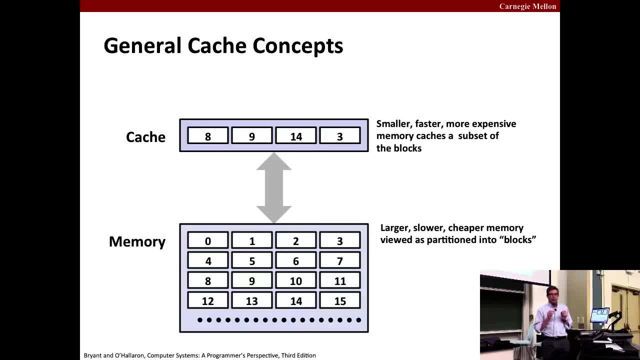 Thursday how these hardware cache memories work. okay, but, like I said, caching is a very general idea that can be applied at all levels in the in the hierarchy. so here we have a cache. so the in all kinds of most caches there's some kind of transfer unit to go from one level to the next. so here we have at. 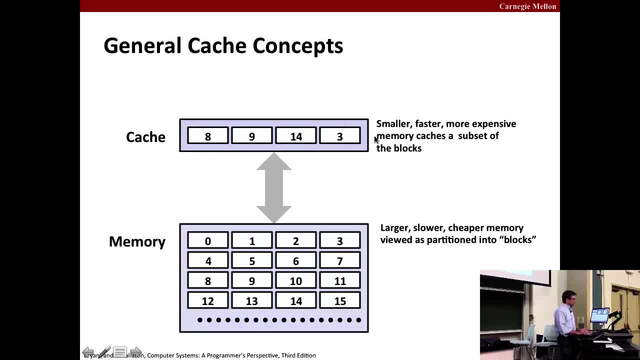 this. at this upper level, we have a, what we'll call the cache, that can hold four blocks, so our, our memory. and then at the lower level, we have memory, and this memory is partitioned into blocks of some fixed size. that's this. that's the way. cache is near the upper part of the hierarchy, work now at the lower levels. 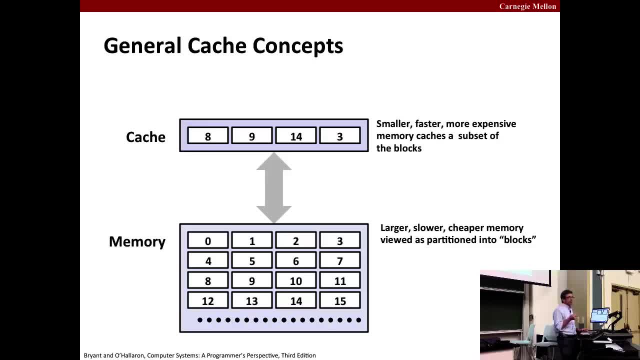 like, if you're accessing data, say, from a web server, then the the data is partitioned into files, typically okay, but at upper levels the data is partitioned into blocks. so just suppose this is main memory and then above that we have a that consists of a bunch of. 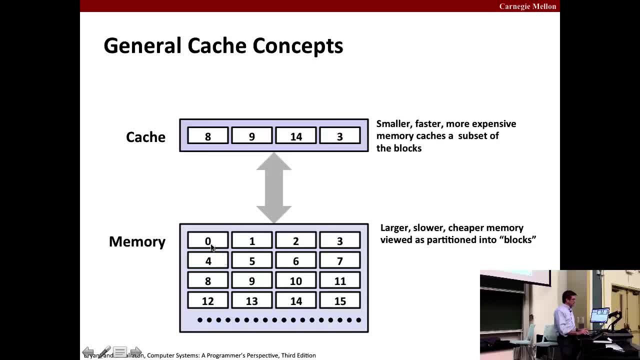 these blocks. so we just take the memory and partition into blocks where each block is the same number of bytes, and then data will be transferred between memory and the cache in block size transfer units. okay, so if you need data from the memory, if the cache needs data from the memory, it'll grab a whole block and then at any point, 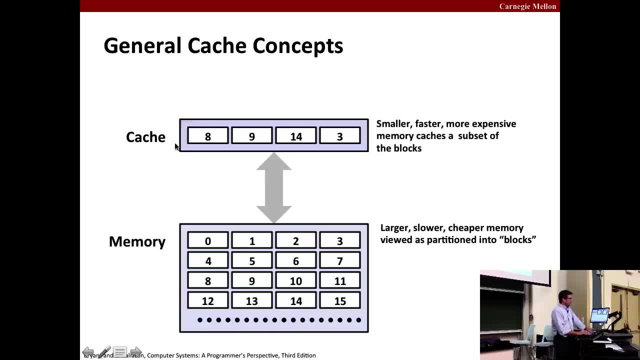 in time. the cache holds a subset of the, the blocks in main memory. okay, so this, this cache is much faster but it's also much slower and because of that, and it's much smaller. I'm sorry. it's much faster but it's 40 for the cache and it's much more expensive because it's faster, it's. 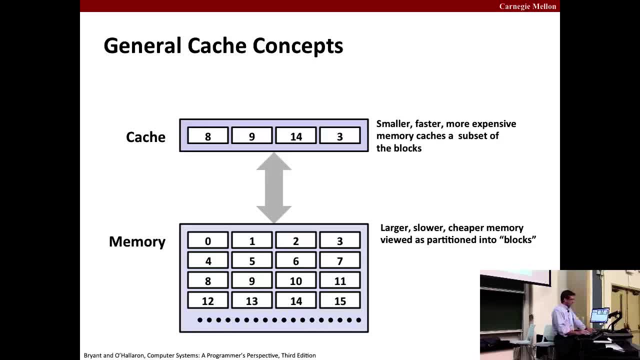 more expensive and because it's more expensive it's smaller. now suppose, suppose the cache wants to reference, say that the CPU asks for data that's contained in block 4, so it looks. it looks to see if the data is in the cache. it's not, so the cache asks the memory to. 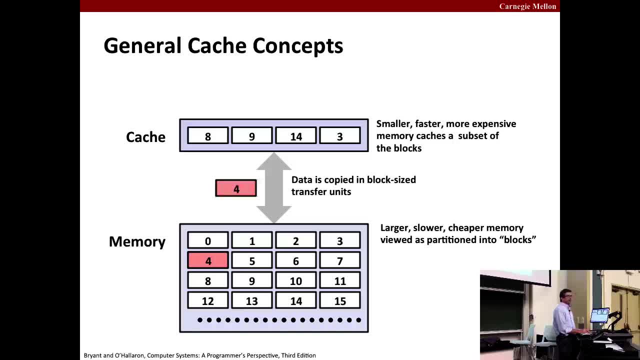 give it block four So that block is copied from memory into the cache, overriding the one of the existing, in this case block eight. it'll overwrite block eight. So now block four is in our cache. Now suppose the CPU asks for some data that's in block ten, that gets copied up and we 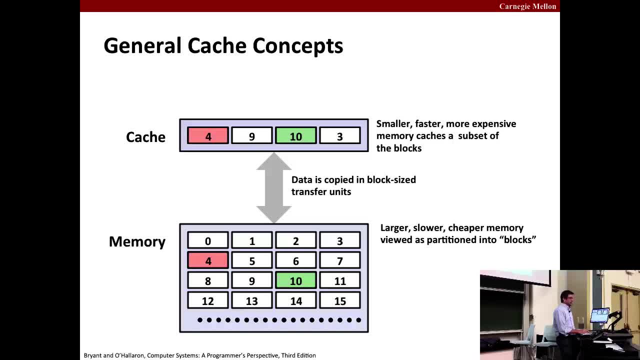 overwrite that block. Now the whole idea of storing it in the cache is that we're hoping that the program that's executing on the CPU will reuse one of those blocks. We just spent all the time we went to all this trouble to copy it from memory to this cache and we know that's slow. So now, 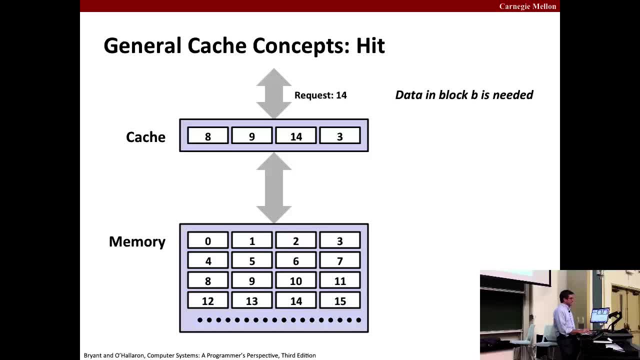 suppose that the CPU needs some data in block B in this case 14.. So now suppose that the CPU needs some data in block B in this case 14.. So now suppose that the CPU needs some data in block B in this case 14.. 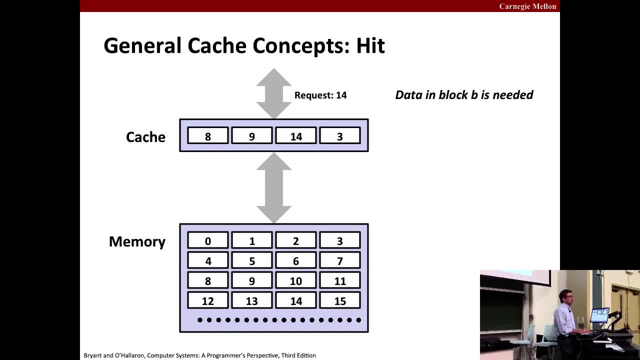 So it needs a memory word that was originally stored in memory in block 14.. Well, now this cache can just return. that's what we call a hit right. So the block that we access is in the cache. so that's good. hits are good, Because now we 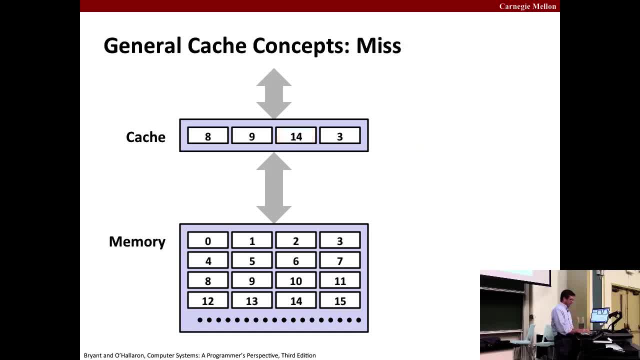 can return that block directly to the CPU and this memory is much faster than if we had to go all the way to main memory, to the DRAM. Okay, so the SRAM much faster than the DRAM. so the CPU gets that block 14 much faster than it would have if it had just gone. 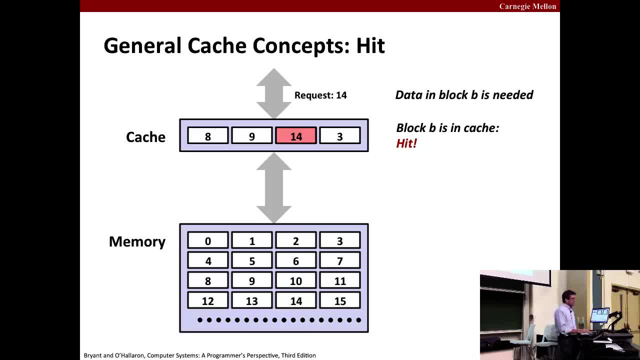 all the way to memory. Okay, the sort of other. the opposite of a hit is a miss. So suppose the CPU asks for block 12, the cache looks for that block. can't find it. that's a miss, So the cache has to. 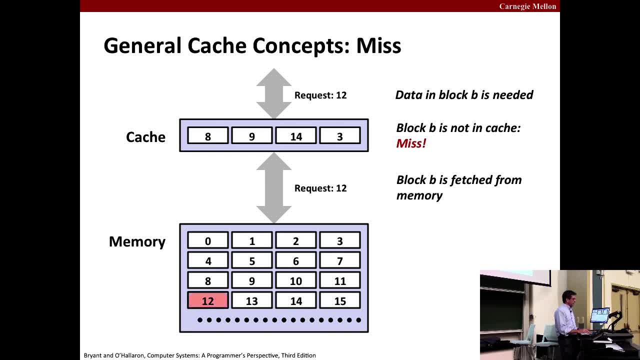 ask that the main memory of the DRAM for block 12, where it gets copied into the cache and then it can return that. So that takes longer, right? So the CPU has to wait for that block to be to be fetched from memory and so misses are. 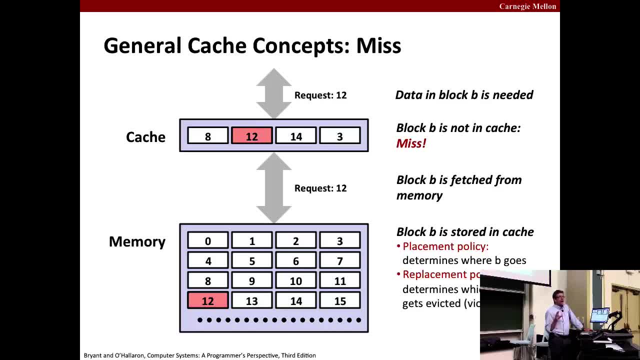 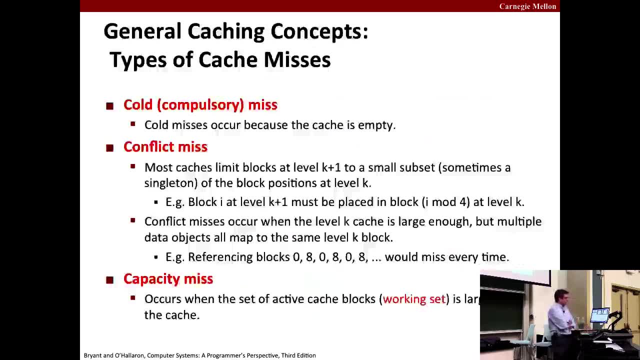 slow. So hits are good because they're fast, misses are bad because they're they're slow. Now we typically distinguish between several different kinds of caches. So the first kind of miss is a cold miss or a compulsory miss, which is caused because 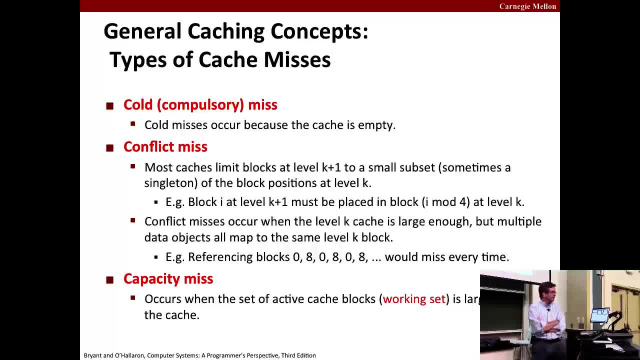 there's just nothing in the cache. right Initially, caches are empty. they have no blocks and as we fetch, as we fetch blocks from the lower level, from the next, the next level and put them in the cache, the cache will slowly fill up with. 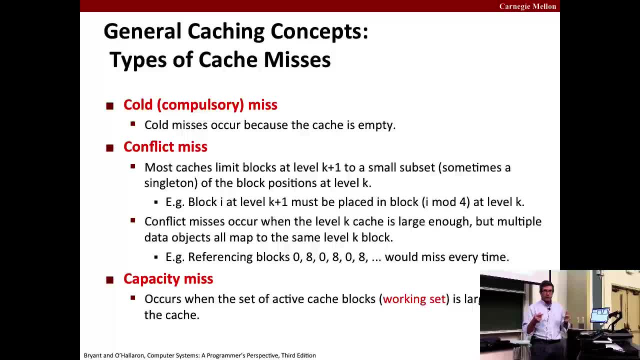 blocks and we'll get, and that'll increase the likelihood of hits. But when the cache is empty, we're going to miss every time, right? So there's, there's just no way to avoid cold misses. right, You got to. 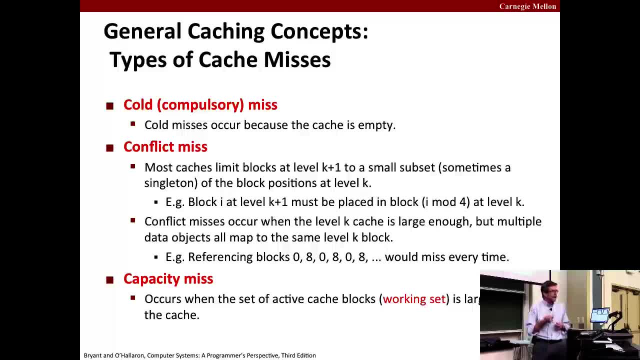 this is called warming up your cache. So as you load data items into the cache, initially it's cold, and as you add more items, you're warming it up, meaning that you're increasing the likelihood of a hit. Now there's a. there's another sort. 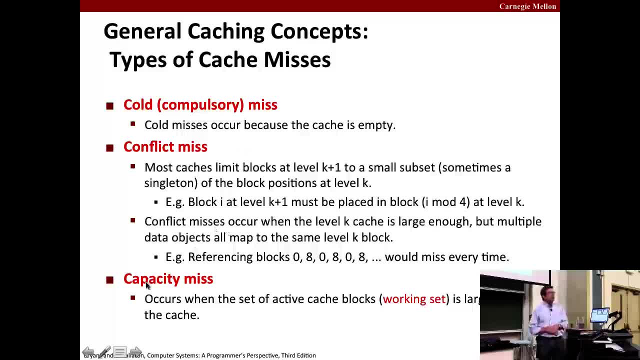 of symmetric kind of miss, which is called a capacity miss, and these misses are due to the fact that the cache is just a certain size, right, You just can't. in the example we looked at, we only had four blocks. So if we're, if we're trying, if our, if our, if our temporal, 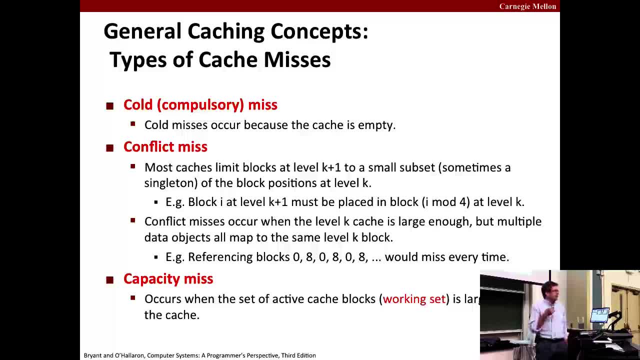 locality involves eight blocks. you know, say, if the loop that we're accessing is is accessing elements in array, that that consists of eight blocks. there's just not enough room to store eight blocks and have four block cache. so we're going to 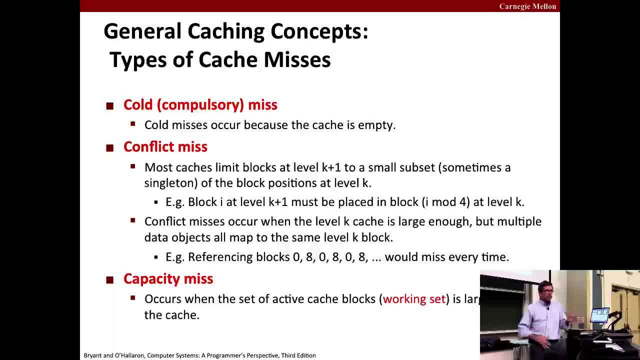 get misses right. We would need a bigger cache to be able to satisfy and store those eight blocks. And if we had a big enough cache then we get good hit rate right. If we could store all the blocks in our cache then we then the cache could. 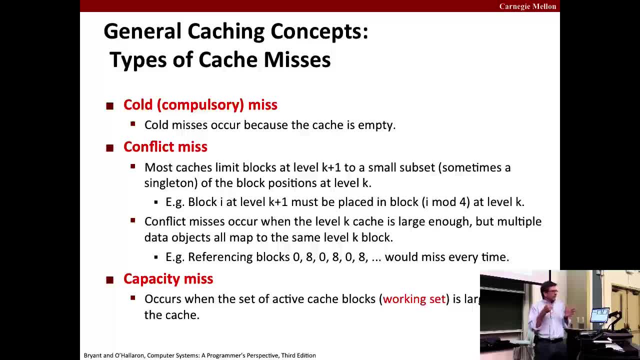 take advantage of the spatial and temporal locality within that program. So, in general, what we call this set of blocks at any point in time when a program is running, we call the set of blocks that are sort of being accessed over and over again, the working set. And so your working set and the working set, if you let, if you made six regular blocks. 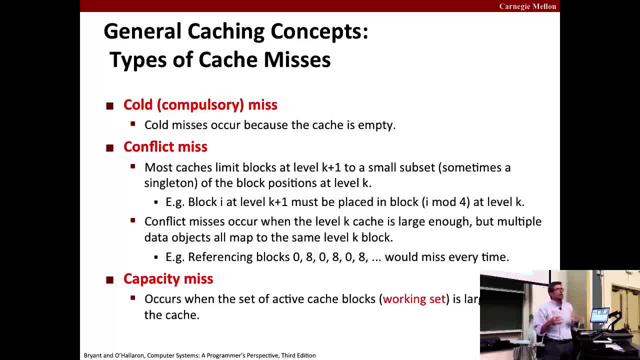 working set, and so your working set and the set will change, you know, as you go from loop to loop or from function to function. but at any point in time in your program when it, you have this idea of a working set which is sort of the 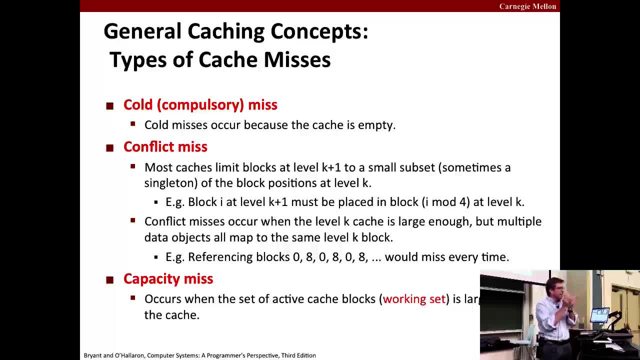 blocks that you need to have stored in your cache. okay, the same way. so when you're working, set size exceeds your cache size, then you get capacity misses. there's this other kind of weird miss called the conflict miss, which has to do with the way that caches are often implemented. so the idea 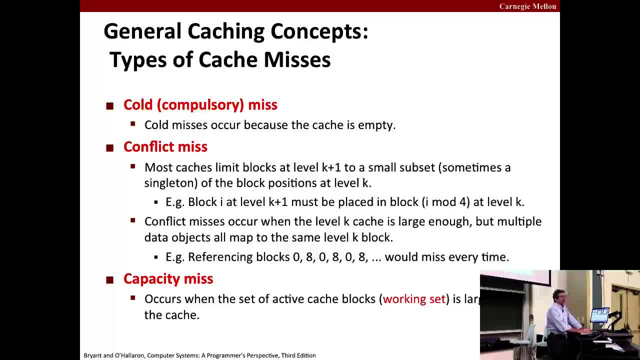 is that most caches, especially hardware caches, because they're they have to be simple, they have they limit where a block can be placed to some small set of positions in the cache. so, like one of the, the simplest models is to just take block I can only be placed in block. I mod the cache size. so in our that that little cache we saw, 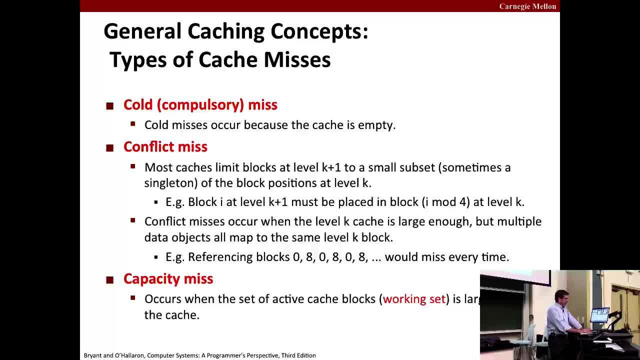 that had four blocks we would take. we would take block I for memory and we would stick it at block I, mod 4, so block 0 would go at block 0 in our cache, as would block 4 and as would block 8, block 9. 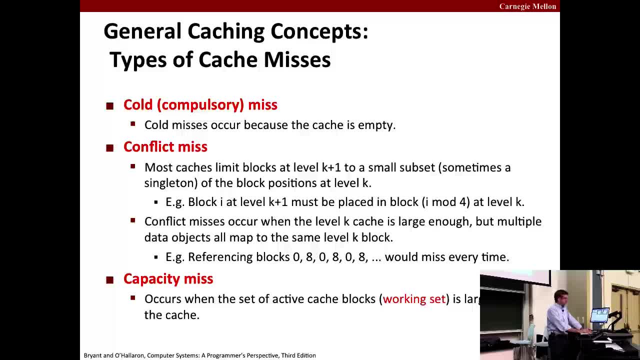 would go into block 1 in the cache, and that's when that happens. suppose, suppose we use that model. so we're going to take block I and we're going to put it. we can only place it in the cache at block I, mod 4. now suppose our, suppose our. 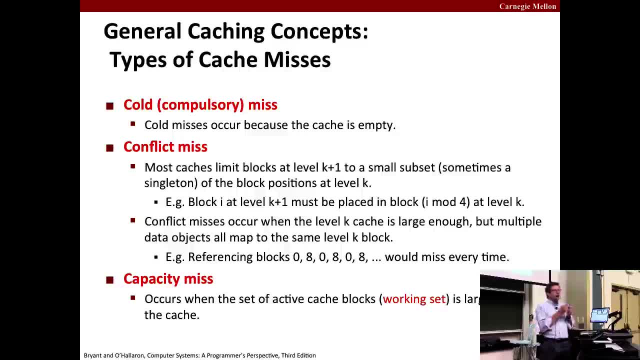 reference pattern involves, from memory, block 0, block 4 and block 8. it's only three blocks. so we have we have enough room in the cache to store those three blocks but because of the way we've decided to place blocks, each block will be will evict. when we access block 4, it'll go into block. 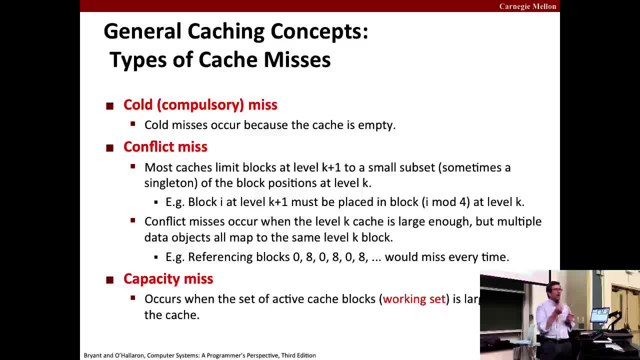 0 in the cache. when we access block 4 in the cache, it'll overwrite that block and it'll go into block 0 in the cache, and so, because of this, it's really the, the access pattern, conspiring with the, the algorithm that we're using for placing blocks. okay, so because of this, we have 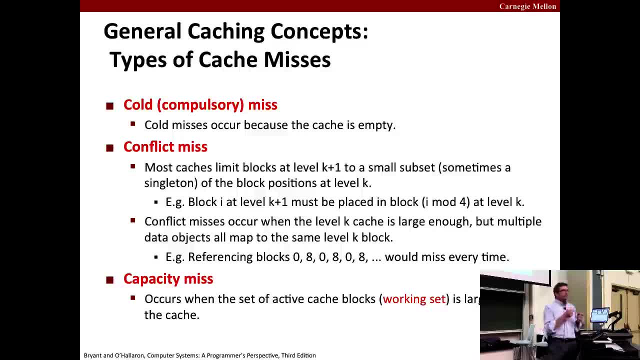 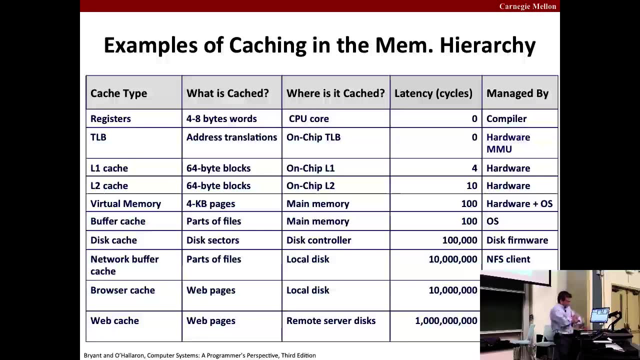 plenty of room in the cache, but because of this sort of the- the access pattern conspiring with the placement algorithm, we get misses every time. okay, we'll see how conflict. we'll see how conflict nurses work in detail when we study cassius tomorrow. so so this is the 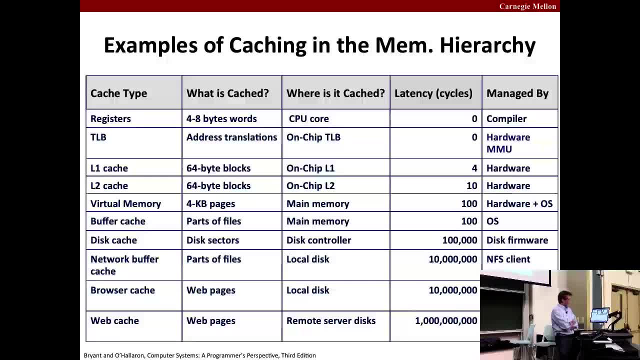 These caches exist everywhere in the memory hierarchy, And so all of them are caches of one form or another. So you can think of the registers as a type of cache. What are they cached? Four or eight byte words. Where is it cached? 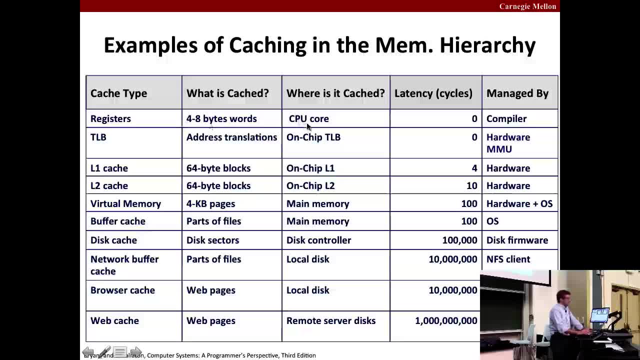 It's cached right on the CPU itself. What's the latency? It's instant. It happens within an instruction. And then who manages the cache? Somebody has to manage the cache When there's a request to load an item from the lower level in the hierarchy something. 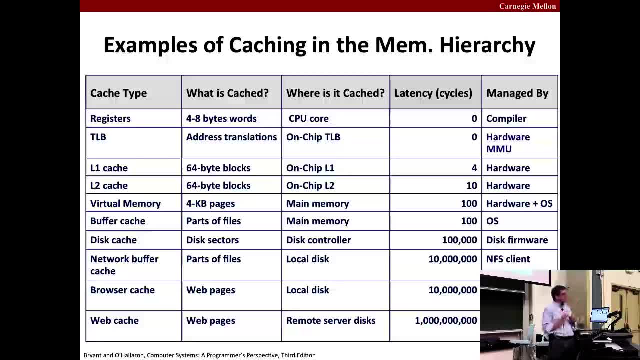 has to decide what to do with that, where to put it in the cache. That's called managing the cache. Well, in this case the compiler manages the cache. When you compile your C code, the compiler figures out which register data items from memory. 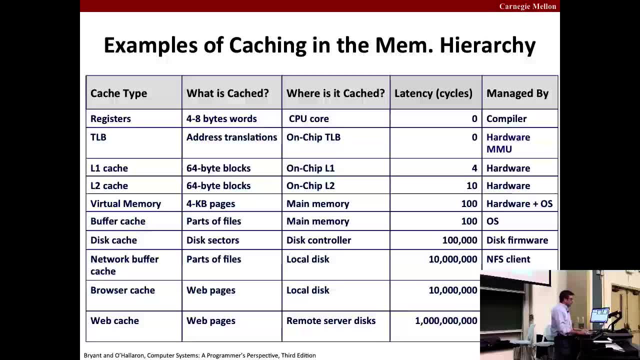 are going to go into. So TLB, this is something. This is a cache that's used. It's used in virtual memory. Then there's these hardware caches called L1 and L2 caches, So they store 64-byte blocks on modern Intel systems. 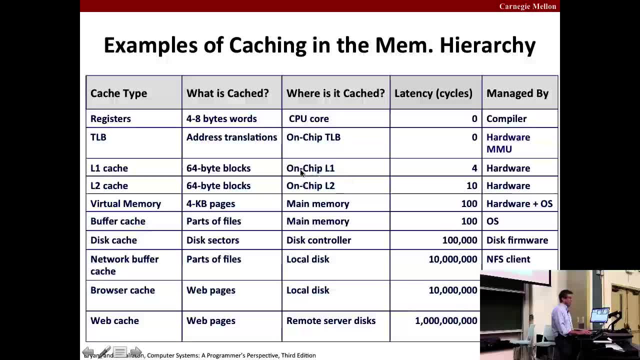 And they're cached on the CPU chip itself, in SRAMs that are built right into the CPU chip And, depending on whether L1 caches on Core i7s have a latency of four cycles and L2 has a latency of 10 cycles. 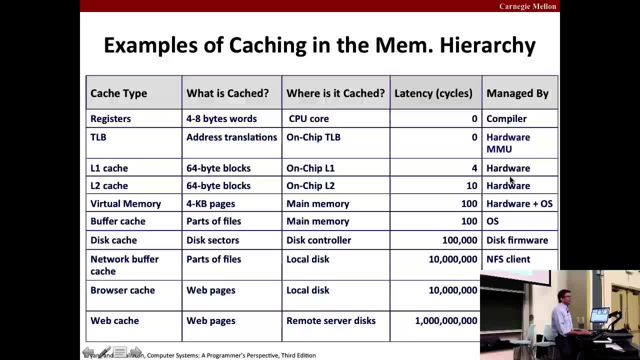 And both of these are managed by hardware. So when the CPU fetches an item from the L1 cache, hardware finds it, And if there's a miss and a block is loaded from L2, hardware in the L1 cache figures out where to put it. 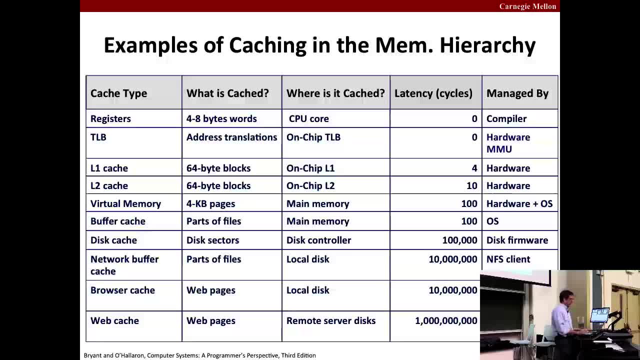 So all this is done without any intervention by hardware. Operating systems maintain buffer caches, So in this case what's cached is portions of files, and they're cached in main memory, And latency to main memory is about 100 cycles or so. 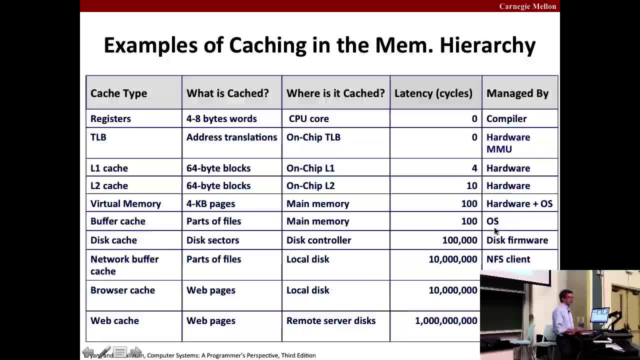 And these are managed by the operating system. So the operating system reserves a portion of memory to store files that you've loaded. So the operating system exploits locality. If you read a file and then start referencing bytes from that file, it'll actually be served from the file cache. 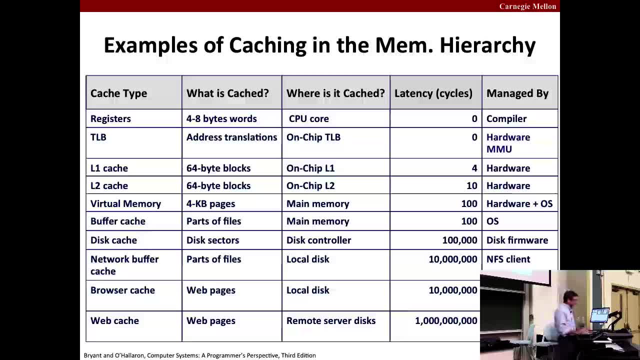 and it won't go out to disk. Networks maintain caches. Things like NFS and AFS maintain local caches on disk. Your browser has a cache, So when it fetches files from servers it stores those files locally on disk. So if you reference those web pages again,